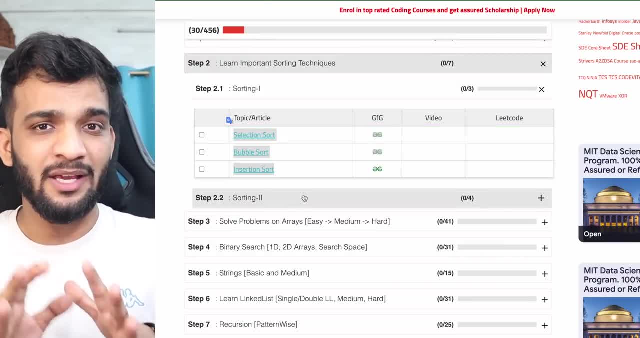 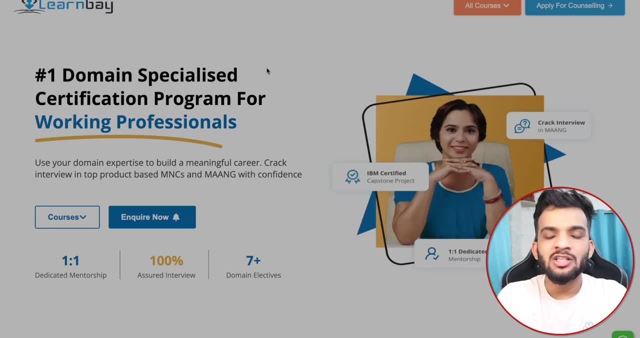 And you have to tell them right. And sorting two will be based on recursion, So we'll be covering that in the next lecture. So, without waiting, let's start with selection sort. So before moving ahead in the video, let me tell you about LearnBay. 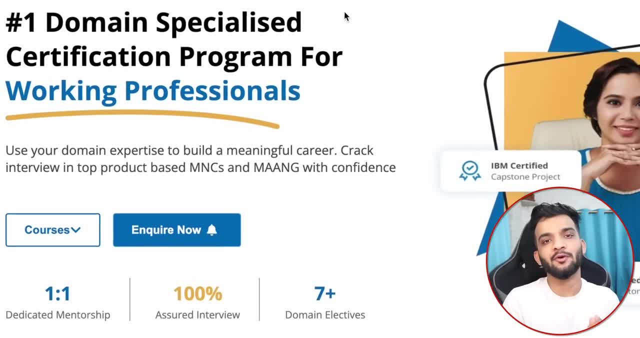 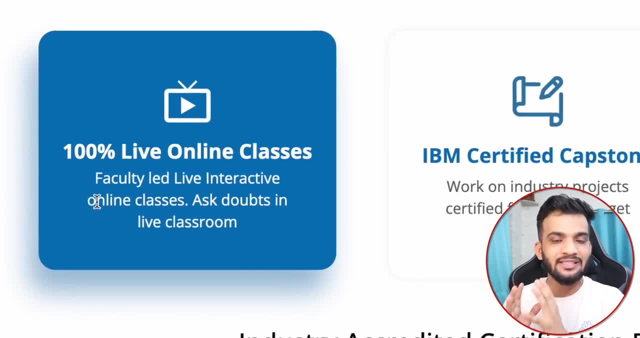 So LearnBay is an edtech platform that offers you data science and full stack development programs dedicated to professionals only. So at LearnBay, you will be getting 100% live online classes where you can interact with the faculties directly and get your doubt resolved. one is to one. 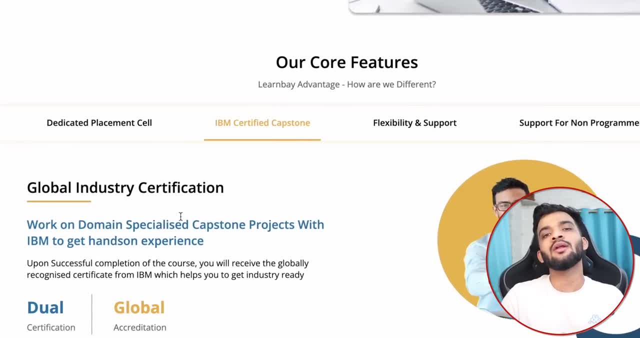 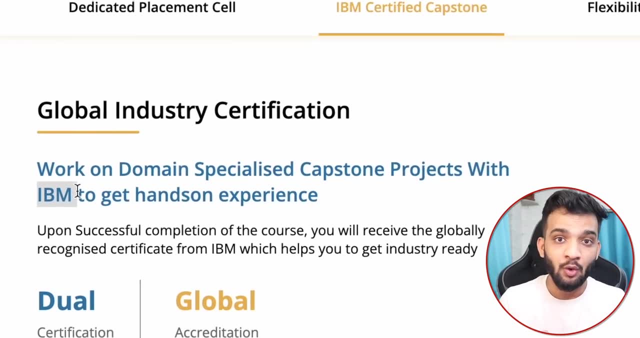 One thing I did like about LearnBay is you'll be getting an opportunity to work on industry-based capstone projects which will be certified by IBM. So you're going to get a global accreditation which will be beneficial whenever you present that project anywhere. 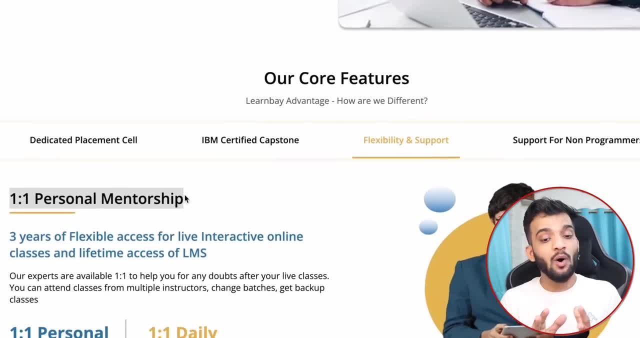 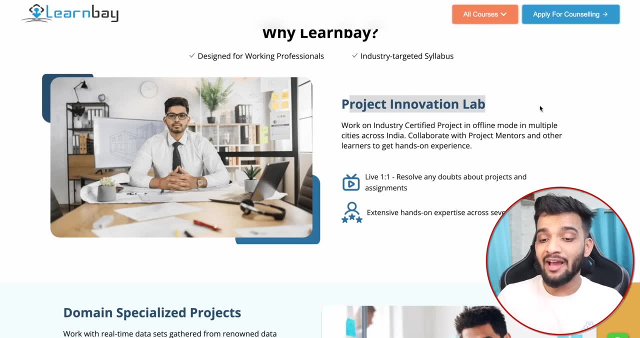 That's going to be very, very helpful. You also get in one is to one personal mentorship and you also get a one is to one daily doubt session where you can actually get all your doubts resolved. Also, they have project innovation labs across the country in Kolkata. 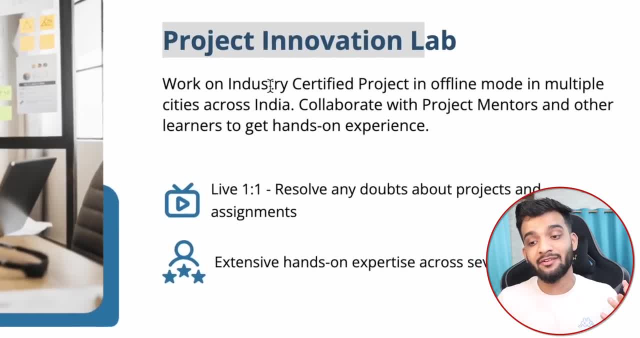 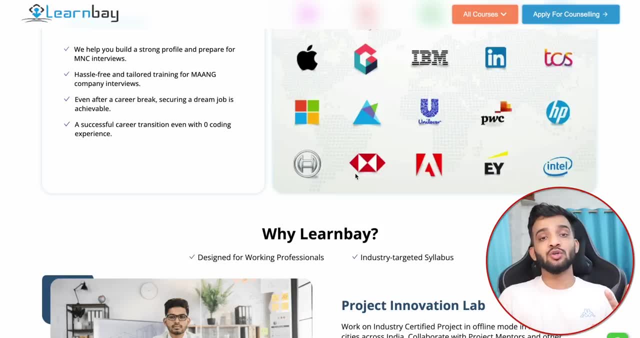 Pune, Bangalore, Hyderabad and a lot of other places, So you can go over there and create your projects in the offline mode as well. Once you enroll for any of the courses, you have three years of subscription, So you can have all the learning modules and all the videos for three years. 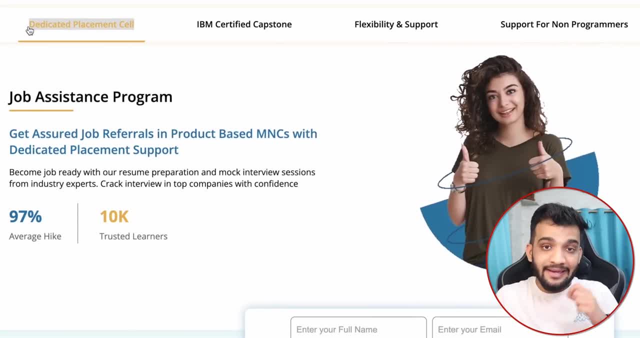 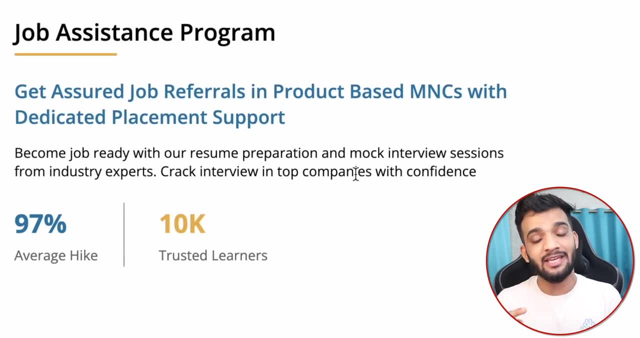 In this program you'll also be getting 100% job assistance by their dedicated placement cell And in the past people have got hikes up to 250% and they have partnered with more than 250 companies like EY, Intel, SAP and a lot others. 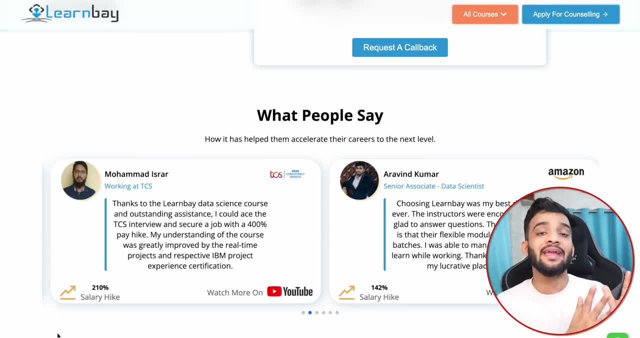 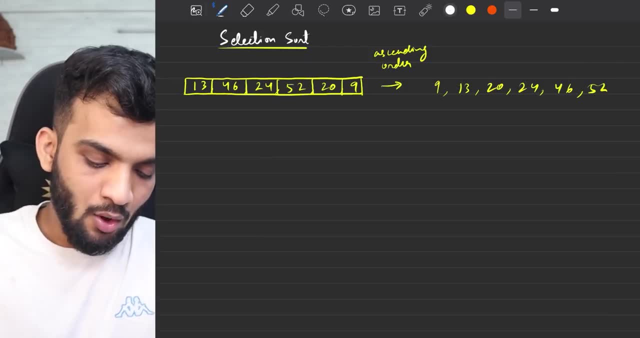 LearnBase nominees have also got placed in top companies like Amazon, TCL, Capgemini, etc. So what are you waiting for? There's a link in the description- Click it and get your free. one is to one career counseling session. The question: what is selection sort? 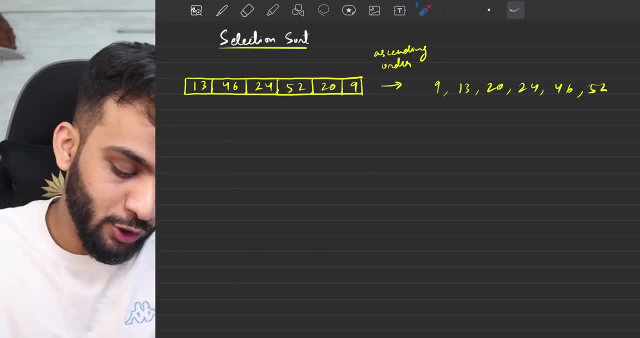 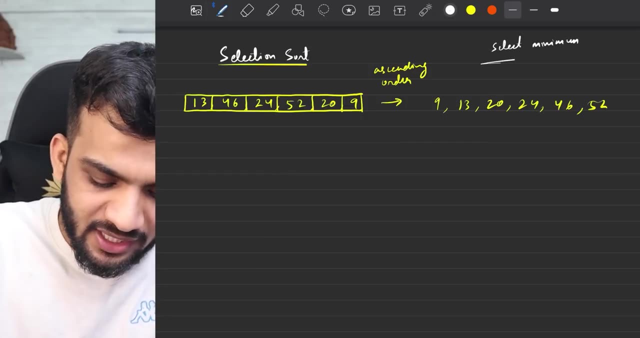 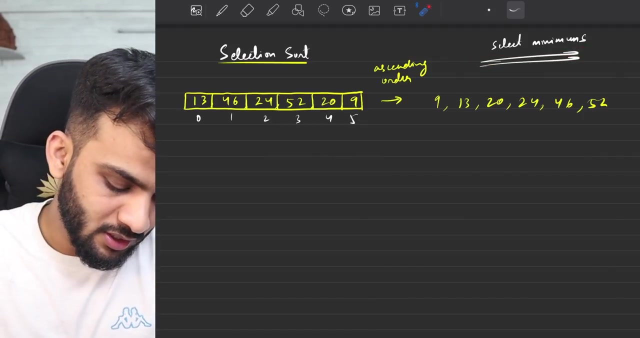 Does the name recommends selection. What do you select? We select minimums. Remember this. as the name recommends, what do you select? We select minimums. So, as the name recommends, select minimums. So what you will do is you'll look at the entire array and you will say who is the minimum. 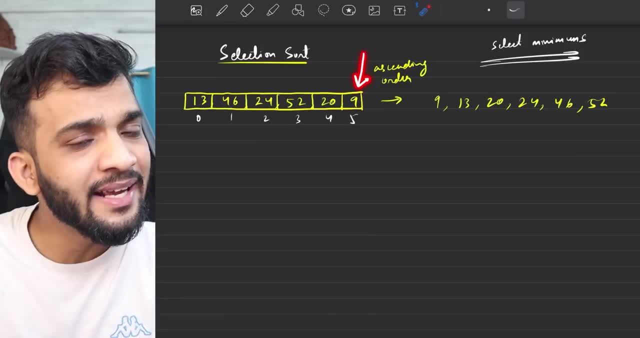 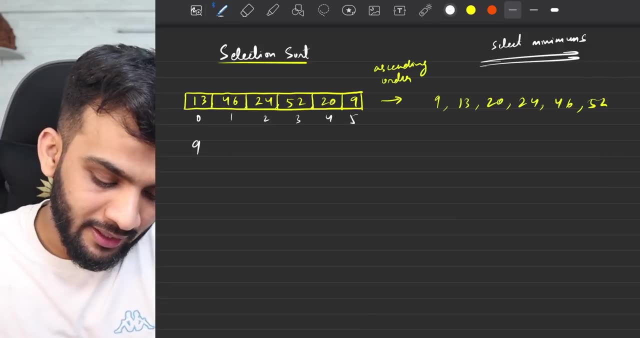 And it states 9 is the minimum. So you'll take that 9 and you'll place it here. Perfect, I place the 9 here. And if this 9 is the minimum and you're placing it at the first place, where will 13 go? 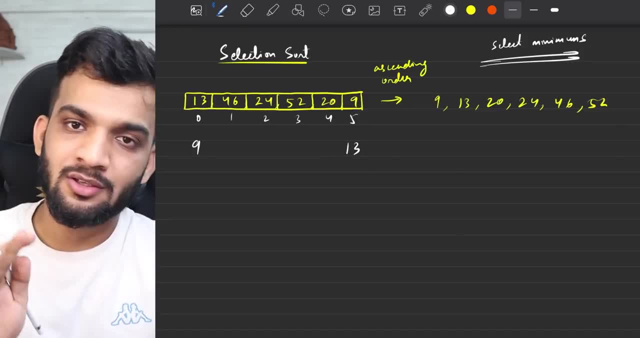 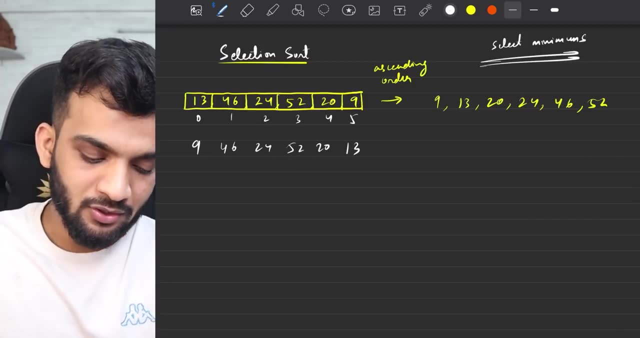 13 says: okay, no issues, I will go to your place because 9 has to come at first, And now I'll write the remaining guys over here. That's how you do it. So that is the step one of the algorithm. 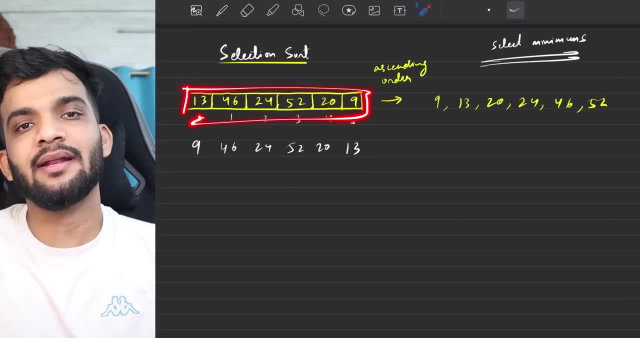 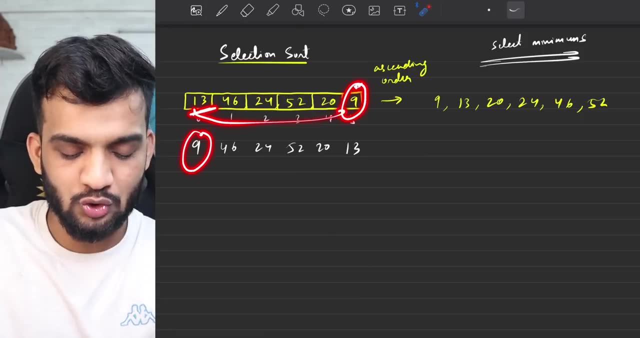 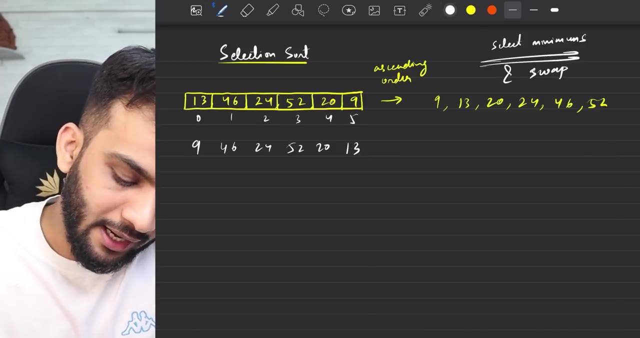 Step one states: get the minimum from the entire And you've got the minimum. They place it at the first. Whoever is at the first goes to that minimum. Simple as that. So swapping- select minimums and swap- Is what the algorithm is all about. 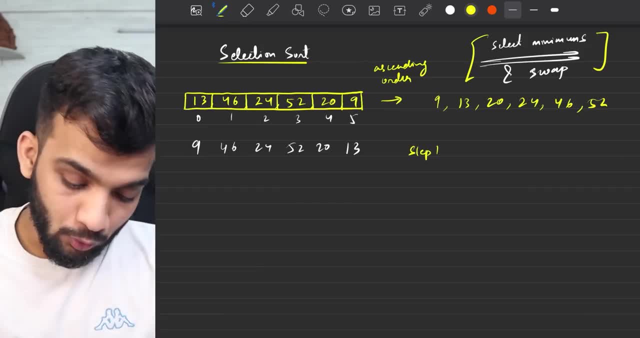 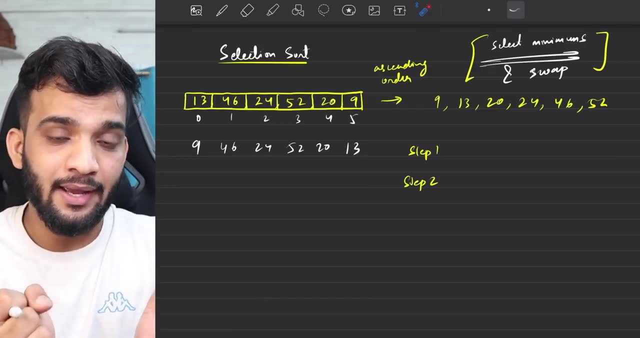 This is step one. Remember this. this is step one. What is step two? Let's see. So the step two states: okay, I know the first, I know, the extreme smallest guy is at the first. Now we should select the next minimum. 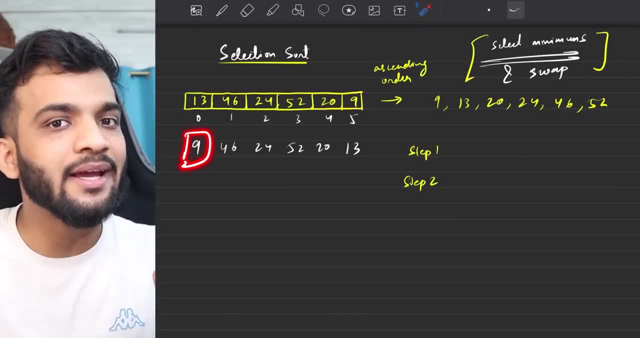 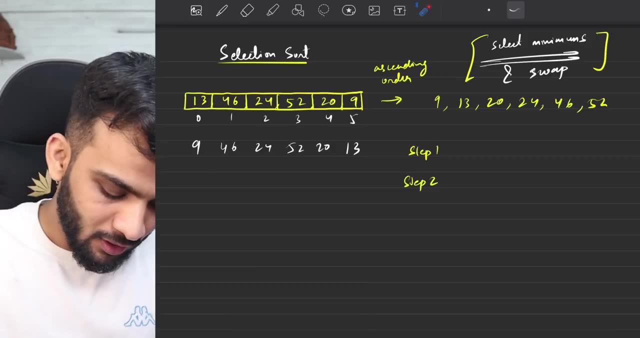 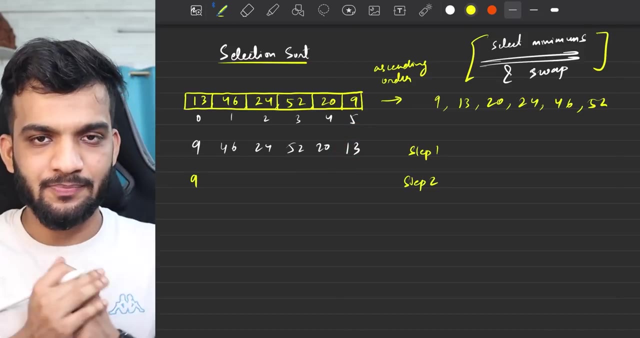 We know one thing: If the minimum is over here, this array is sorted. Which portion of the array is not sorted? That is this: Let's find the minimum. Can I say in this: 13 is the minimum. If 13 is the minimum, I know nine will stay where nine is. 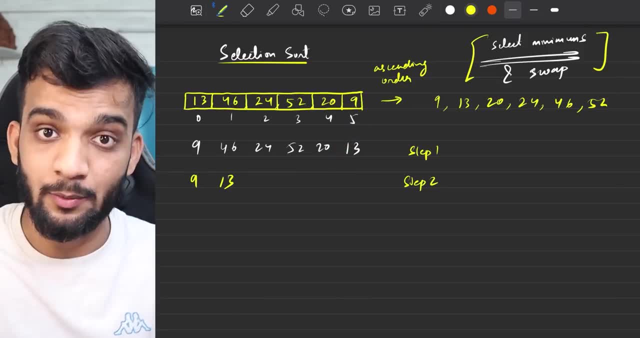 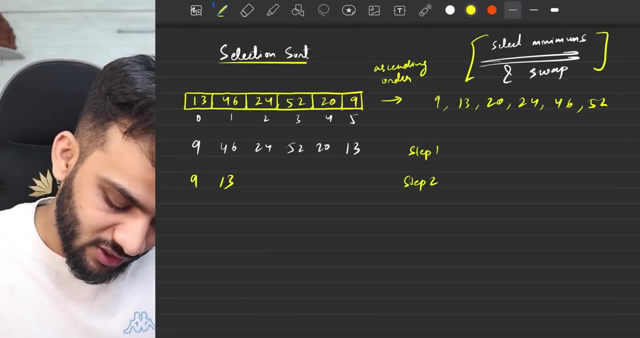 If 13 is the minimum, 13 will come at the first place. It will, And if 13 comes here, where will 46 go? 46 will go to 13. So 46 goes here and the rest remains as it is. 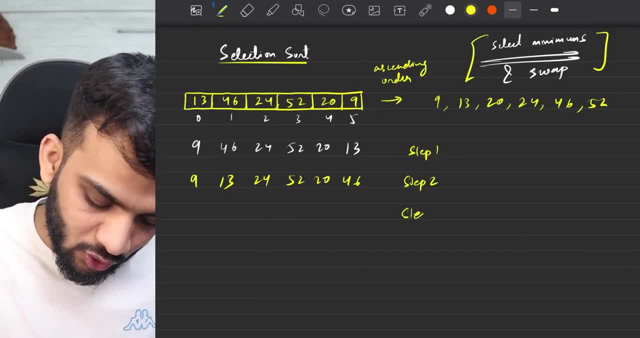 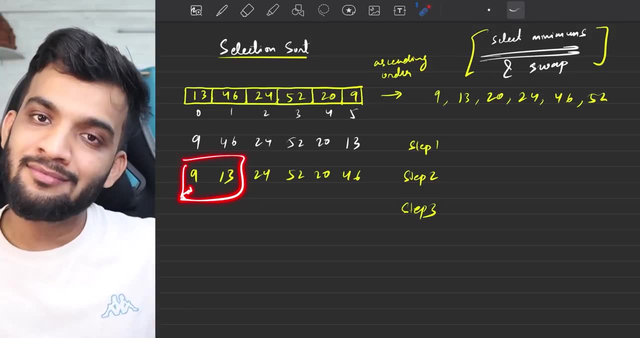 Perfect, Step two done, Let's do step three. So can I say, after two steps, I got the first, First two minimums, and this portion of the array is sorted I can. Now we are left with this portion: What to do. 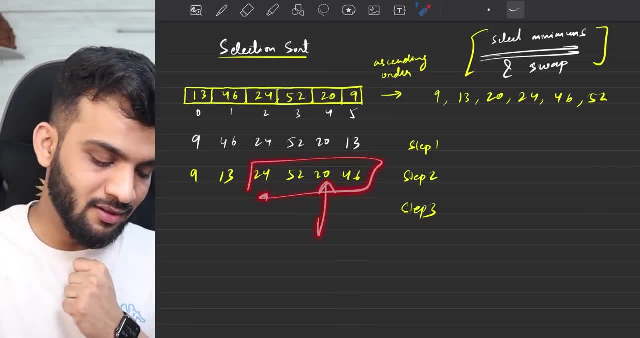 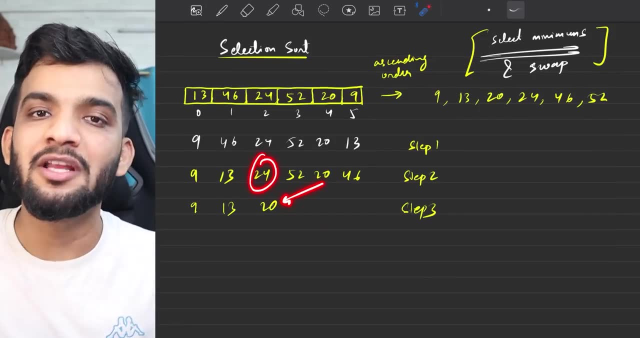 Get the next minimum. Who's the next minimum? 20.. As usual, 930 stays, 20 comes in. If 20 is coming in here, where will 24 go? 24 will go to 20.. So take it to there and 50 to 46 stays. 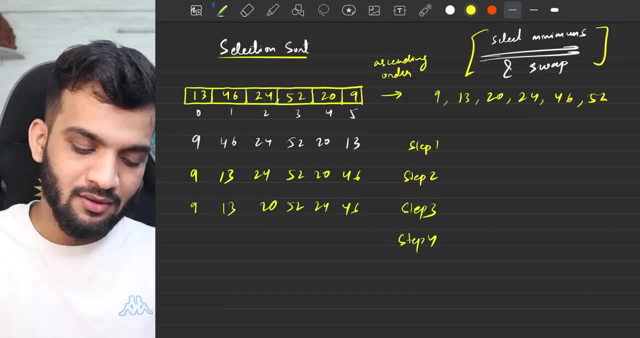 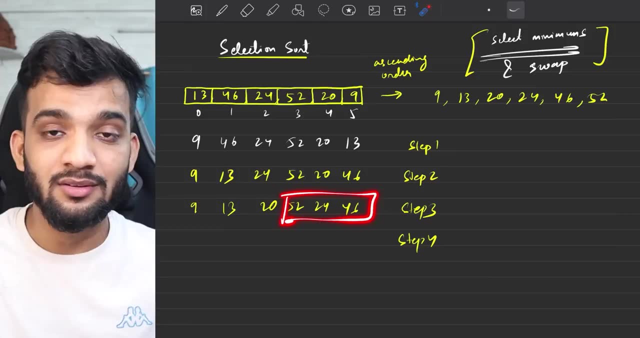 Step three is completed, Let's do step four At step four. can you say that this portion of the array is sorted? You can. Which portion is not This one? So in this, which is the minimum, 24.. Place it. 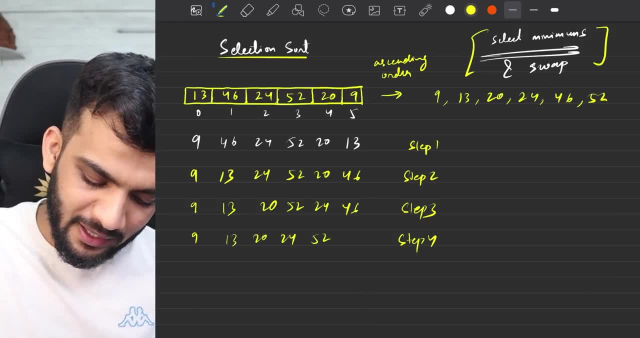 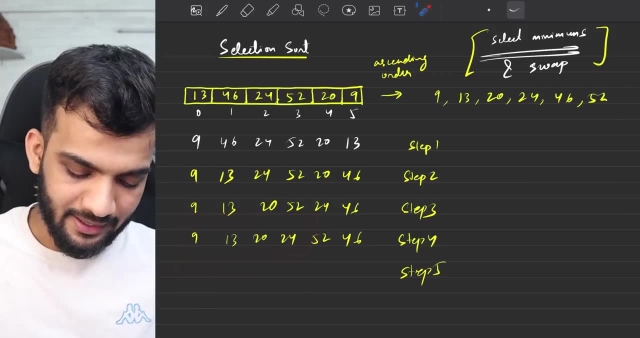 9,, 13,, 20,, 24,. 52 goes at its place 46. Let's do the step five. So can I say at step four, this is sorted and this is unsorted. Who's the minimum? 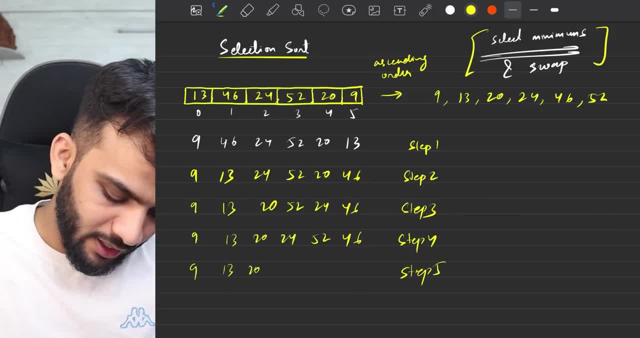 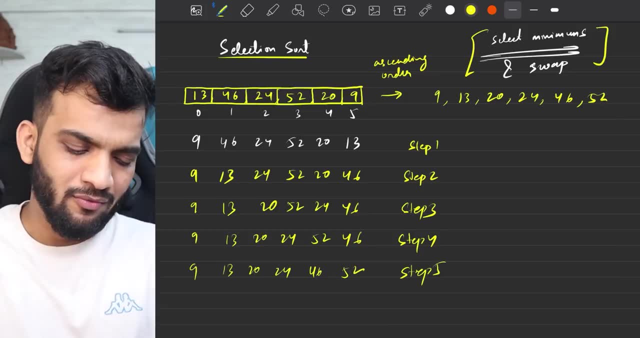 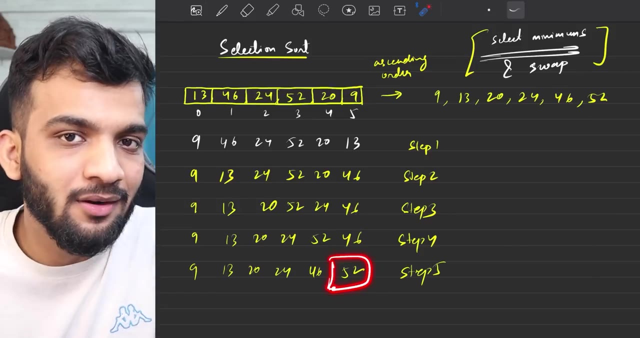 46.. So 9,, 13,, 20,, 26.. 20,, 24,- sorry, 46 will come here and 52 will go here. Now, at step five. if this is done, do you need to look like? do you need to sort one element? 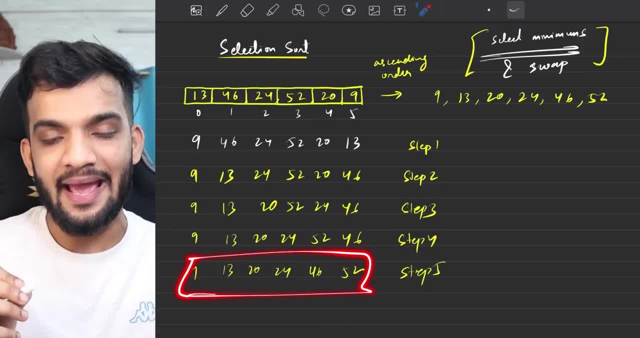 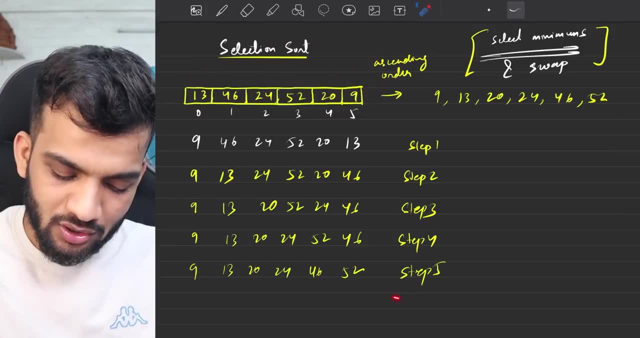 One element will always be sorted. So apparently can I say the entire array is sorted at step five: One, two, three, four, five, six, six elements, but actually took five steps to sort the entire array. What I did. 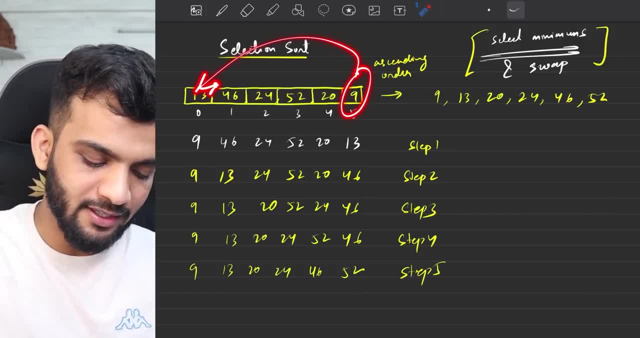 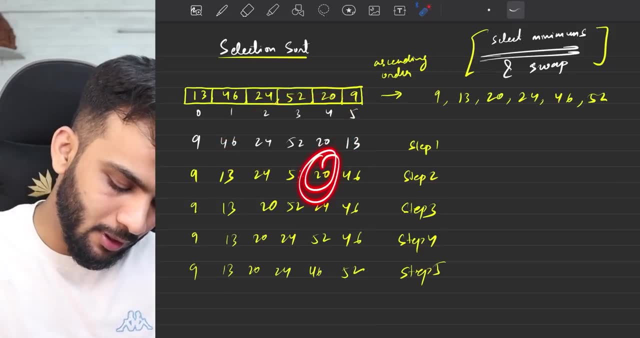 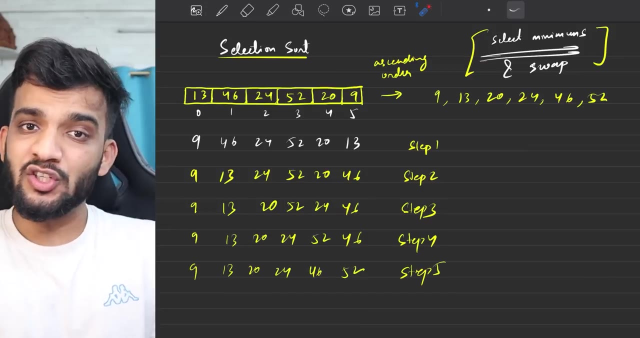 Was get the minimum and swap it and swap it. Then what I did was get the minimum and swap it. Then what I did was get the minimum and swap it. So get the minimum and swap is the algorithm. Now the question comes: okay, we've understood the algorithm, but how do I implement this in code? 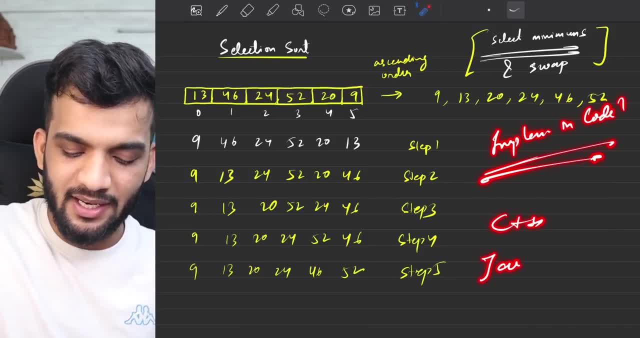 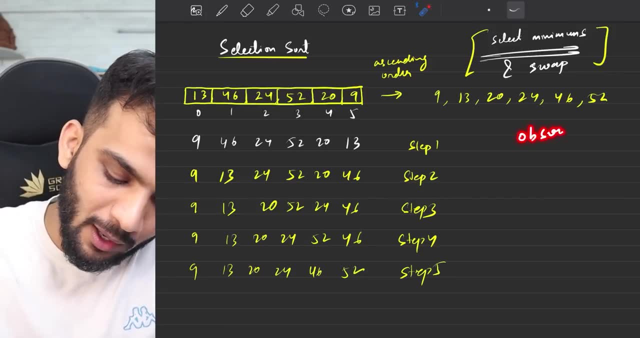 I'll be writing the pseudo code so that you can write it in C++ as well as in Java as well as in Python. So, in order to implement algorithms, you have to have something like observing power. Let's start observing. What's the first observation? 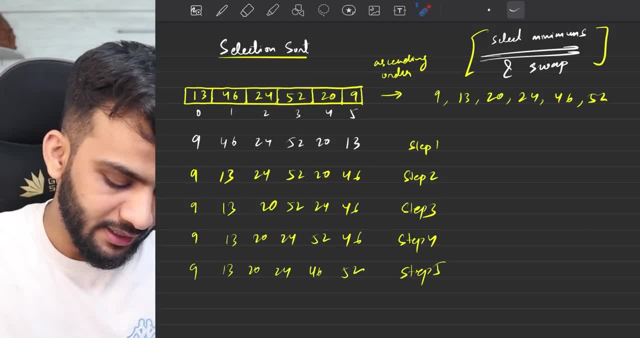 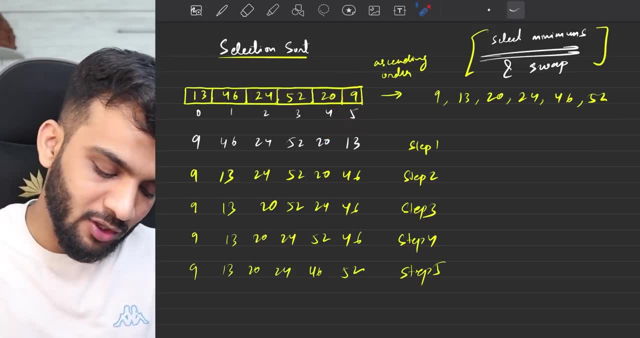 In the entire array, very, very simple. In the entire array you figured out the minimum. Can I say: you figured out the minimum And whichever index the minimum appeared, whichever index the minimum appeared, I swapped it with the first guy, zeroth index. 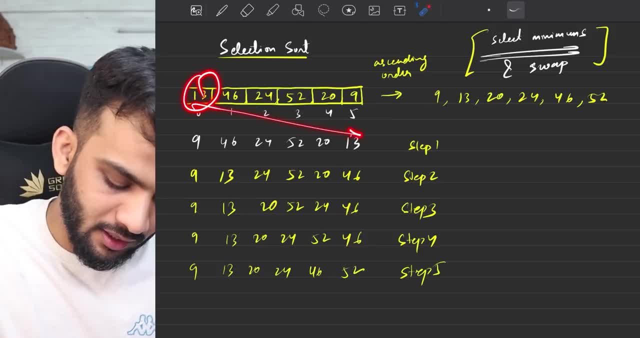 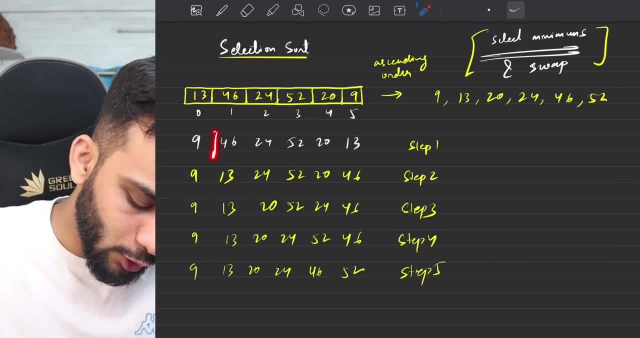 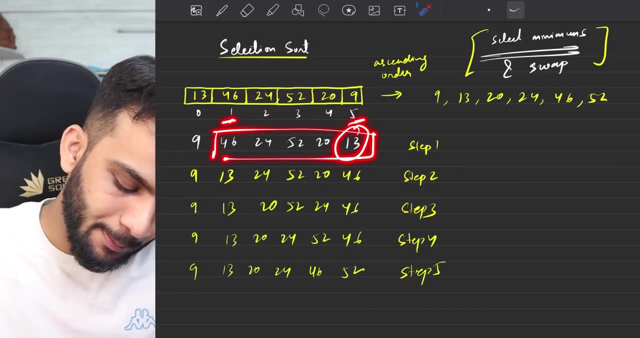 That's what I did. That's why 13 is here and 9 is here. So 0 to 5 is what I went. Next, I took this, which is from index 1 to index 5, and I got the minimum, which is 13,, and I swapped it with 46. 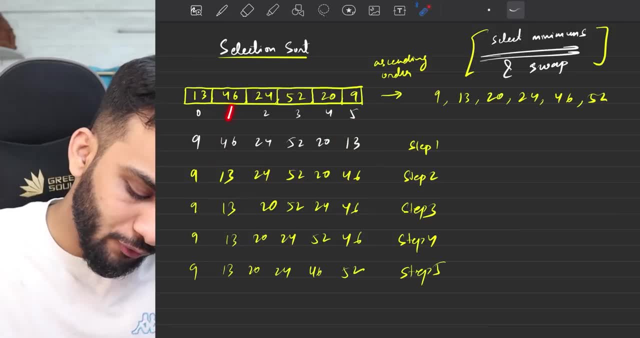 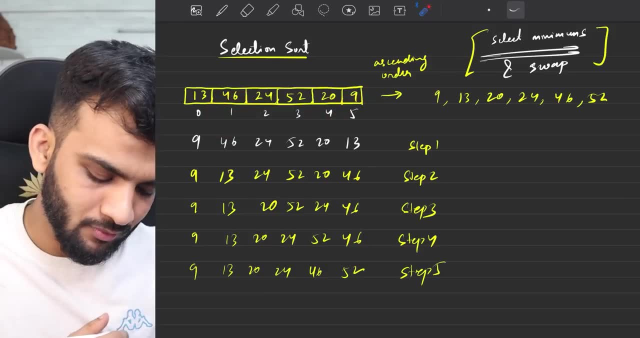 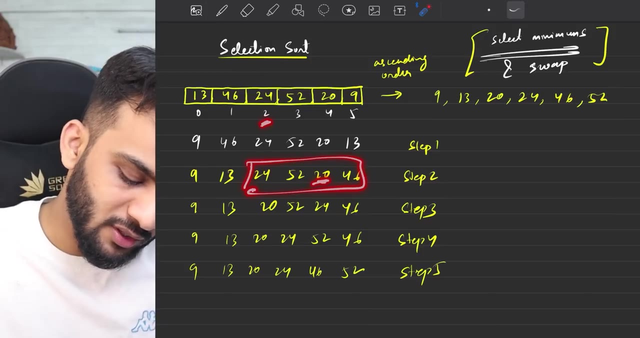 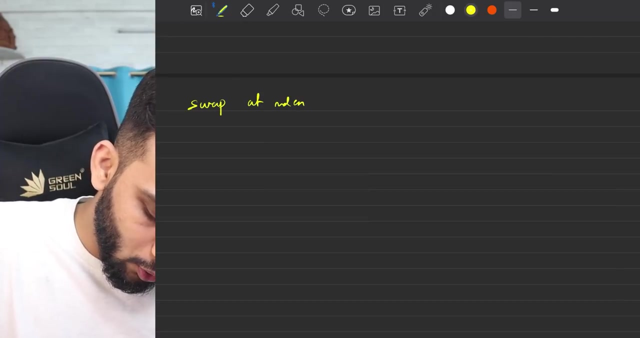 Thereby I got it. So I went from 1 to 5, and the swapping happened with 1 and the minimum Minimum. Next In this I got the minimum and the swapping happened from 2.. So can I say, first time swap happened at index 0 and minimum index. 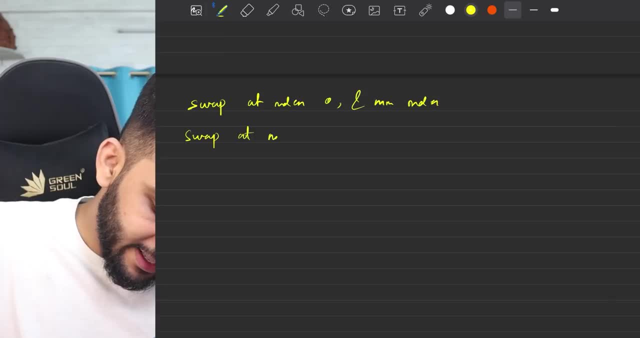 Next time swap happened at index 1 and minimum index, And this minimum index is from the array 0 to n-1.. This minimum index is from the array 1 to n-1.. Next time can I say swapping happened at index 2, because till that 0 and 1 are sorted. 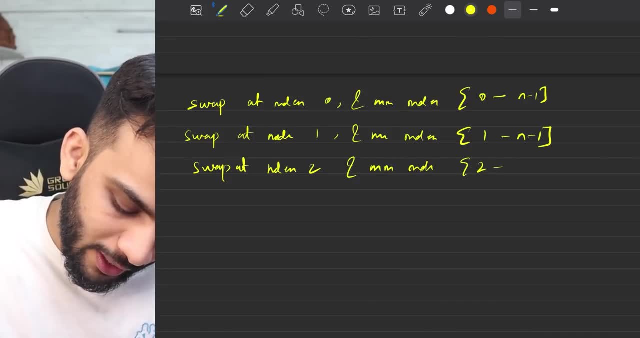 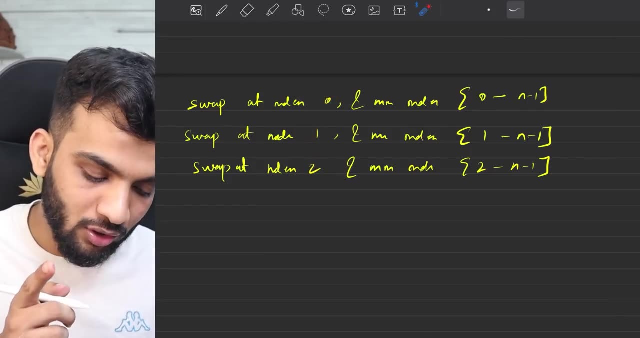 And minimum index this time is from 2 to n-1.. So can I generalize this And can I say this will go like 0,, 1,, 2.. Till, what Are you doing for the last guy? Are you swapping the last guy? 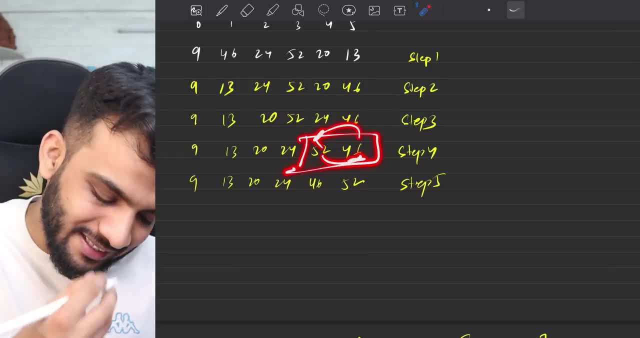 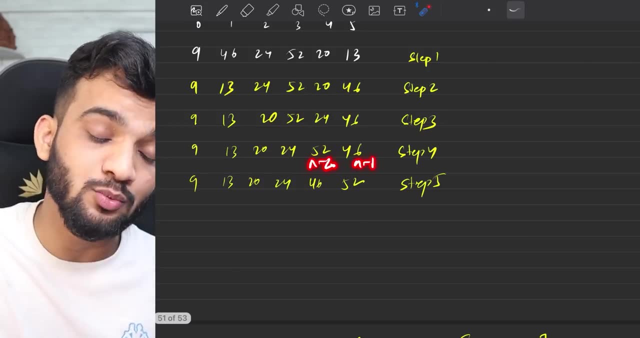 Is this still here? You got 46 and you swapped. Can I say it will go till n-2th index. Why n-2th index? Why? Because the last index is n-1 in arrays. So can I say: okay, swapping is happening. 0,, 1,, 2.. 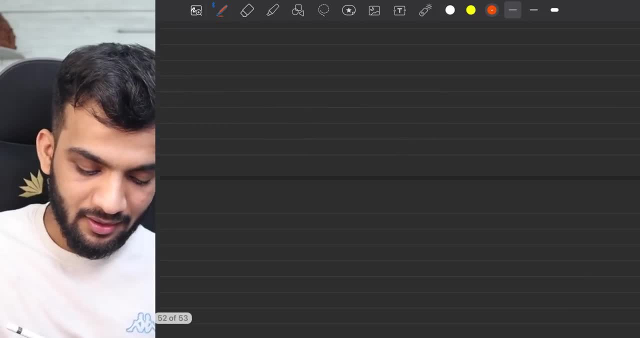 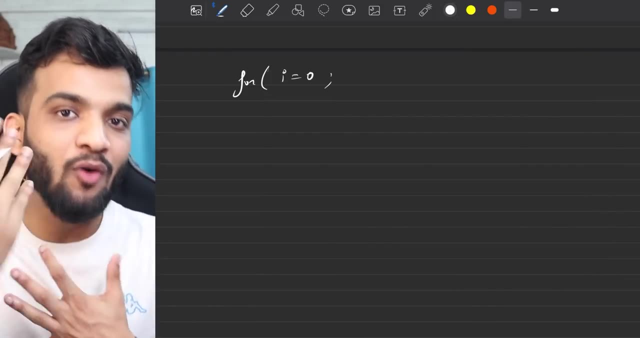 And it will go till n-2.. So thereby can I write this as like this a pseudocode: Okay, 0.. First time it will go 0., Next time 1.. Next time 2.. Next time 3.. 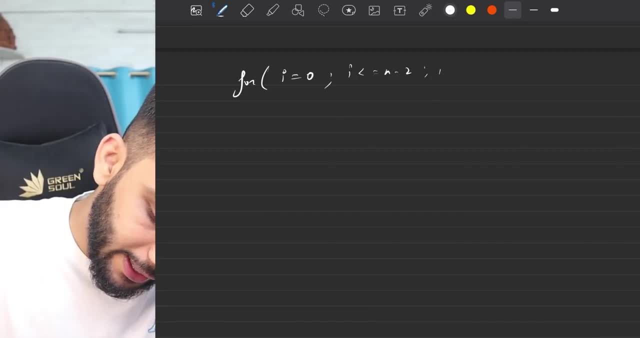 And it goes on till n-2 and i++. Can I say this: The first, And whenever i is 0,, I find the minimum from 0 to n-1.. Whenever i is 1,, I find it from 1 to n-1.. 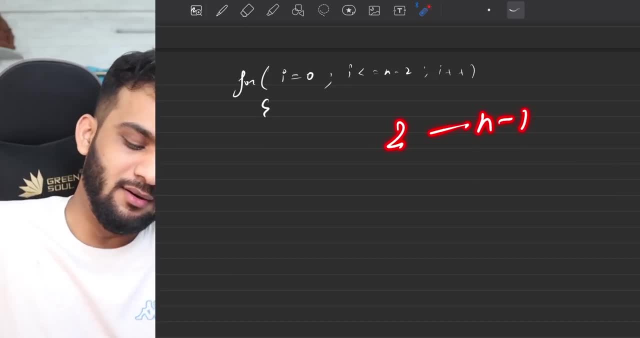 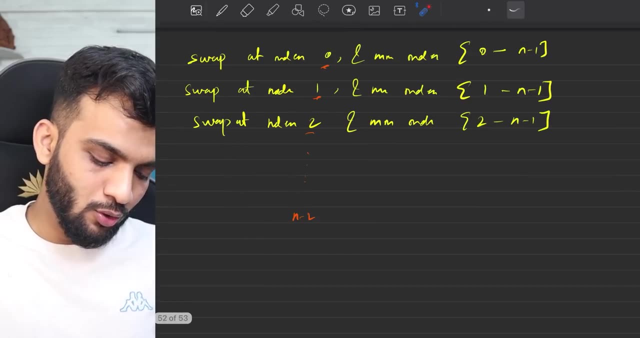 Whenever i is 2, I find it from 2 to n-1.. So can I say you need to find the minimum guy, Minimum. So we know one thing: i will be 0,, 1,, 2.. And there has to be an internal loop. 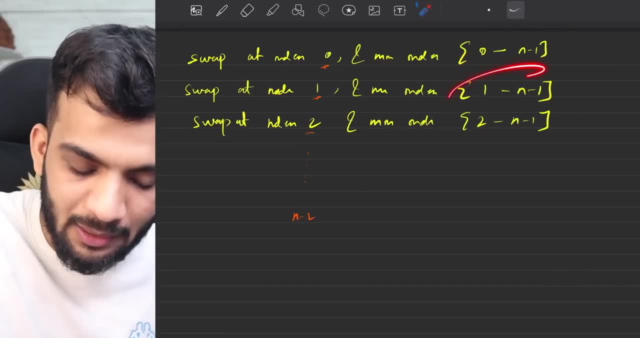 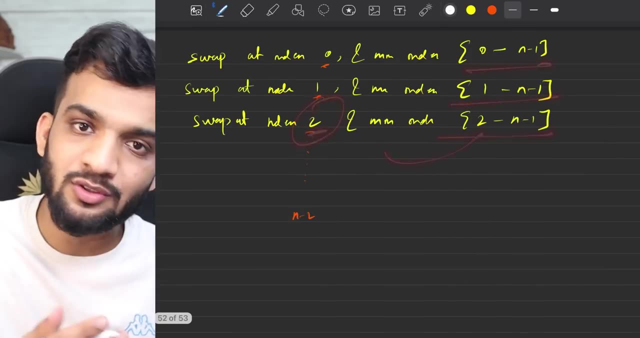 Why? Because you have to find the minimum in this range, Minimum, Minimum in this range, Minimum in this range. So the internal loop. can you observe something from 2 to n-1?? So write the internal loop. What are you waiting for? 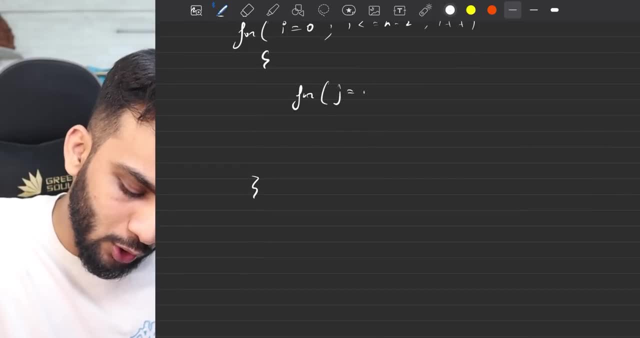 Write the internal loop. So can I say the internal loop will be from j equal to i till j lesser than n-1?? Because that is the last index until j++ And you need to find the minimum. I know the internal loop as well. 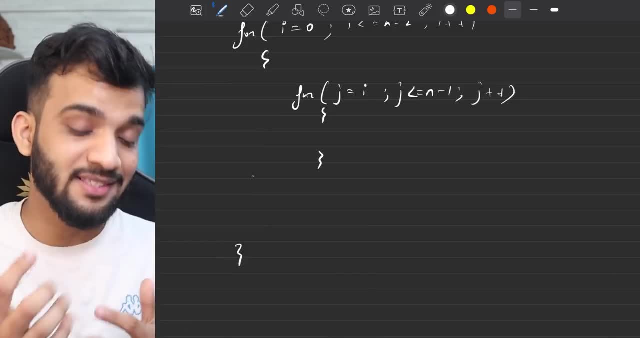 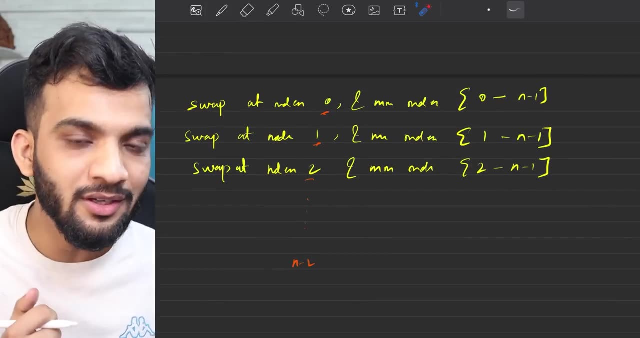 I know the internal loop as well. Now, what is the next thing you have to do In this range? in this range, you have to find the minimum. How do you do it? Very simple, Can I say: initially I will keep the mini. 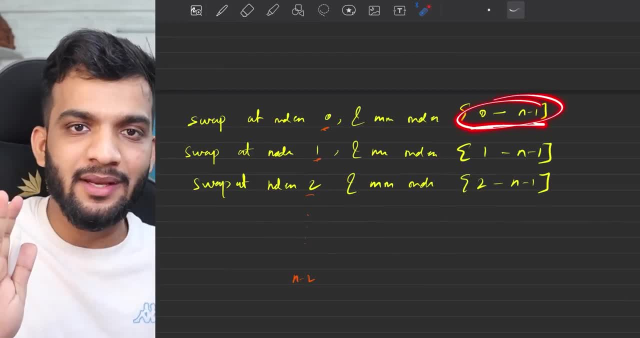 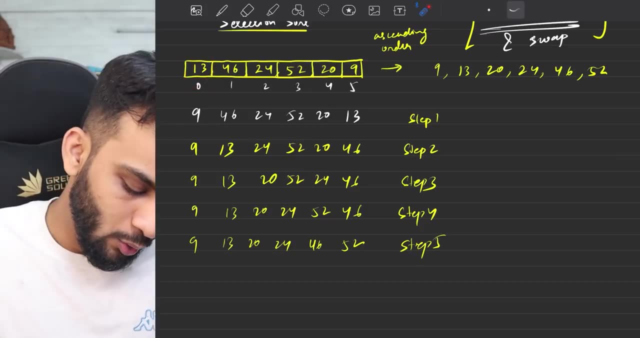 Just imagine. just imagine, Since your array is from 0 to n-1.. I will say: okay, while we start, let's consider this guy to be this small. While we start for this, let's consider this guy to be minimum. 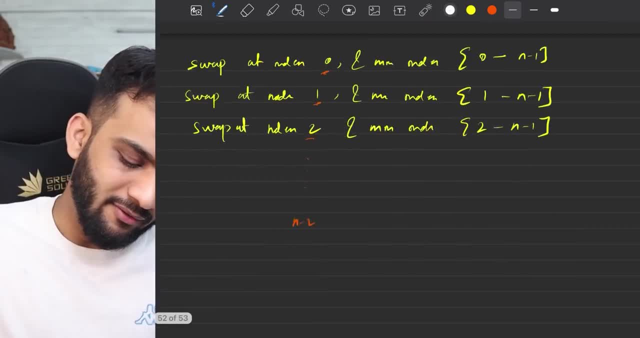 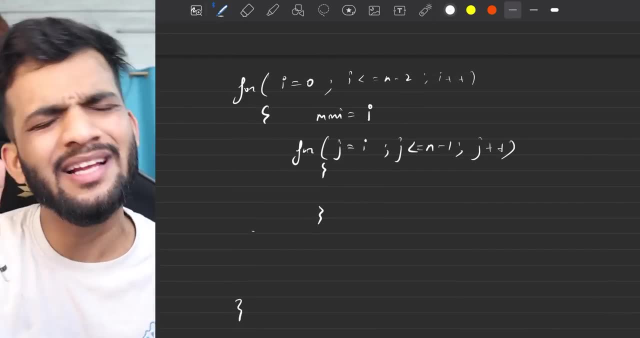 While we start for this, let's consider this guy to be minimum. So I will say So. I will say hey, my minimum appears at index i itself, At index i. Whoever is the first guy, let's assume he is the minimum. 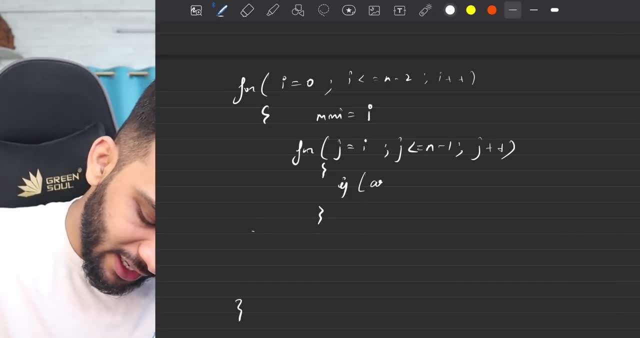 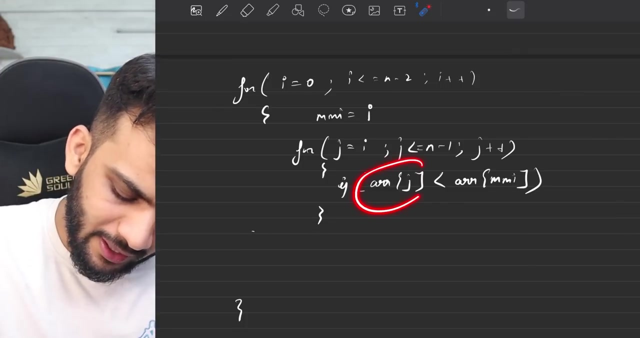 I am like: okay, Then I am saying: if array of j is smaller than array of whatever minimum index you are considering, What does this mean? When I am iterating, when I am iterating element by element, I am saying: hey, element, are you smaller than what I considered? 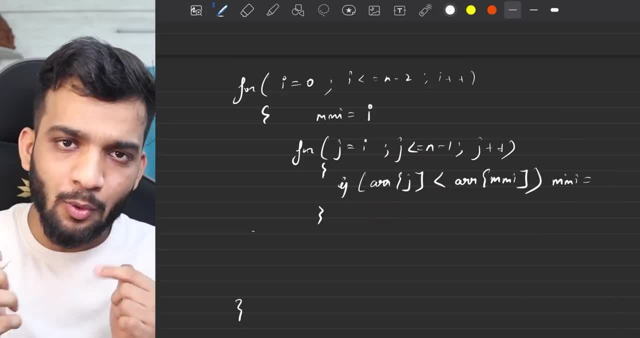 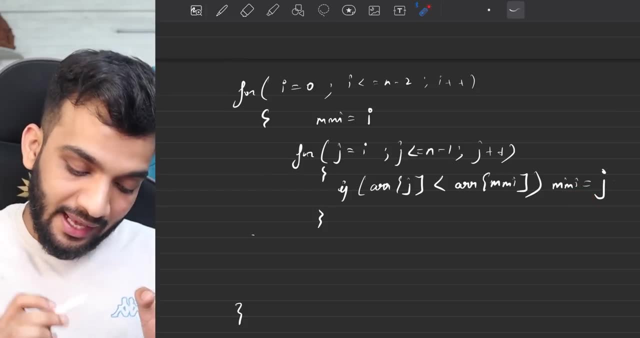 If you are, can I say minimum? okay, you are smaller, So my minimum appears at the jth index, not at this guy. I updated, So can I say once you have iterated? can I say once you have iterated in the entire thing? 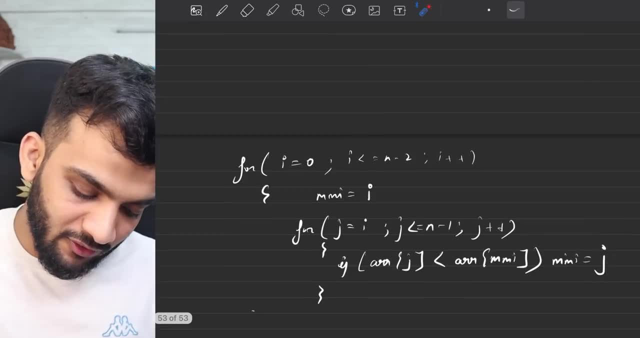 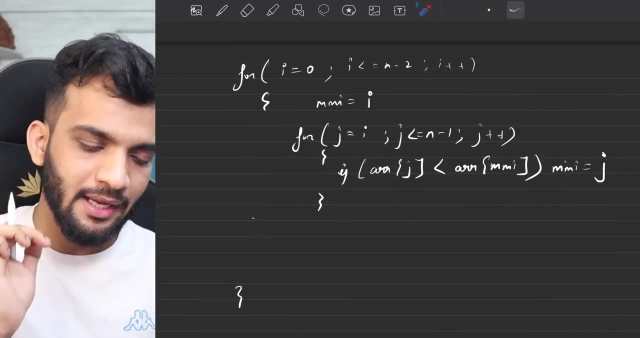 you will get the minimum index stored at the mini variable. You will, you will right. So, once this is completed, what did we do? Let's go back to the algo. What did we do? So if you are iterating Over here, what will happen? 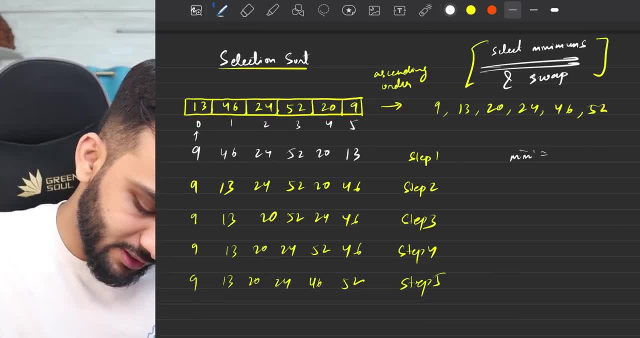 Let's see: Minimum initially is 0th index right, The minimum is 0.. What happened? Let's see In iteration: we are taking 13.. It's like 13,, lesser than 13, because minimum is 0.. 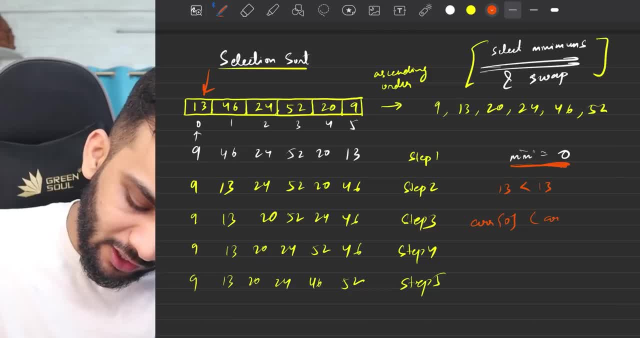 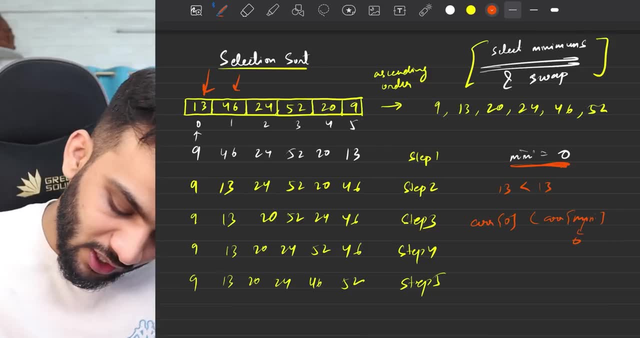 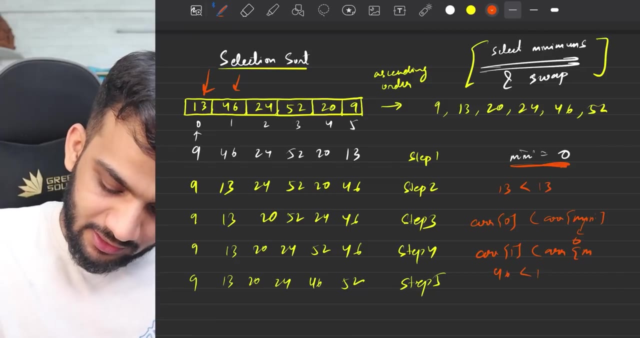 What happens? Array of 0, lesser than array of mini, because mini is 0.. It's not there, So it doesn't work. Next it goes here: Array of 1, lesser than array of mini. It's like 46, lesser than 13.. 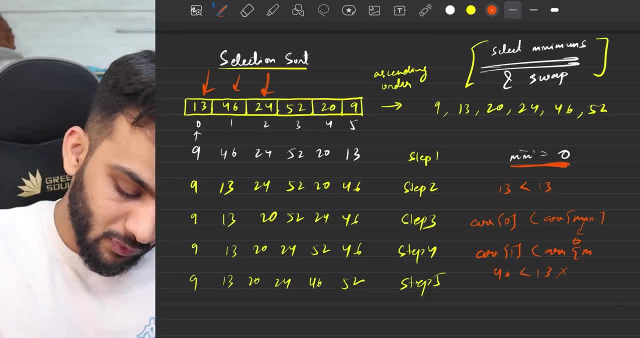 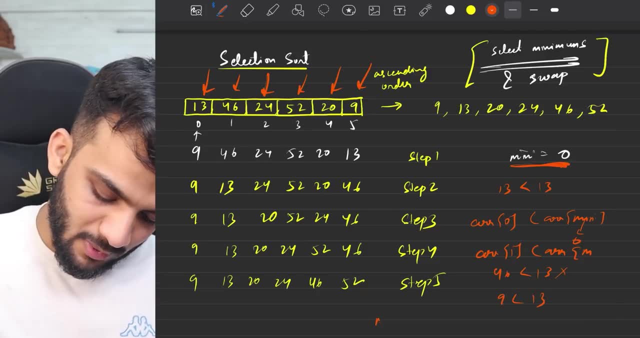 No Next time: 24, lesser than 13.. Next time: 52, lesser than 13.. No Next time: 20, lesser than 13.. No Next time: 9, lesser than 13.. So the mini gets updated to 5.. 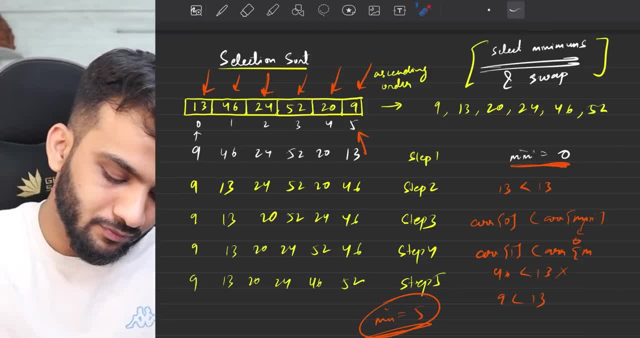 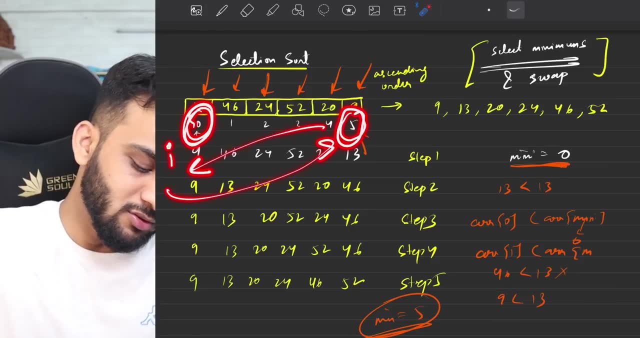 So you know, at the 5th index, the mini is, what did you do? You took the mini index and you took the ith index and you swap, and you swap. So you can just do a swap, You can just do a swap. 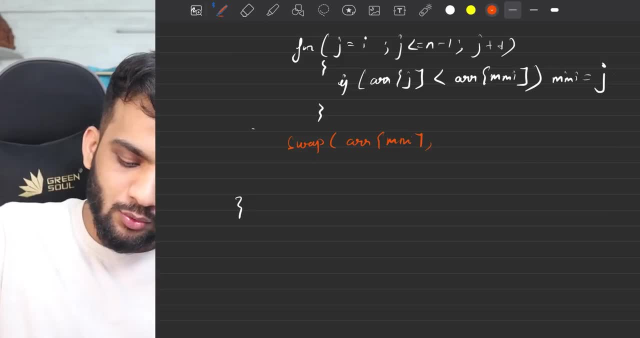 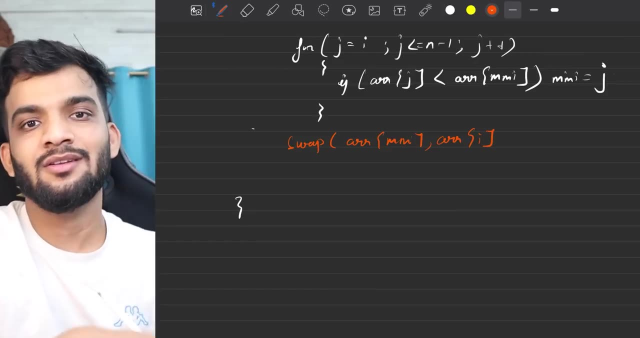 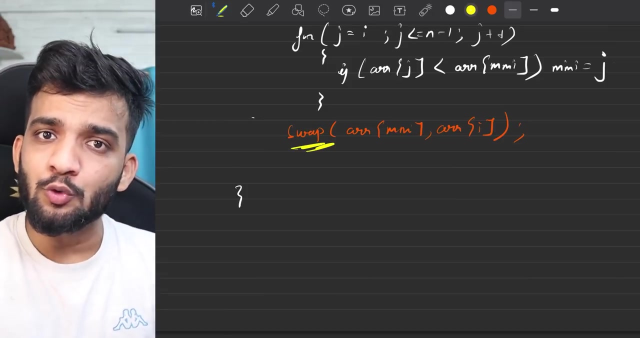 Swap of wherever is the mini, whatever is the value with the first guy, because if you have to take that mini and place it at the first, first will go to that mini index. So the swap is also done. Simple as that. So, by the way, how do you swap two numbers? 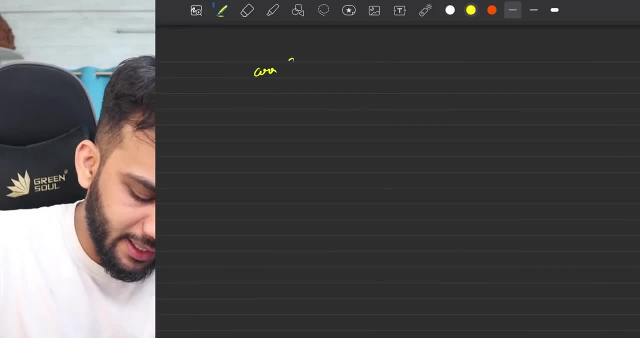 It's very simple. Imagine I have array of i and I have array of mini. Okay, These are the two numbers that I have to swap. Imagine this is 15 and this is 12.. So what I'll do is I will take a temporary variable. 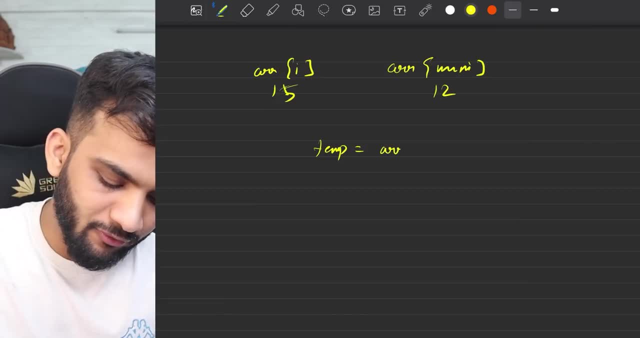 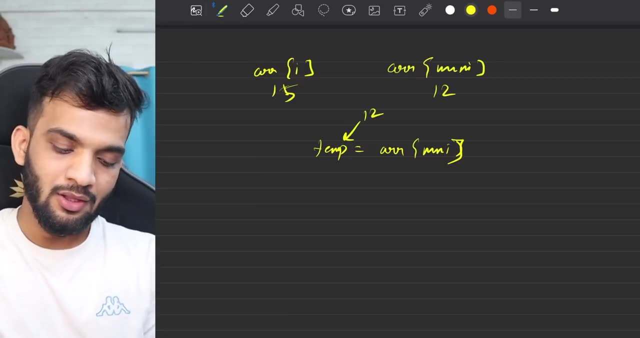 That's another third variable that I'll take, and I'll say array of mini to go there. So what will array of mini, what will temporary have? as of now, 12, because array of mini is 12 and that was put in to the temporary. 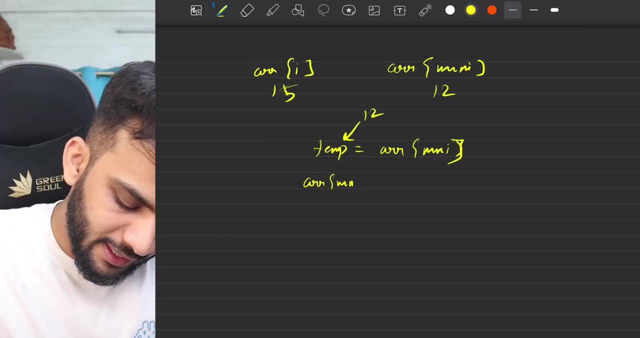 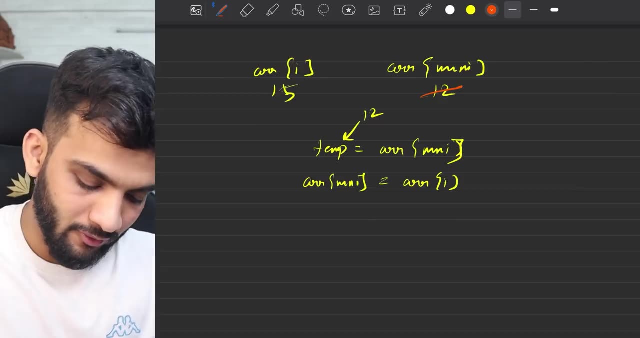 Now what I'll do is I'll say: array of mini. Can you replace yourself To array of i? So what will be the value of array of mini will not be 12.. This value will go here and this will become 15.. 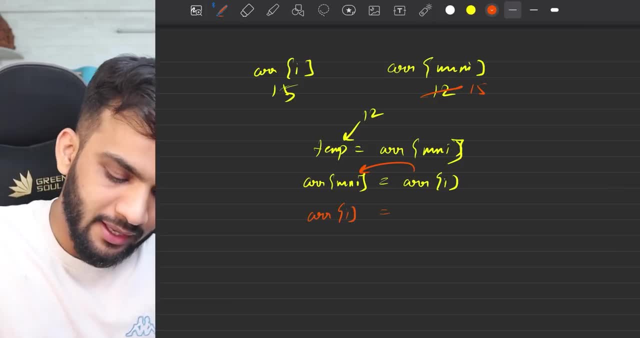 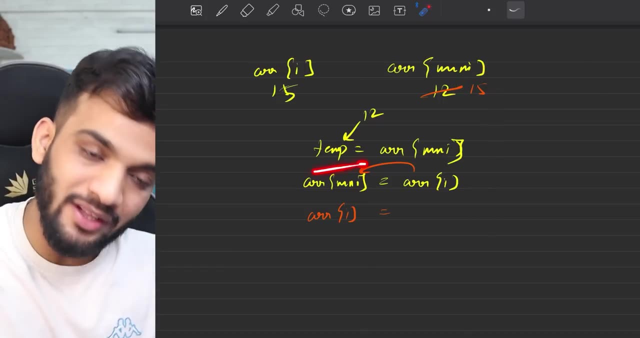 Right now I will say array of i. Hey, array of i. Can you take the value of array of mini, but it is replaced to 15.. This is where, since you stored in the temporary, that works and is a temporary, Can you get it? 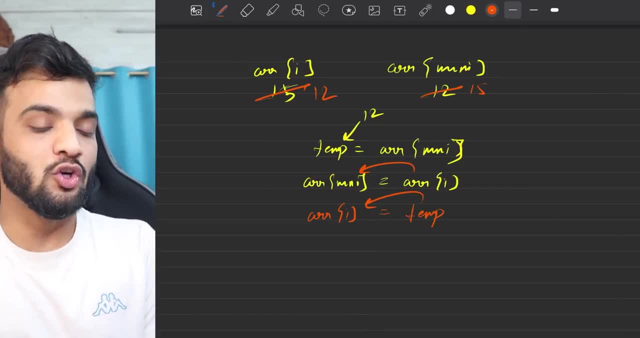 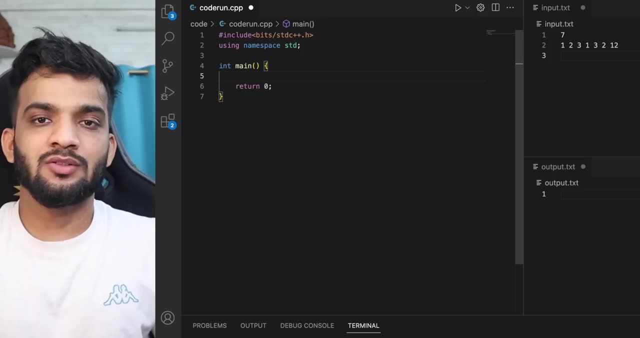 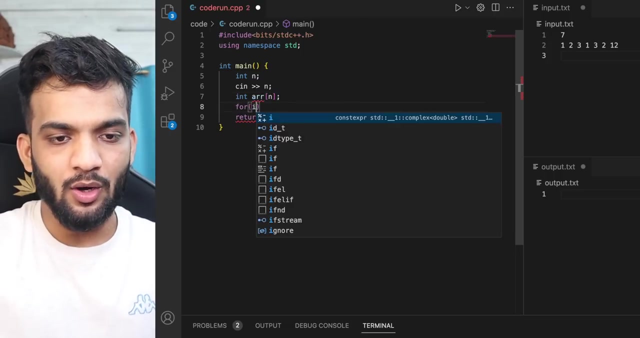 The temporary will get it and this will become 12.. So this is the swap that you have to write. This is the pseudocode of swap function. So if I had to code it up, imagine I have given the end, I take it as the input. then I take this array of n and then I go across and I say this: 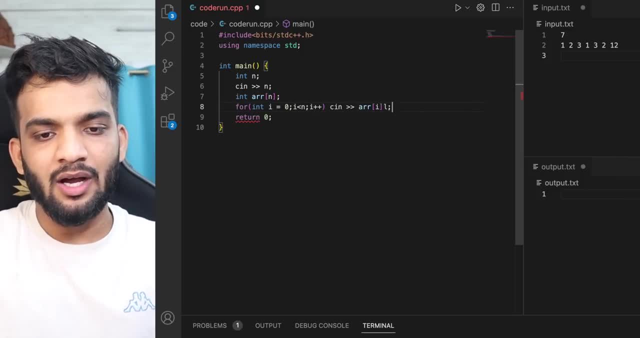 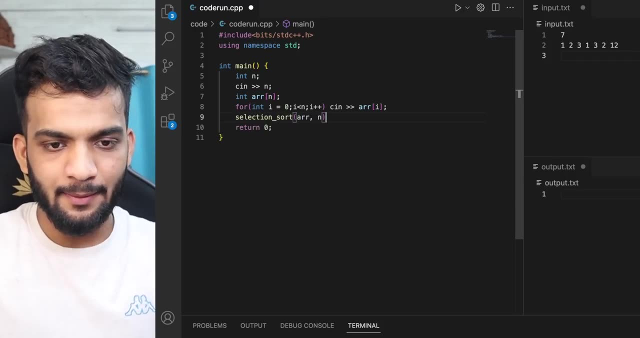 So this is basically nothing but the array input that I'm taking. now I have to write the selection sort, So maybe I can say selection. I'll just pass it into the function. I'll pass it. Let's write the selection sort. 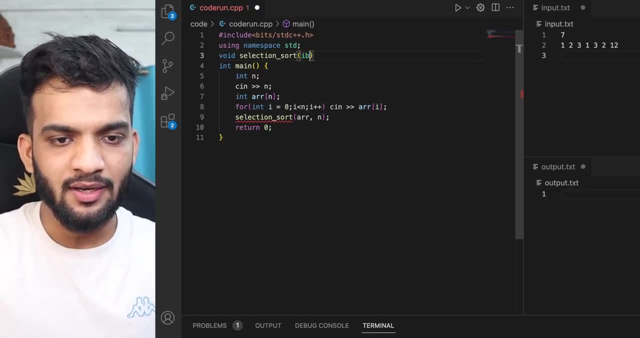 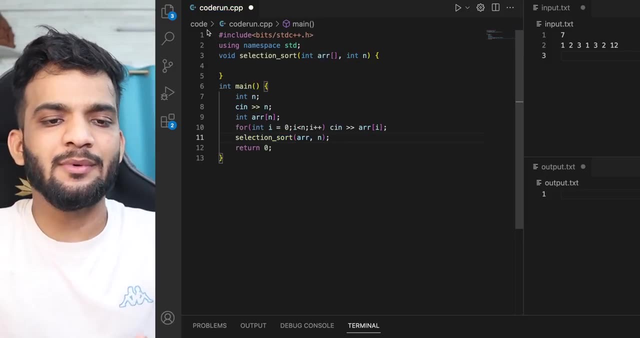 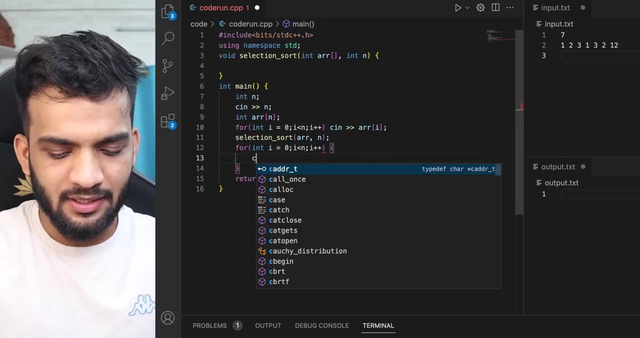 So void selection And this will be sort and I'll say: let's take the array, Let's see the end. So I'm passing this and I'm assuming this will do it and post this. What I'll do is for int, i equal to 0, i less than n, i plus plus. 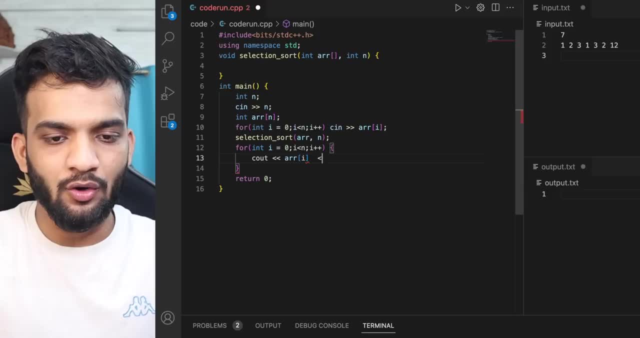 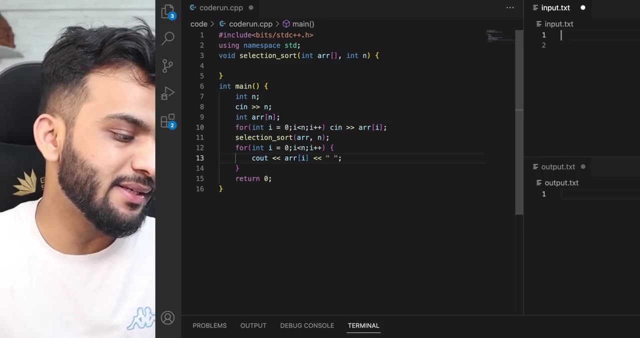 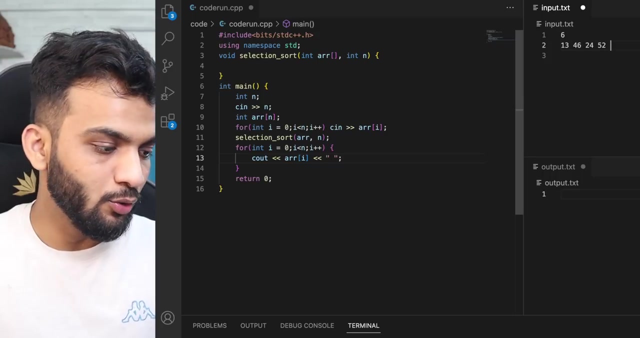 Can I print the array values to see if they are sorted or not? Okay, let's see if they are sorted or not. And what we can do is we can take the same example that we took, that six numbers 13,, 46,, 24,, 52,, 20 and 9.. 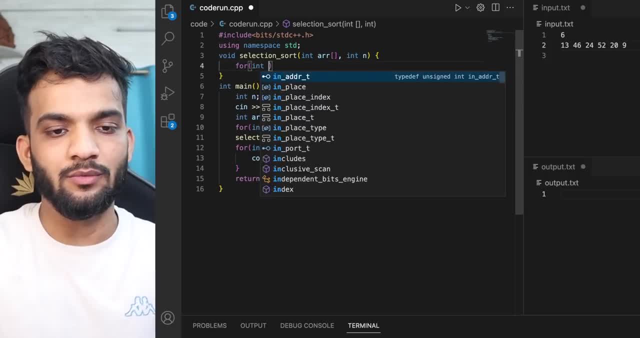 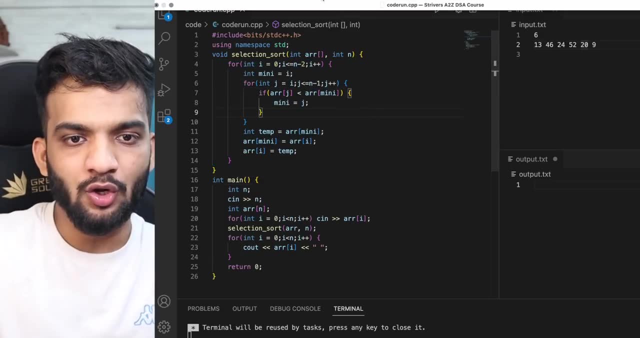 I took the same example over here. Let's quickly write the code. So whatever pseudocode I did write, that I've converted into code now over here And if I go across and run this particular task, you will see that this particular array is sorted over here in the outputtxt. 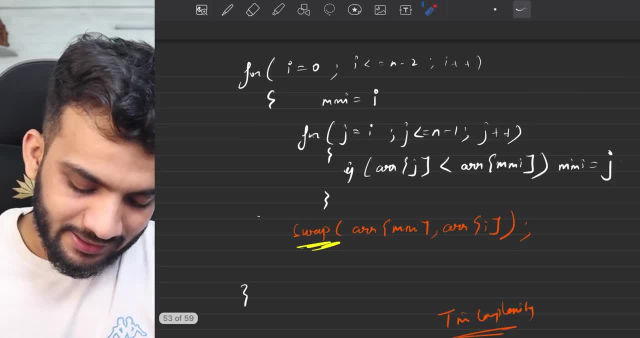 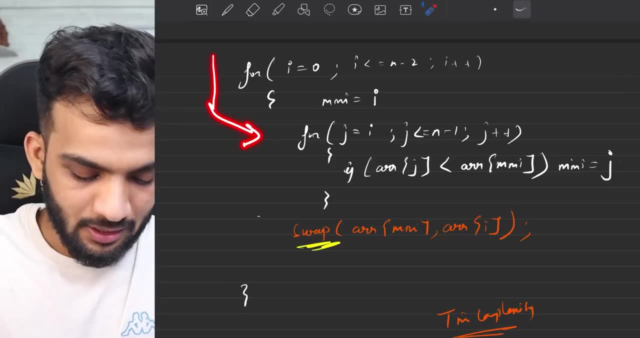 So you have understood the selection sort algorithm in depth. It's time to analyze the time complexity of this particular algorithm. Let's see, Can I say for the first time, when the loop gets inside. this particular loop runs for n times exactly Yes. 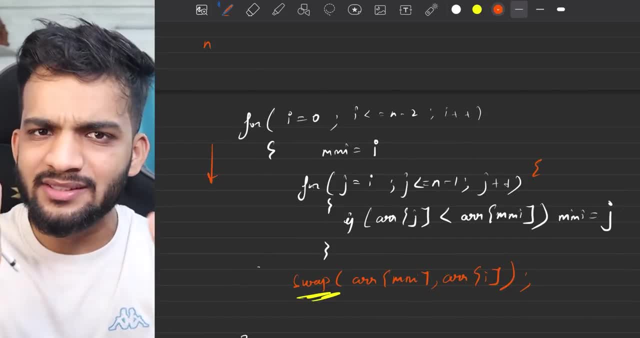 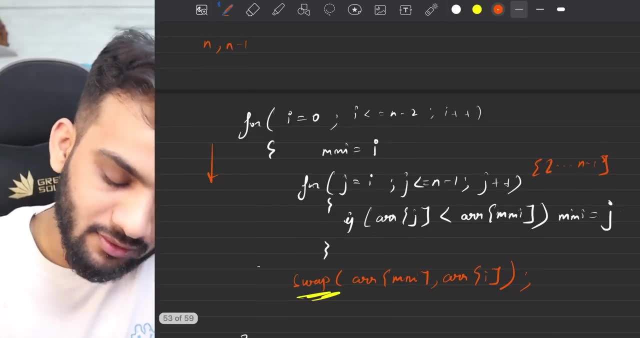 Next time when it gets in, then this actually runs for 1 lesser. It runs for 1 to n minus 1.. So can I say it runs for n minus 1?? Next time when it gets in, it runs for 1 lesser. 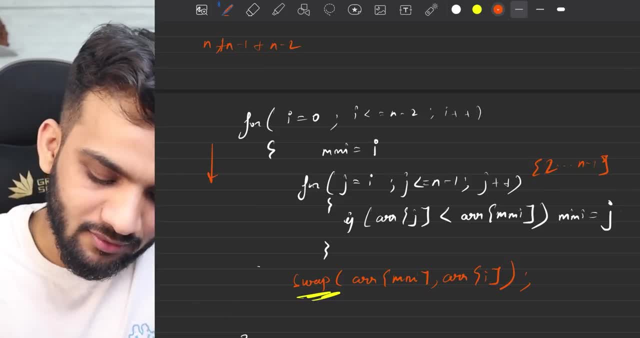 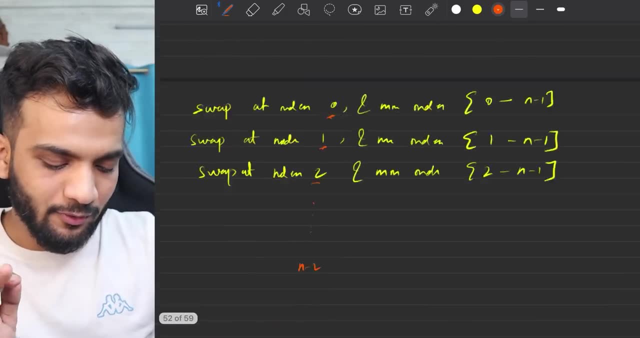 So it's like n minus 2.. Next time when it gets in, it runs for 1 lesser, n minus 2.. So on, it kind of runs for till last. Last that we run for this is till here. That's for two types. 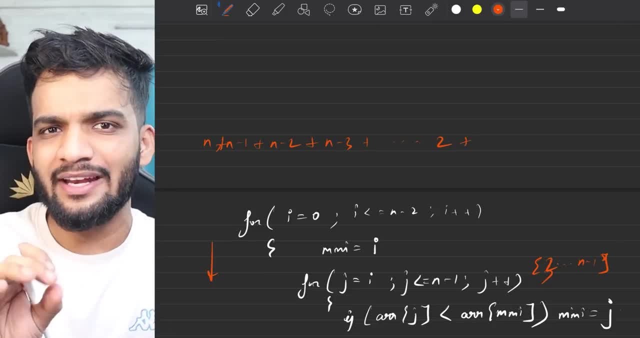 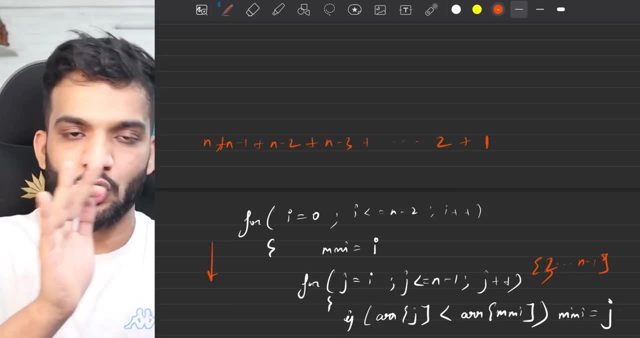 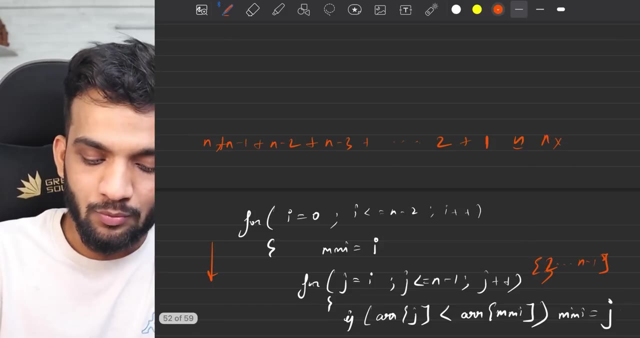 So this is kind of kind of- if I just try to take it to some near near formula stuff, Can I say it's something like 1 plus 2 plus 3 plus dot, dot, dot till n, which is nothing but the summation of the first n natural numbers, which is n into n plus 1 by 2.. 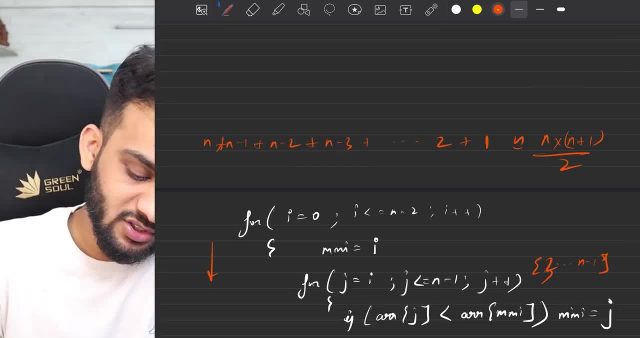 Can I say this? I can. If I can say this, what is this? n square plus n by 2.. Can I say this is how it looks like? And if you remember the time complexity, remember the time complexity lecture we did, we ignore. 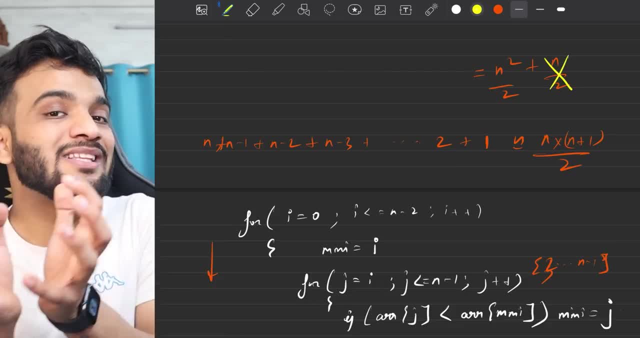 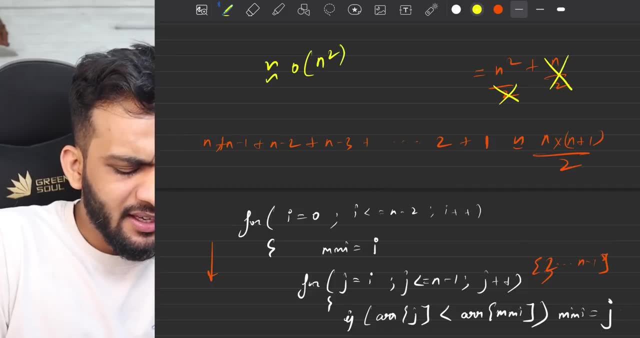 smaller things, because n by 2 in comparison to n square is very small and we ignore constant. Thereby I can say that the time complexity Is near, about b go of n square. and this is the best, This is the worst and this is the average time complexity for this particular algorithm. 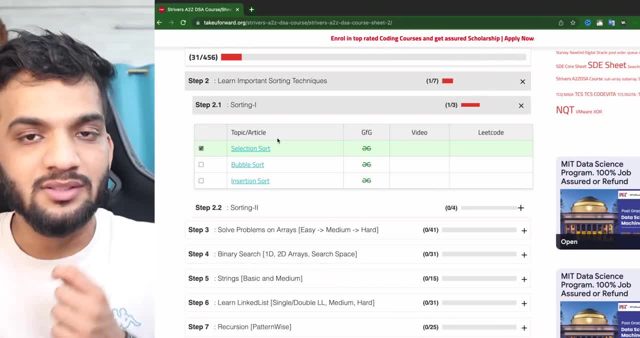 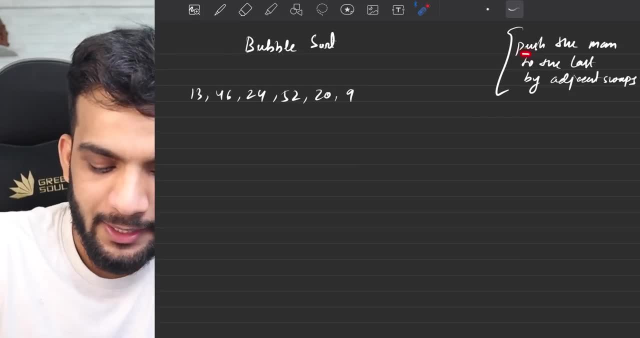 So we can say that we have completed selection sort successfully. That's time to understand bubble shot, Bubble shot. So when you talk about bubble shot you have to remember it pushes the maximum to the last and opposite to the selections, because selection sort was taking. 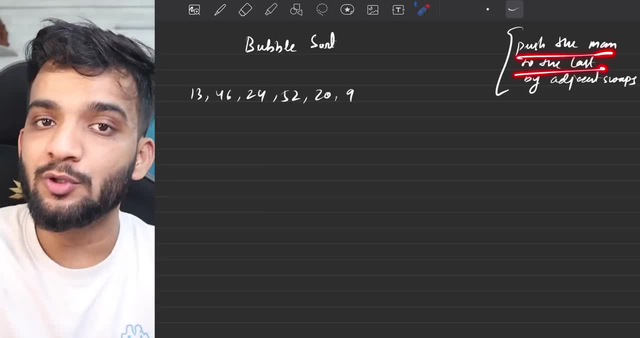 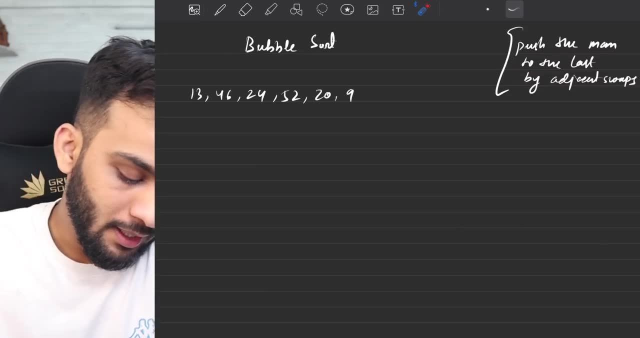 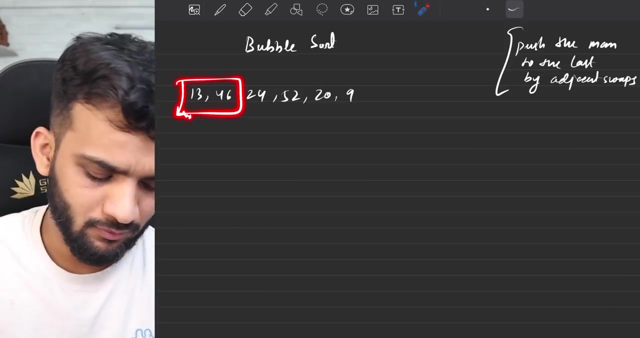 the minimum at the front, If you remember, pushes the maximum to the last. how does it do it? by adjacent swapping. Adjacent swapping is the key over here. How does the algorithm work? Let's understand. first, two elements compares are the, in the sorted order, 13 and 46.. 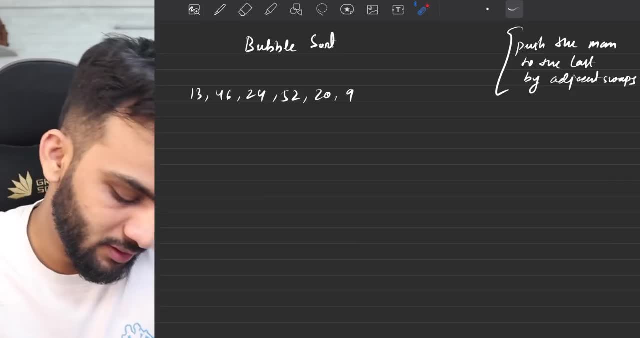 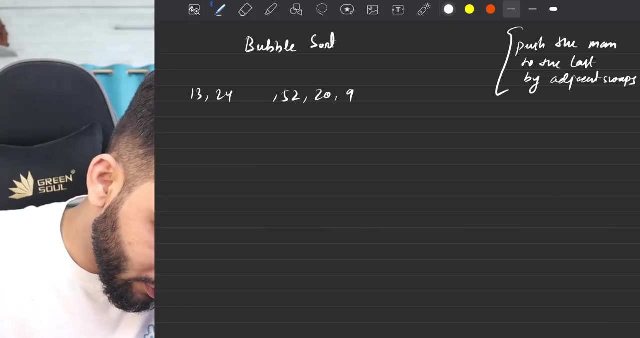 They are because 13 is smaller than 46.. Do not do anything. Go to the next two. Are they the sorted order? 46 before 24?? No, Swap it Okay, Stop 24.. 2446. Perfect. 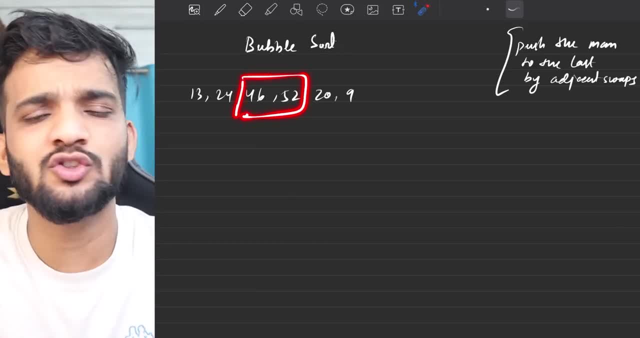 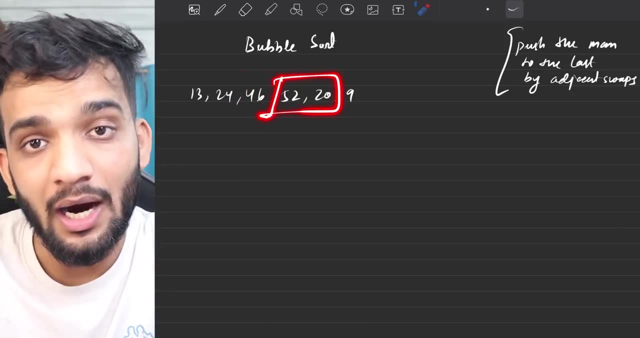 Let's go to the next 4652.. Are they in the sorted order? Yeah, they are. Why will you do any? Next, 5220.. Are they in the sorted order? No 20 should be before. take 20 here. 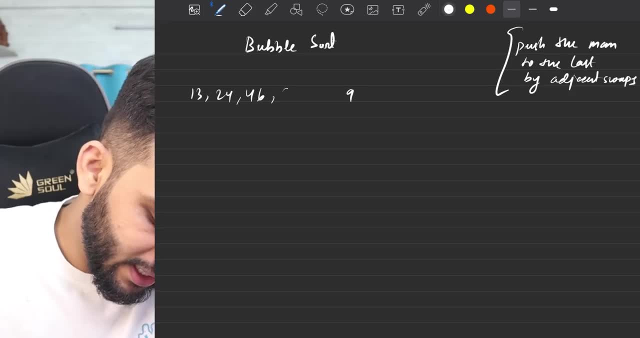 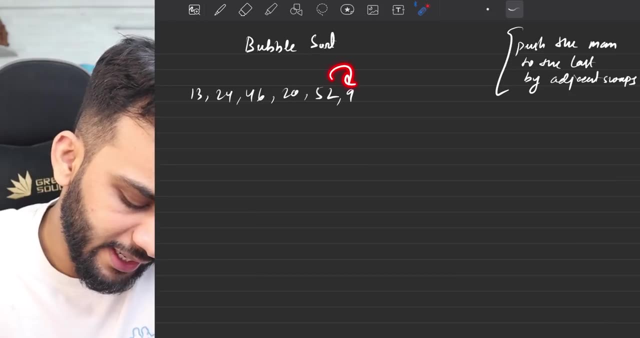 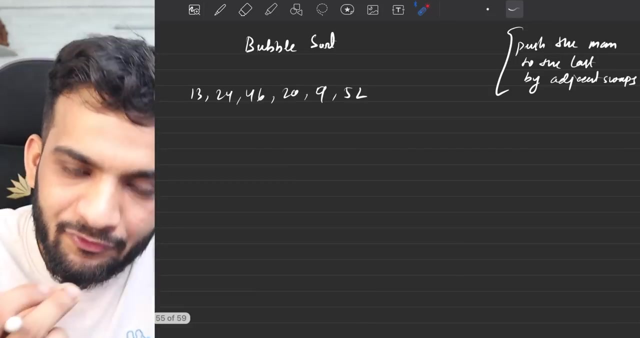 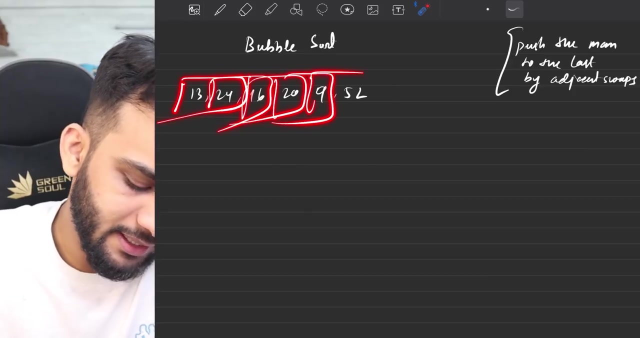 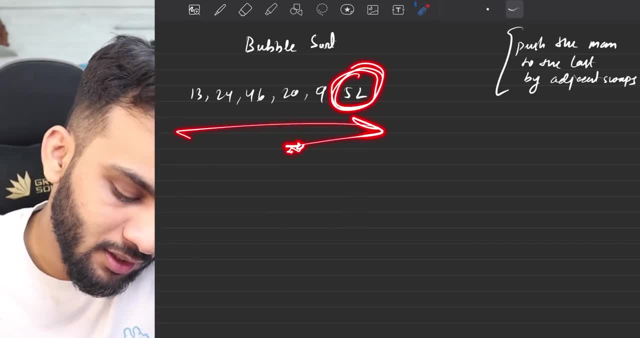 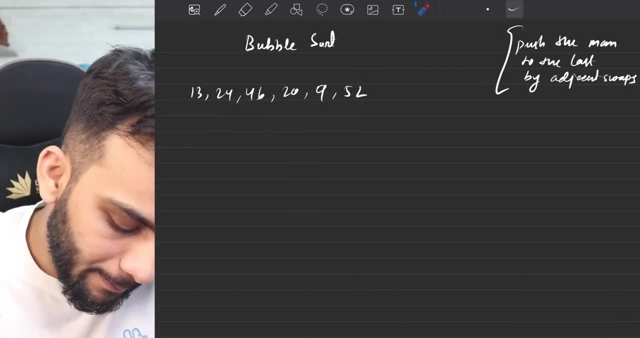 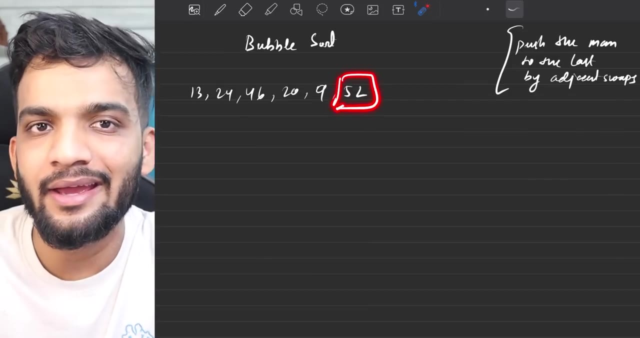 adjacent swap checkings. Do you observe something? The max 52 is at the last, the max 52. Is at the last. done to the max 52 is at the last. What should be your next step? This portion of the array is kind of sorted. 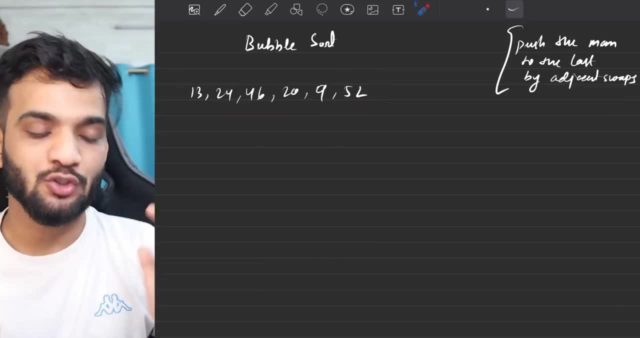 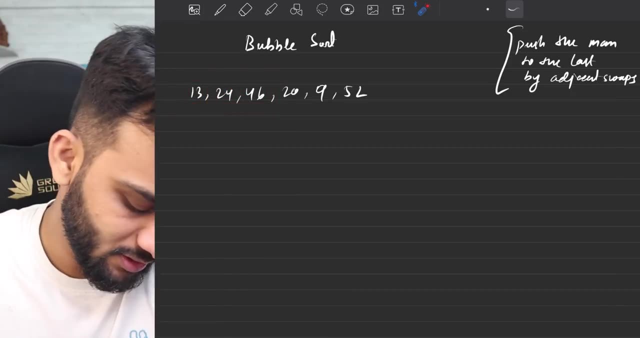 So I need to work on this, perform the same algorithm again. Let's do it: 1324.. Is it okay? It is 2446.. Is it okay? Is 4620? No, no, no, no. Trap 46 here. 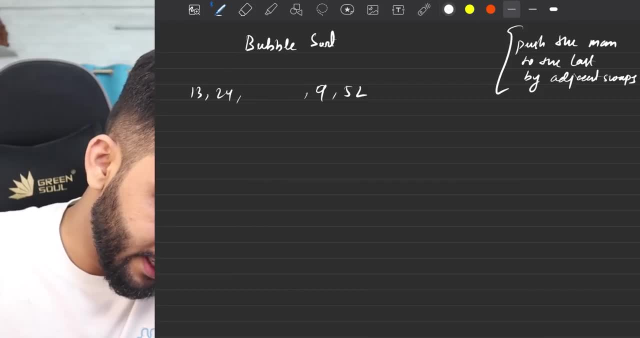 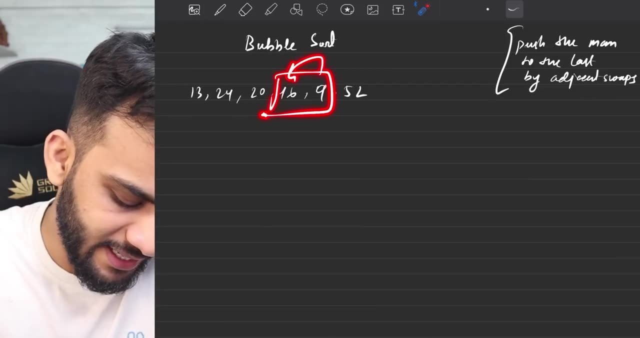 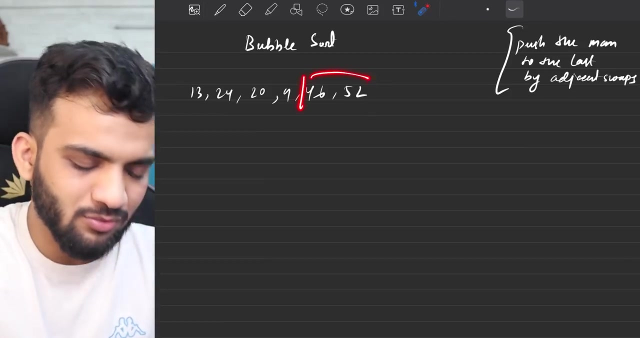 Take 20 here, Let's stop it- 2046.. Let's do the next 469.. Are they? No? no, take nine here. Take 46, here 946.. Do you compare the last two? There's no point because 52 is already in the sorted file. 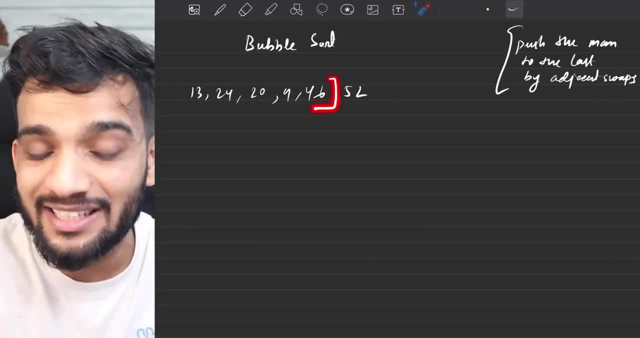 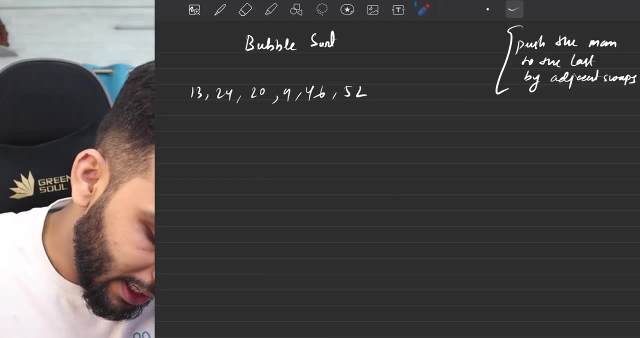 There's no need. Do you only do it till here? Can I say now, In this particular array, 46 was the maximum and it's at the last. Thereby, after two steps, the last two are in the correct orders, So step one is done. 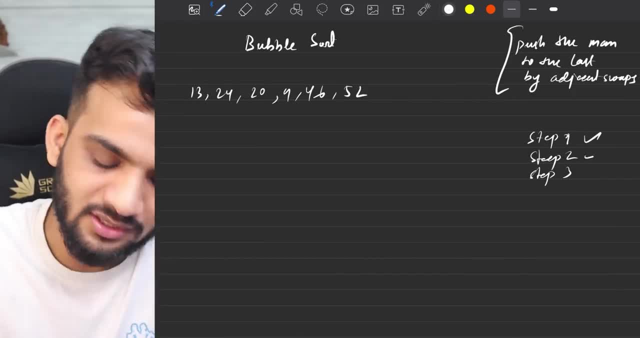 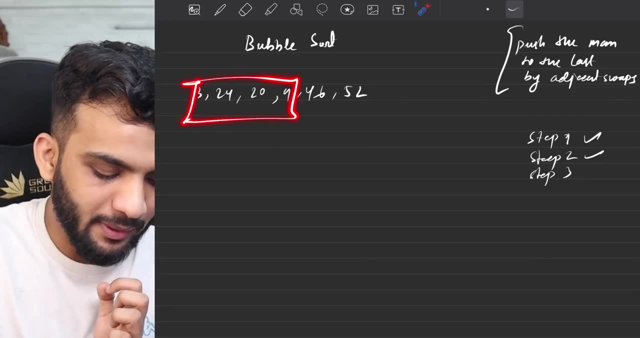 Step two is done. Let's do the step three. So this is done. This is done. Let's do the step three. Step three means this portion should be making sure that the maximum is over here. Let's do it 1324.. 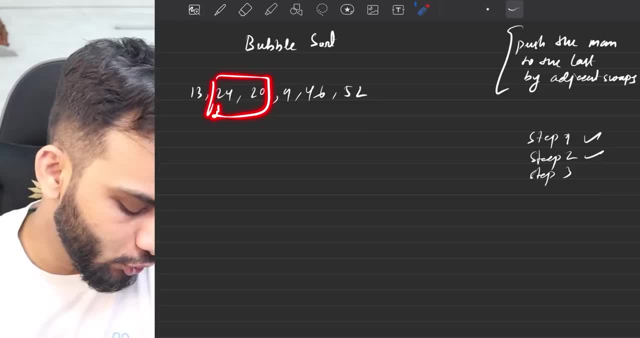 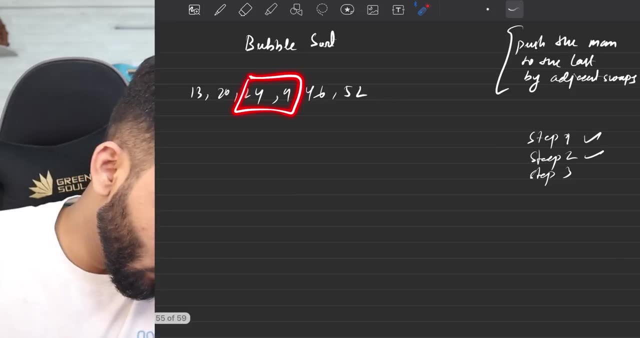 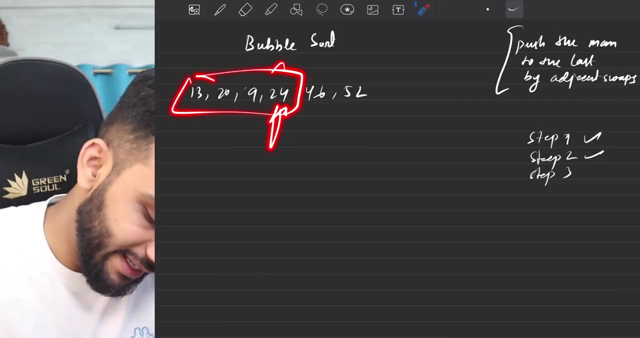 Are they? They are 2420.. No, no, no, Trap it 2024.. Next, 249.. No, no, Trap it Done In this. 24 was the maximum. It's, at the last Step, three done. 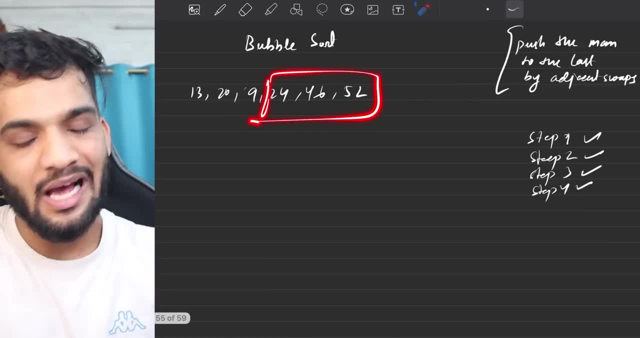 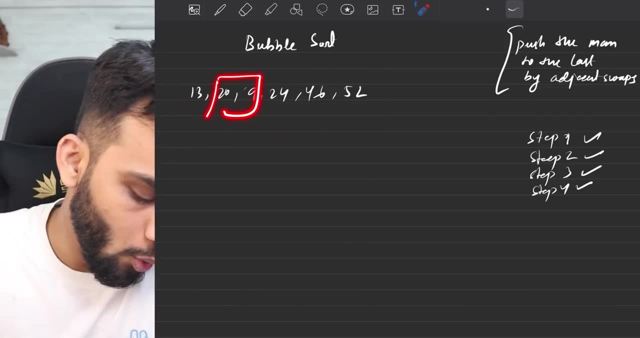 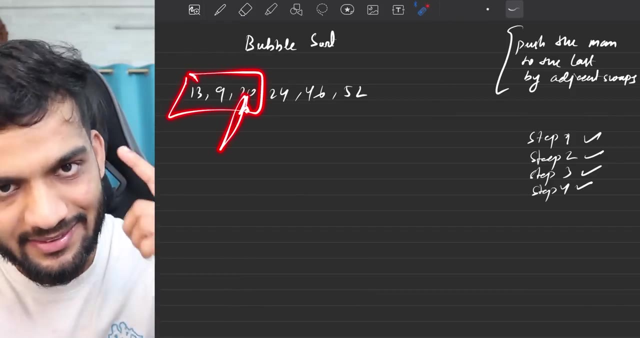 Step four, Can I say? step three means last three elements done. This is left: 1320.. Correct: 29.. No, Trap, Trap, Trap: 920.. Can I say for this, 20 was the largest and it's at the last. 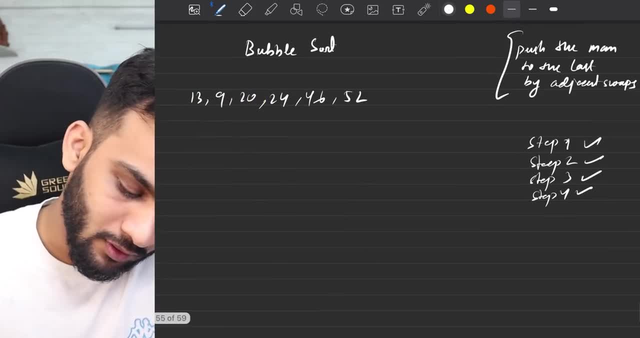 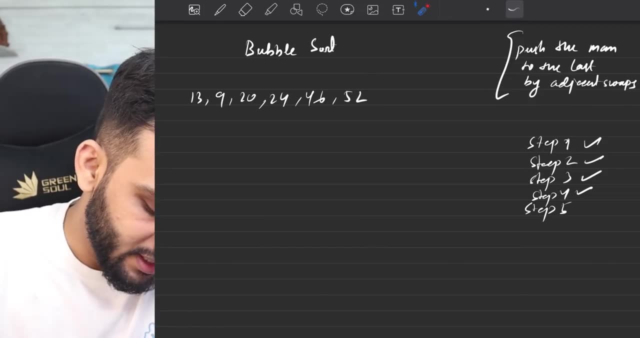 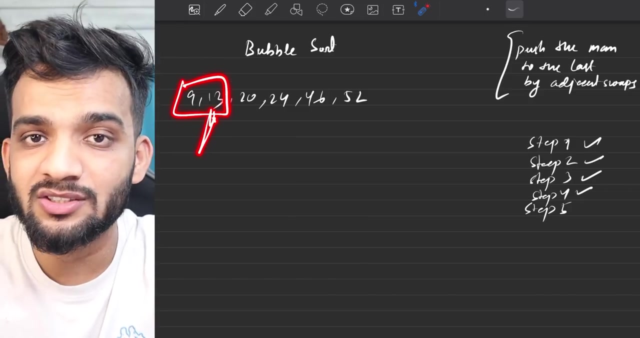 So thereby post step four. This is done. Next step five: What is step five? This? Let's do a comparison. No Trap 913.. For this portion, 13 was the maximum and it's at the last. So for this portion, 13 was the maximum and it's at the last. 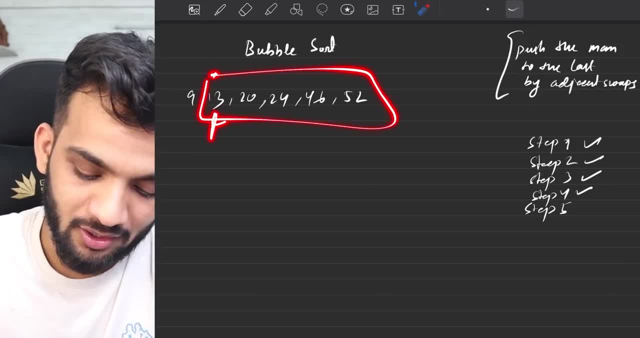 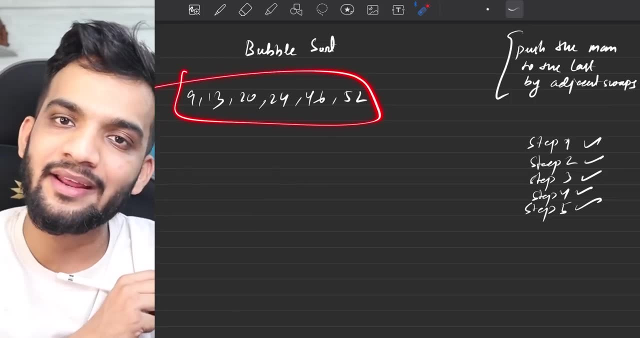 So thereby This portion is sorted. post step five, Do you need to do for a single element? You do not. Thereby the entire array is sorted, If you see So? if so, you have understood the algorithm. but now the key factor comes. 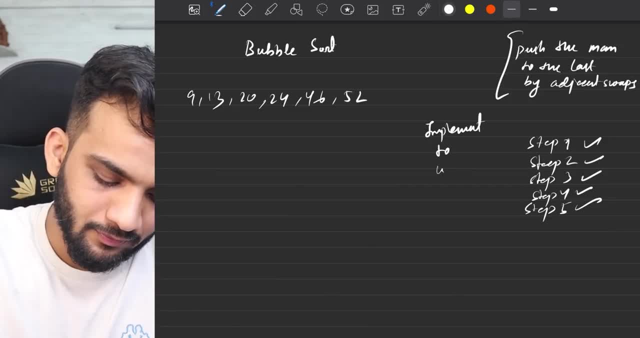 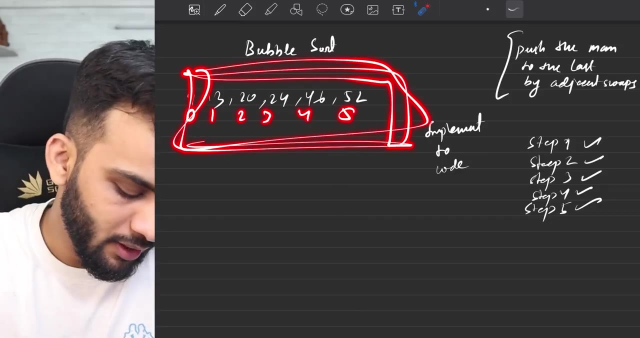 in which is implementing this to code, Because that is where the key lies. Let's try to do that. What are we doing? Observation is the 012345.. We're going till The first step. we went everywhere and we did. 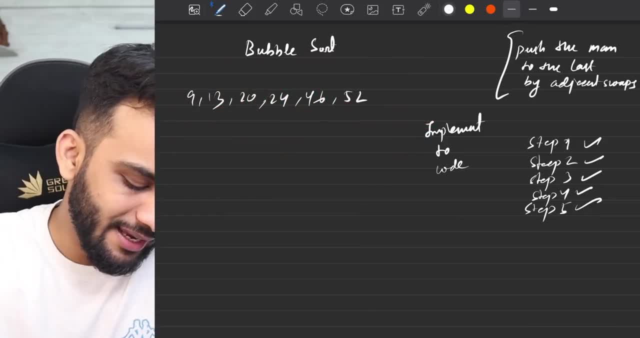 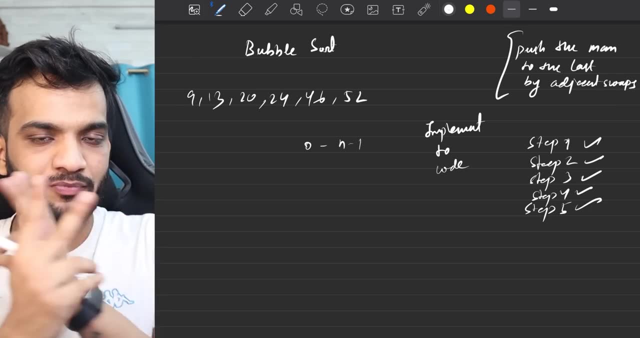 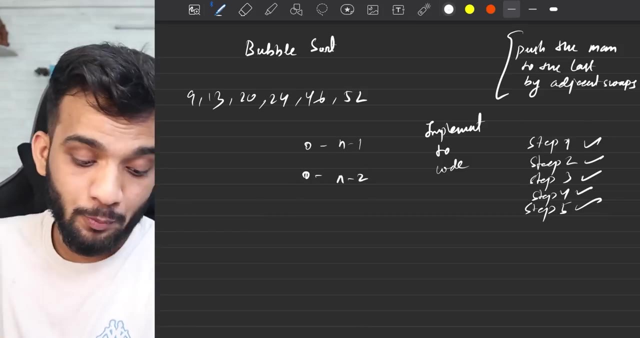 Add, just in company, Though: for the first time we kind of went Tell 0 till n minus 1 and we did adjacent facts If, if it was not in the order, next time you went like 0 to n minus 2 because the last was, so next time we went from 0 to 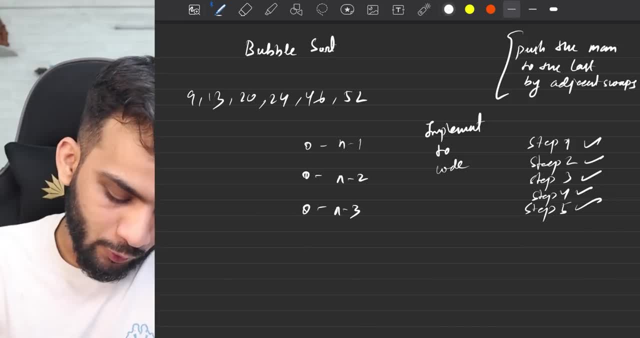 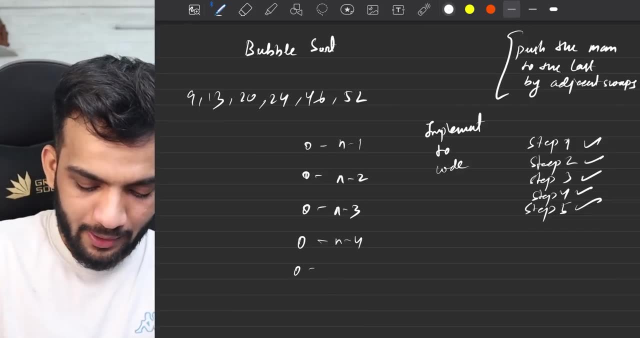 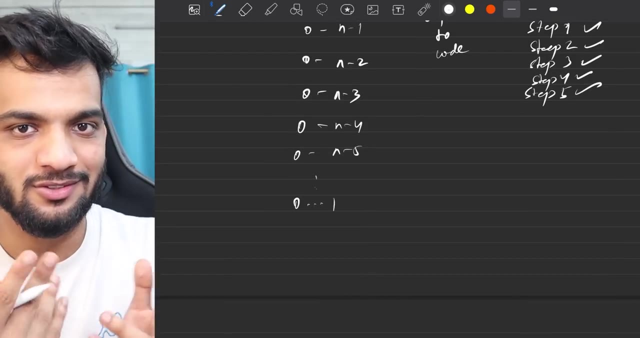 N minus 3. next time we went to 0 to n minus 4.. Can I said this is what we are doing and the next time 0 to n minus 5, and so on. Can I say I will just do till 0 to 1, not till 0 to 0, because one element. 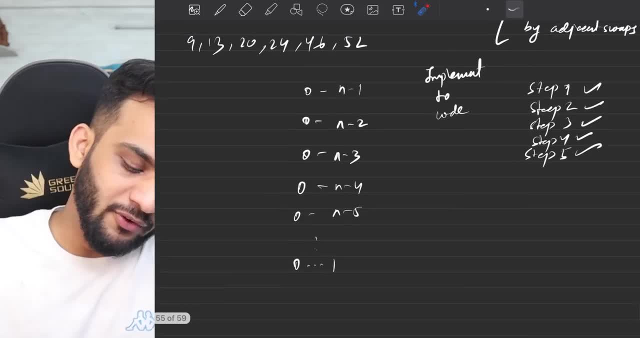 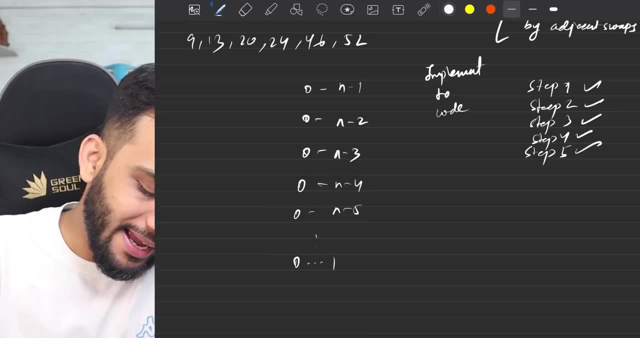 will not matter to them If you carefully observe. First loop should run from here to next loop should run from here to here to kinder. Can I say I can probably keep The value of I from n minus 1 till I. can I keep? I can if I do it. I. 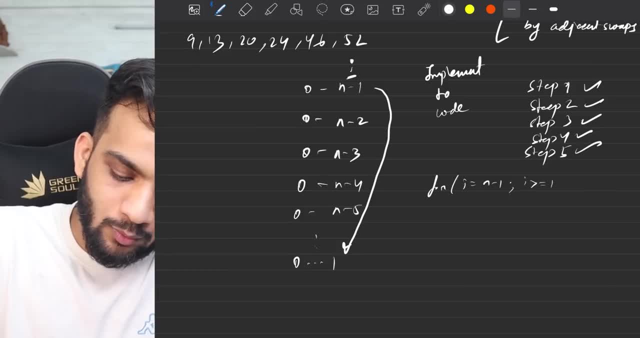 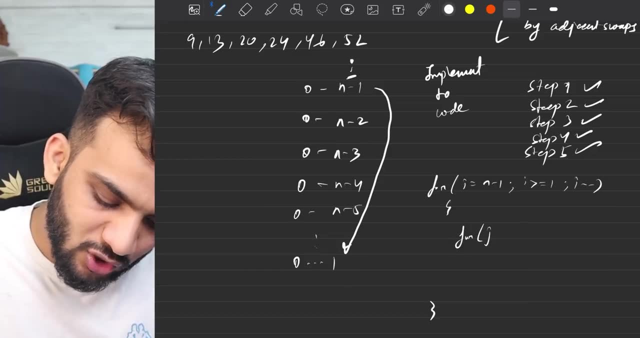 equal to n minus 1, I greater than 1 and I minus 1.. This is what I have And internally I can always run the loop from J equal to 0 till J lesser than I and J plus first. Is it similar? 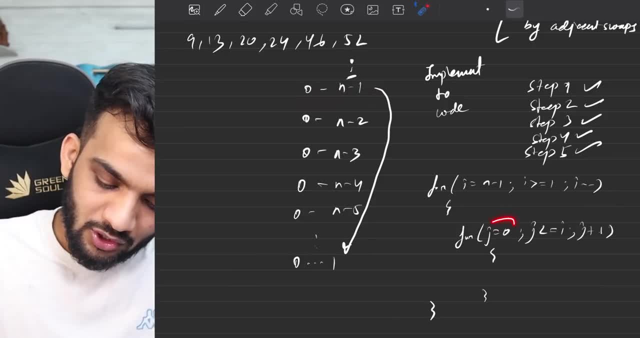 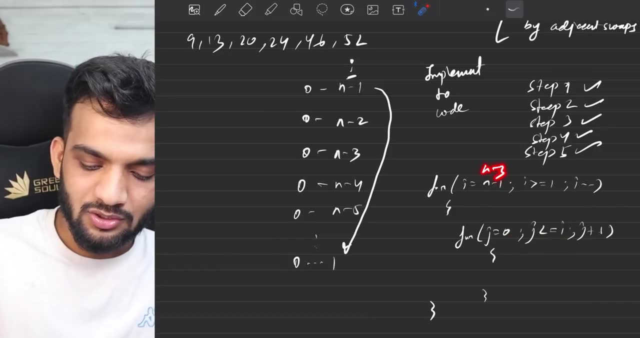 Is it similar? observe: 0 to n minus 1, 0 to n minus 1 for the first time. Next time I is n minus 2, so 0 to n minus 2. next time I is n minus 3, so 0 to n minus 3.. 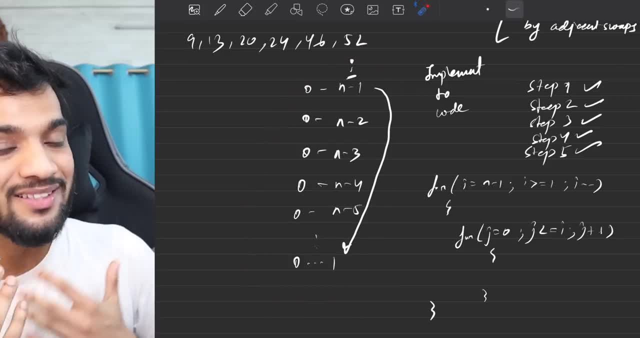 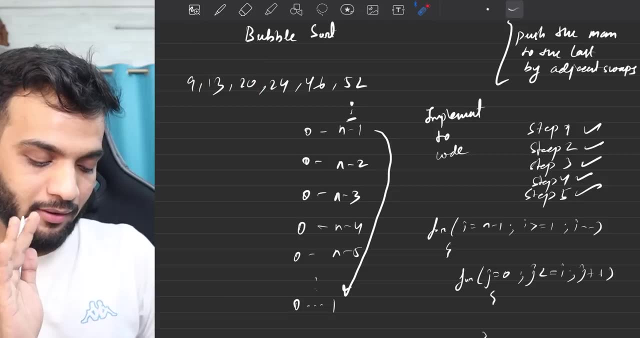 So I have made sure the looping is done. What is the next thing that you're doing? The next thing is very simple: You take up two elements and you compare. you take up two elements, you compare. So when you're looping from 0 to n minus 1, it's kind of. 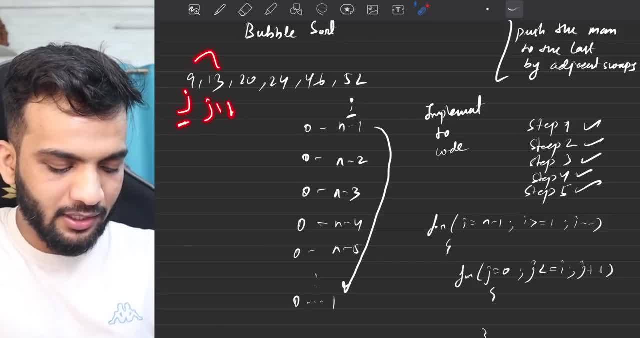 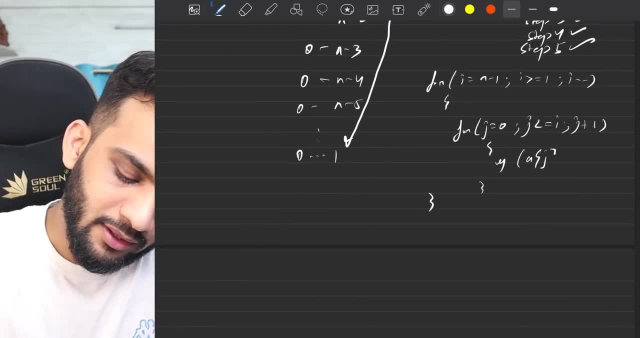 This is J, So you're comparing J with J plus 1, and if they're not, then you're swept Right. So you're kind of comparing. You're comparing If a of J is kind of greater than J plus 1.. 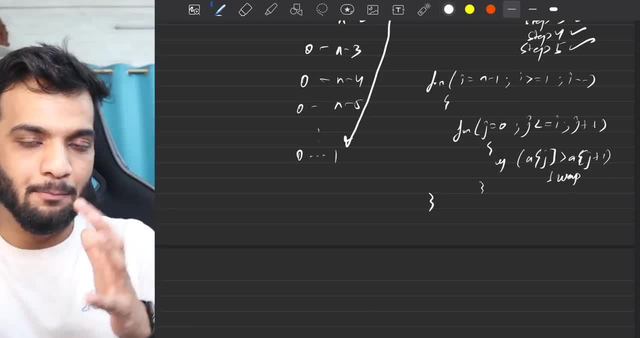 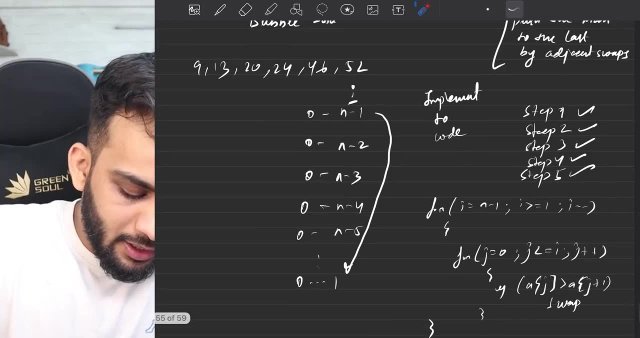 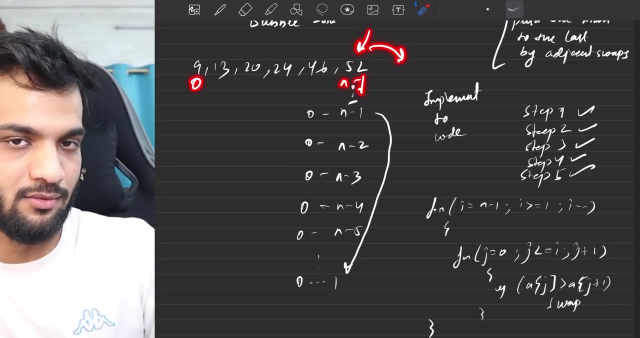 It's not in the correct order, Then you're saying swap, Then you're saying swap, both of them. A key thing to notice away, a very key, important thing: If you are going from here to here, That is wrong, because of 52, it will have no one to compare with. 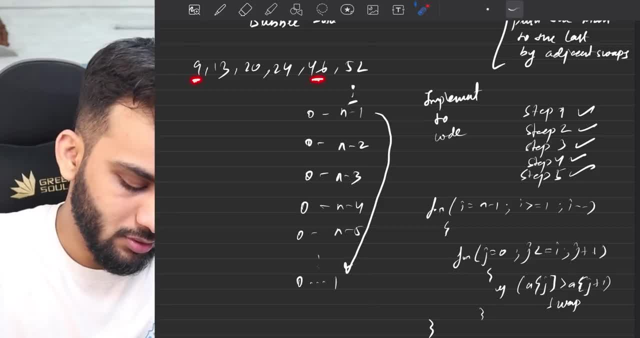 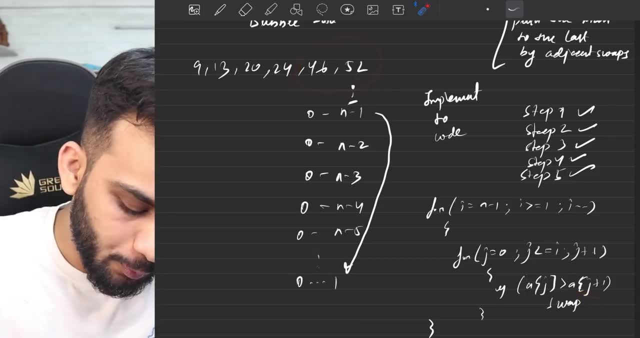 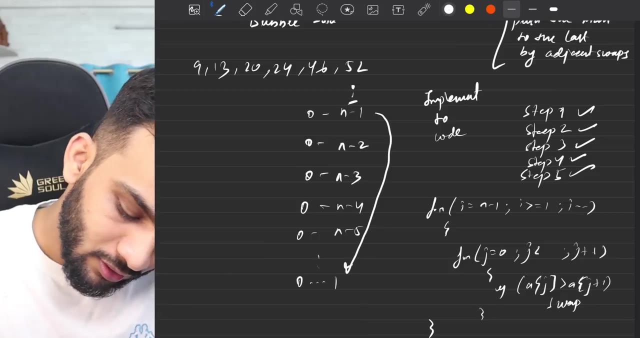 You actually go from here to here Because of 46. Gets compared with J plus 1, which is this: Do you actually look till here? So what you can do is You can go over here and say, instead of going till I, exactly, I will go till I minus 1, because if I go till here, 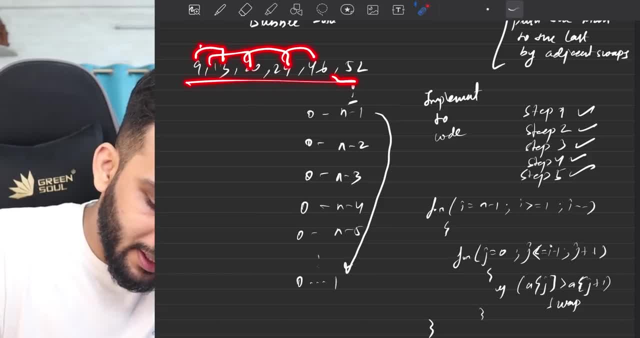 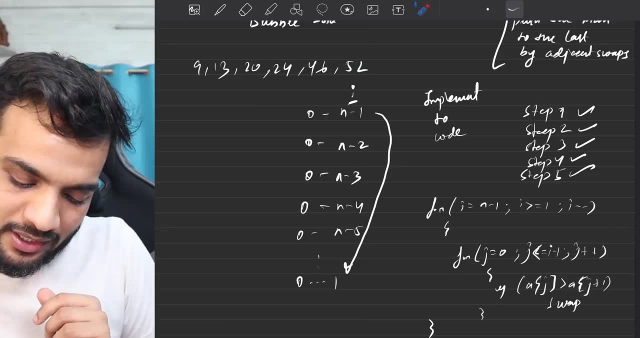 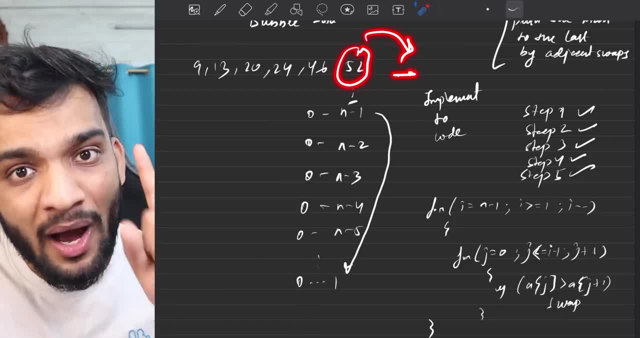 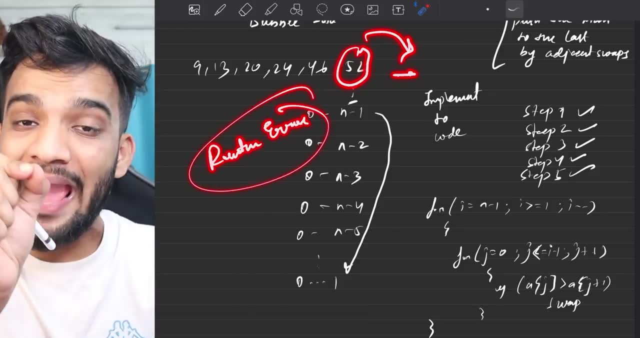 look for the next index which is not present, and if you are accessing an index which is not present, it will throw a runtime error. Remember this: if you are accessing an index which is not present, it will say runtime. I did not, It's a runtime. 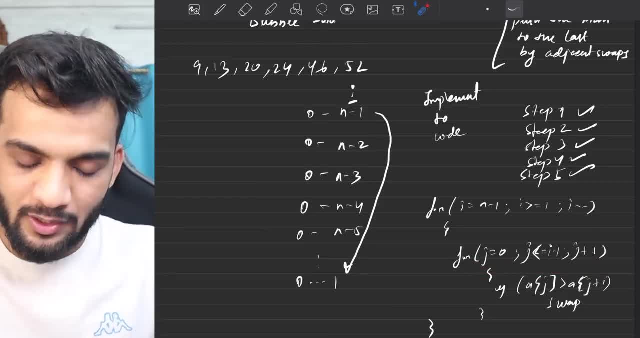 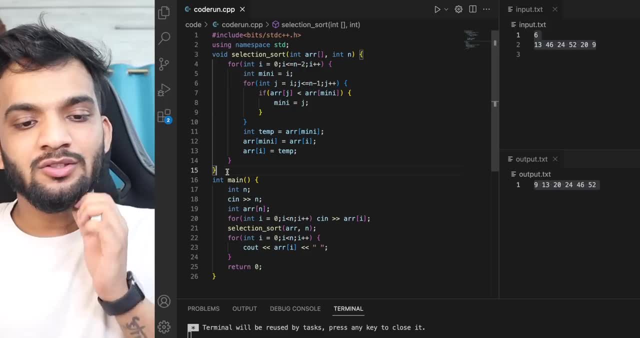 That's why it's very important to run your loops perfectly. That's when you stop, and once you have done this, All steps at the end of the day that they will be sorted. So what we will do is now you write void bubble, sort, and we'll do the same. 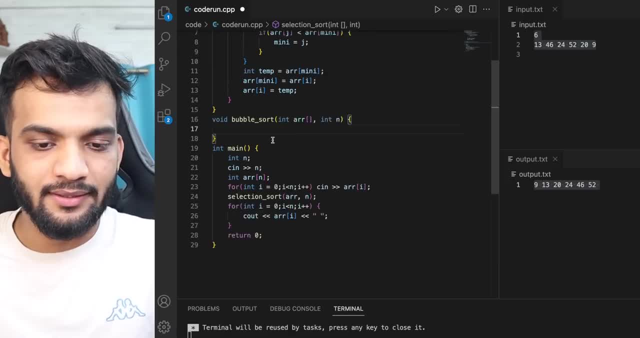 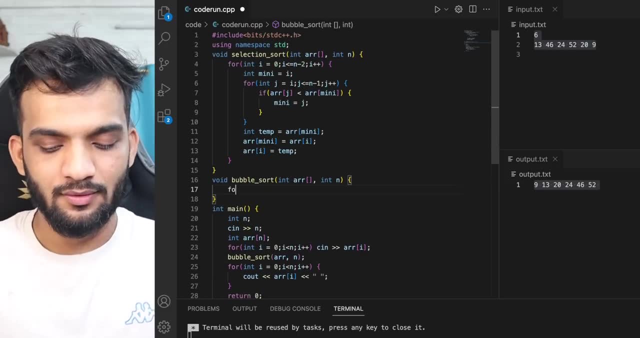 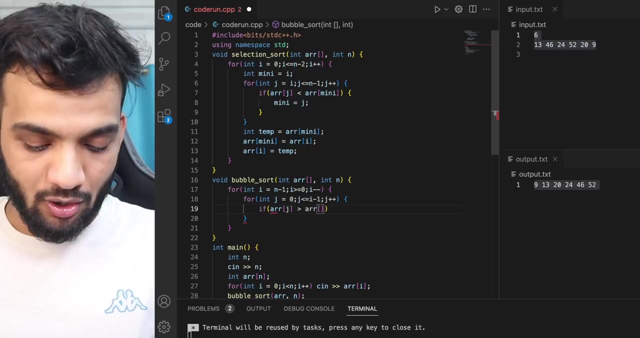 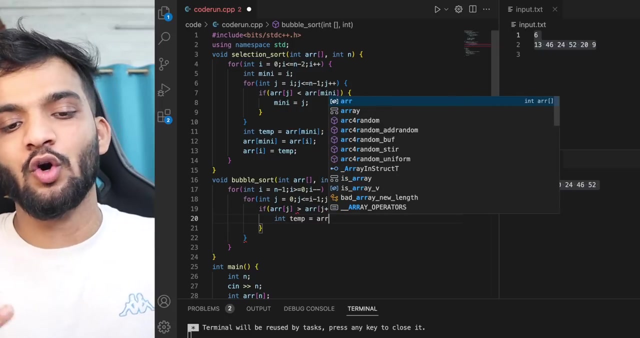 thing: Array and n, and instead of calling the selection sort, we will say a bubble chip. So I will just quickly go and write the same pseudocode. If you remember, this was kind of array of J. if greater than array of J plus one, then you stop. and in order to stop, I've already taught you how to do. 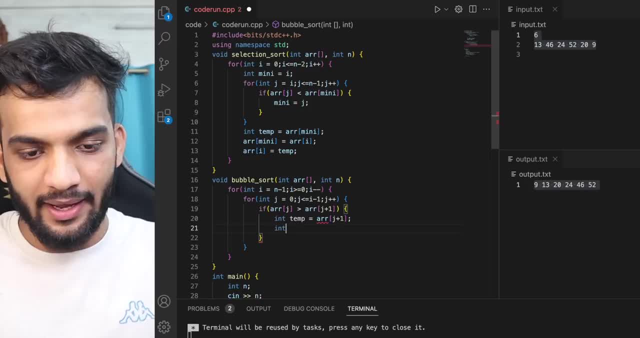 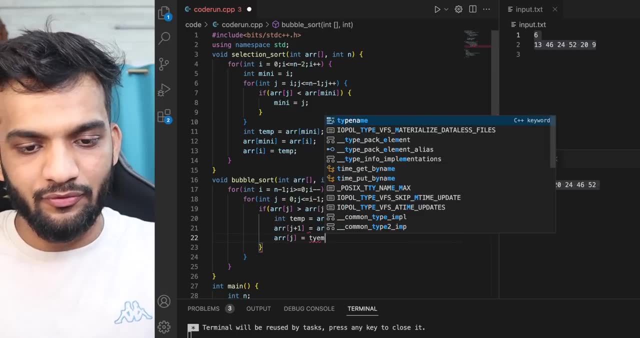 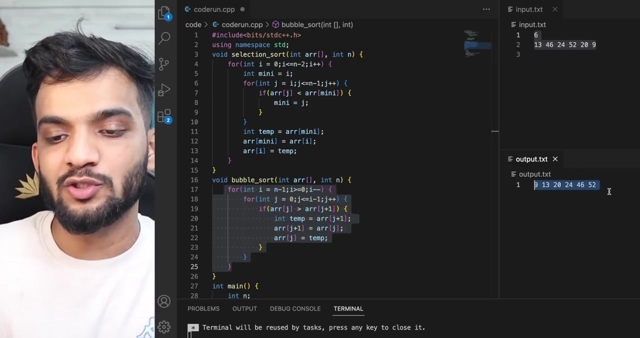 that shopping. you do this and then you say, okay, array of J plus one can use to array of J, and in array of J Can you take the value of the array of J, which is J plus one, which is stored in temporary. once you have done this entire thing, the array will be sorted. 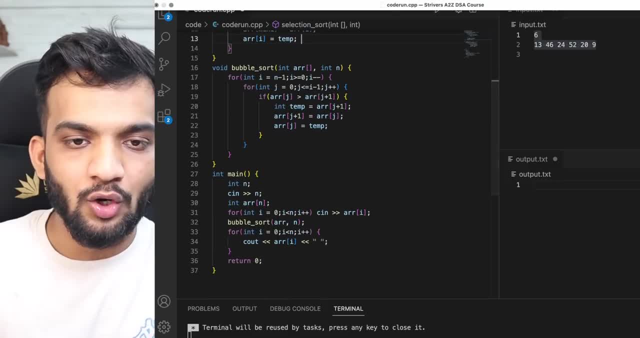 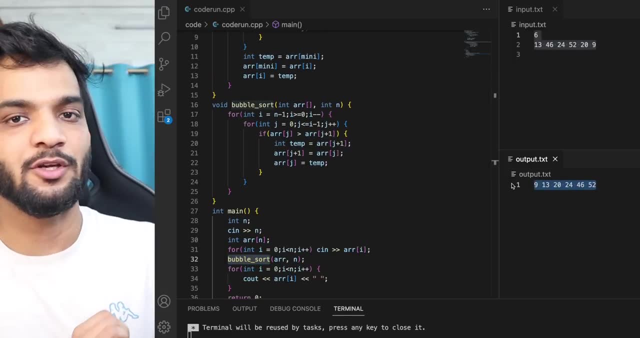 I'll just go and erase this output dot txt and now go across and say To run it and see if the bubble shot is actually producing it. it is, it is producing. So if I have to analyze the time complexity, can you analyze the time? 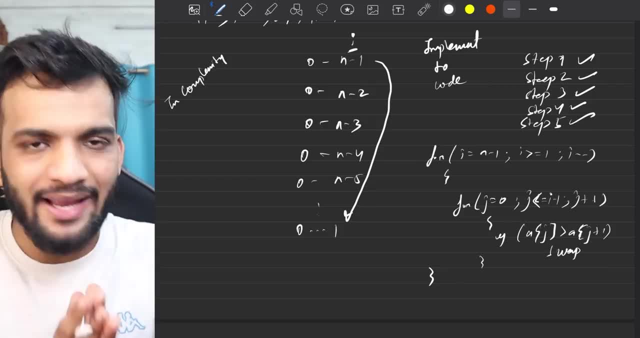 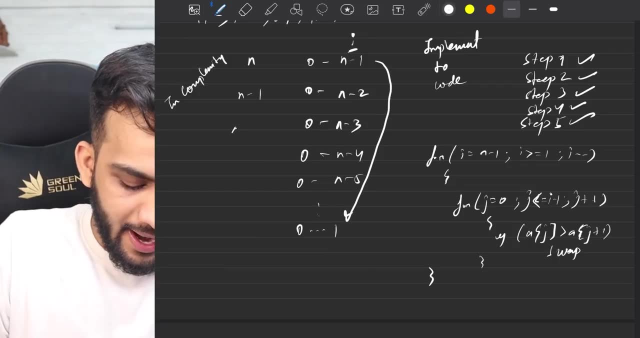 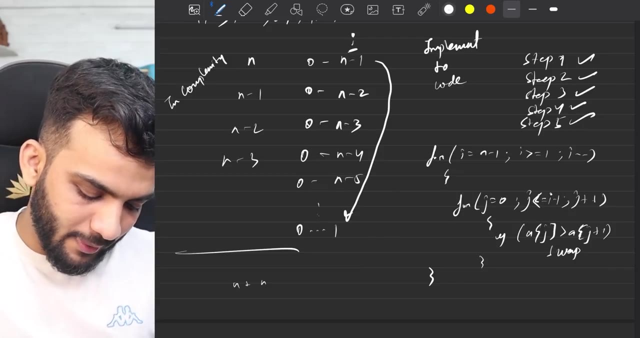 complexity for me for this particular case is quite similar to the selection sort. first time. the algorithm kind of runs for n, then for n minus one, then for n minus two, then for n minus three. So it's similar to selection sort where I say it's n plus n minus one. 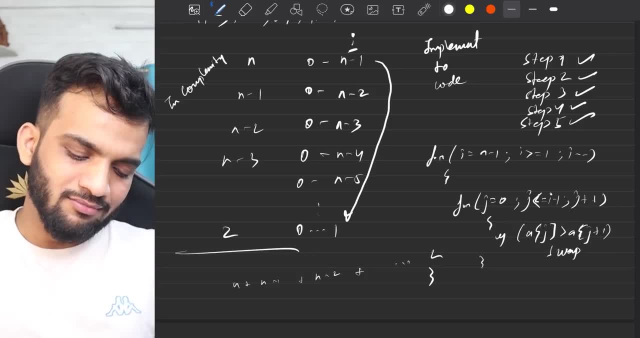 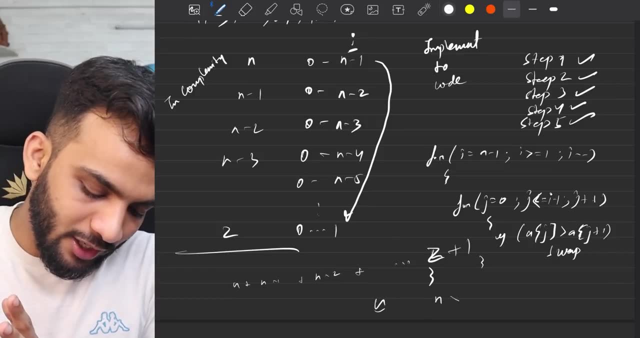 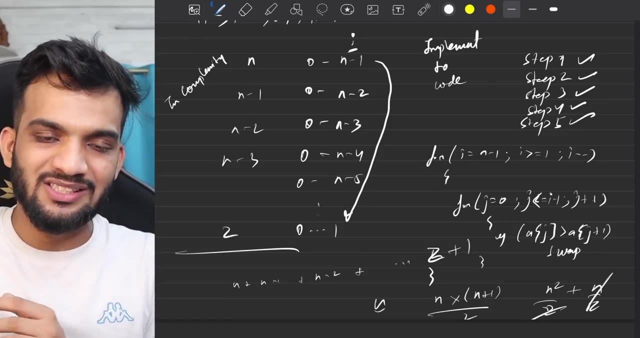 plus n minus two plus so on the last is two, It's something if you just add a one to it. it's similar to sum of n natural numbers. again, n into n plus one by two, which is n squared by two plus n by two smaller constants dissolved. 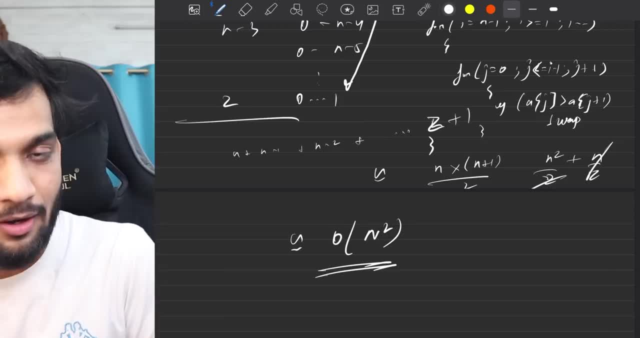 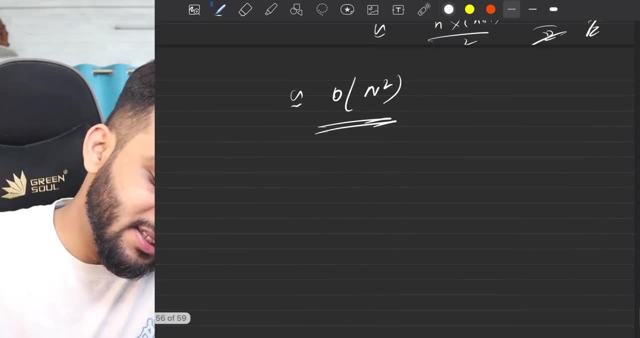 So the complexity is bigo of n squared. Can it be optimized? That's my guess. It can be. it can be optimized. This is the worst complexity. This is the worst complexity and you can also call it as the average complexity in most of the cases. 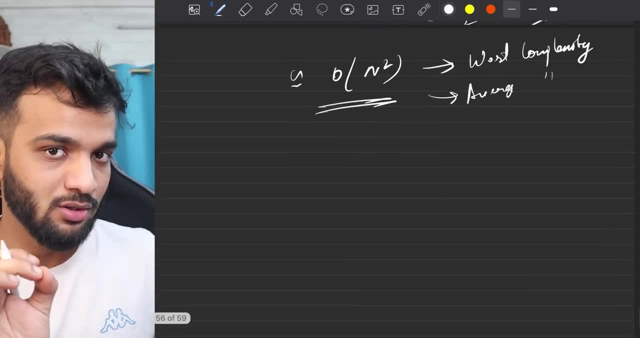 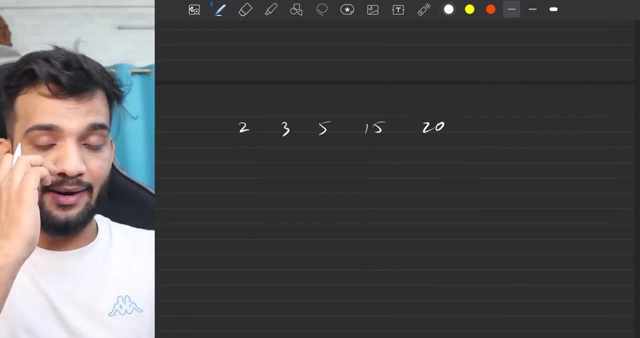 This will be the common most of the cases. but imagine if I give you an array which is something like two, three, five, fifteen and twenty. if I give you an array length, You'll be like Trevor, This is sorted. Yeah, it is sorted. 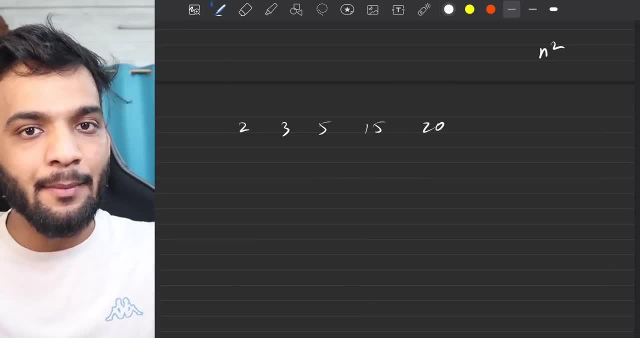 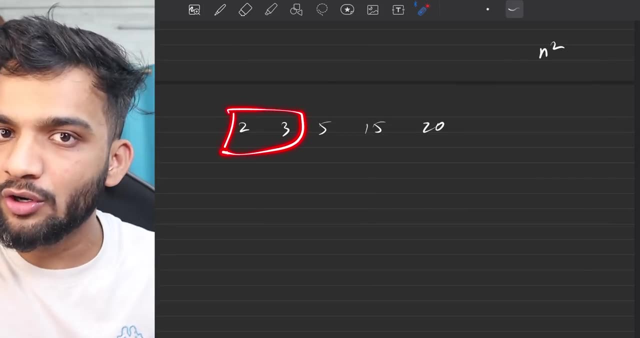 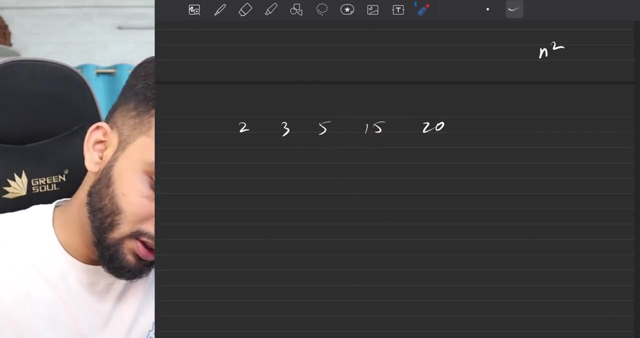 So do you run the loop for n squared? Do you go across every time, every day? No, So what is the algorithm? Correct order- No swaps. Correct order- No swaps. Correct order- No swaps. Correct order- No swap. Arre, dude, if everything is in the correct order and you're not performing, 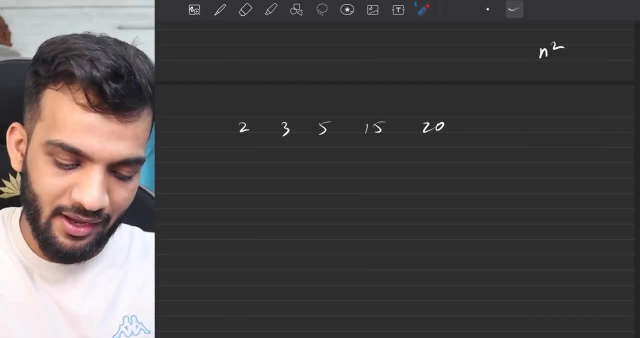 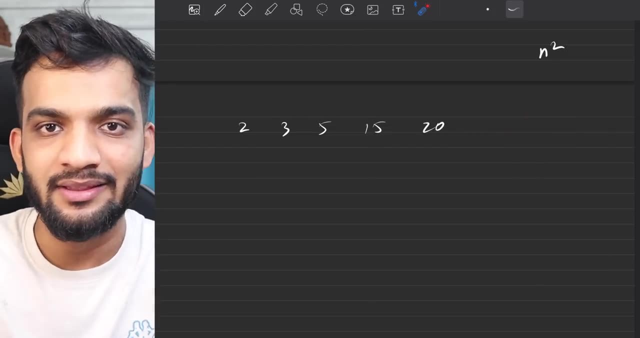 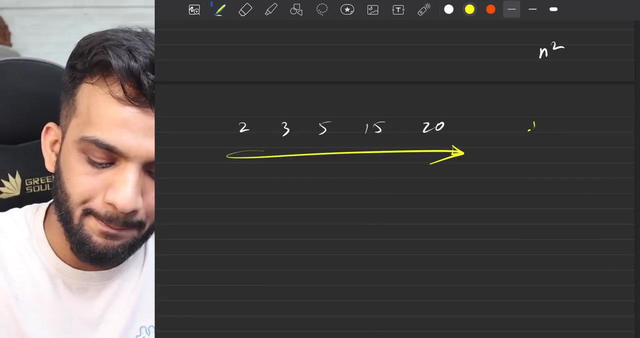 a swap. if everything is in the correct order, what does it signify? The array is in the ascending order. If everything is in the correct order, The array is in the ascending order. so in the first check you did not find a swap to be done because everything was in the correct. 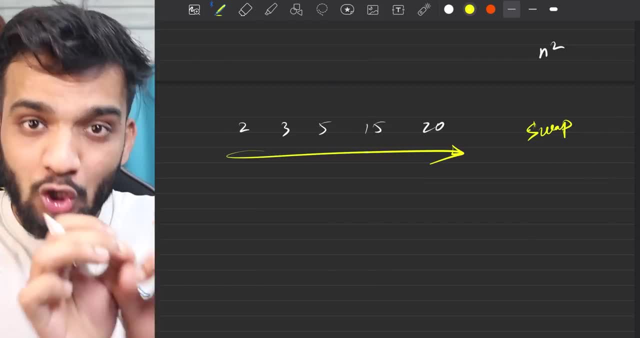 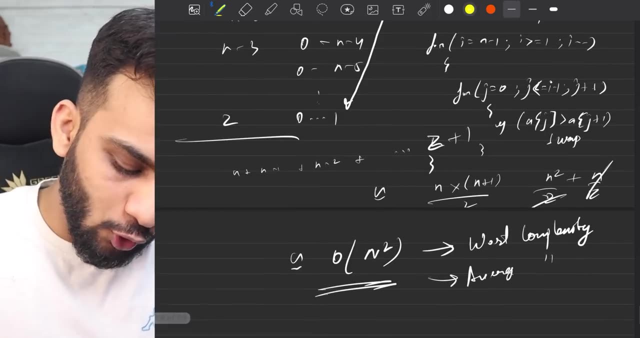 order. so can i say: if i do not do any swaps, if i do not do any swaps, that's when i stop, i do not. so it's kind of: if no swaps done, i don't need to go. if on the first check no swap is done, i don't. 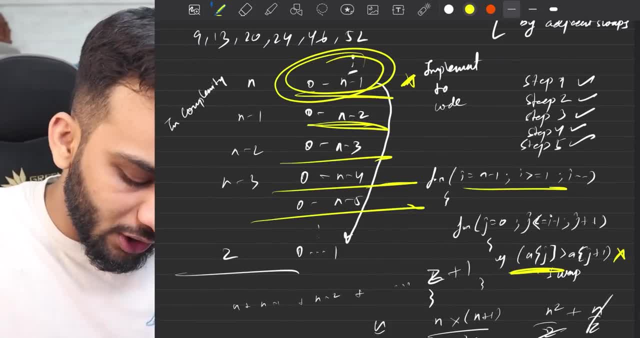 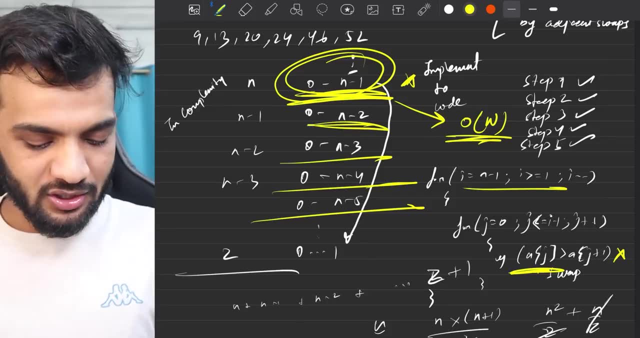 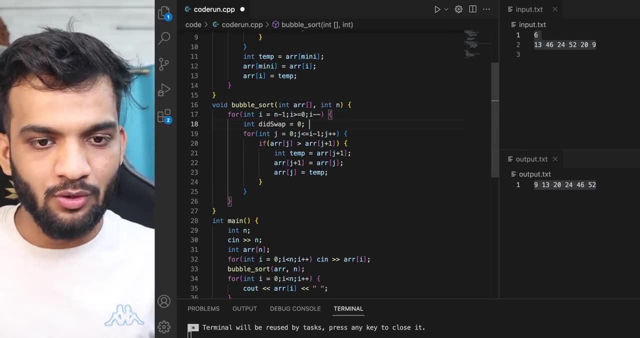 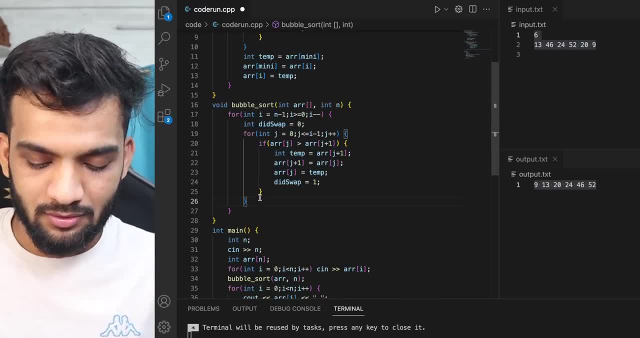 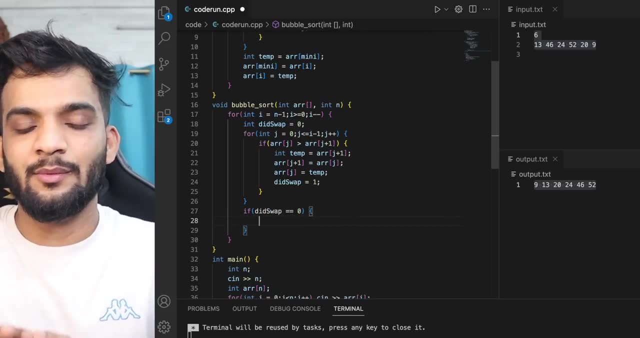 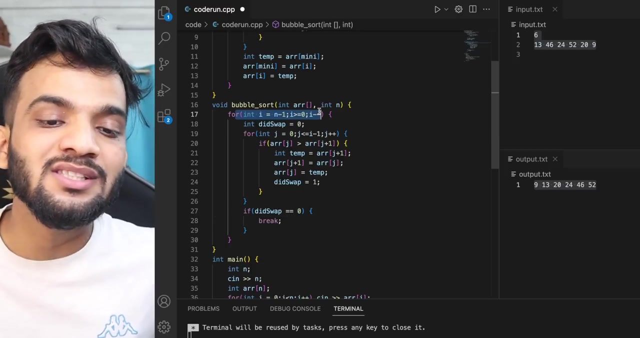 if at any moment a swap happened, then it's okay. but if you you did swap at any time is there was no swap, then i break out. i will not go. if the array is sorted, it will just check for the first time and it will break. post it. right. this also runs. 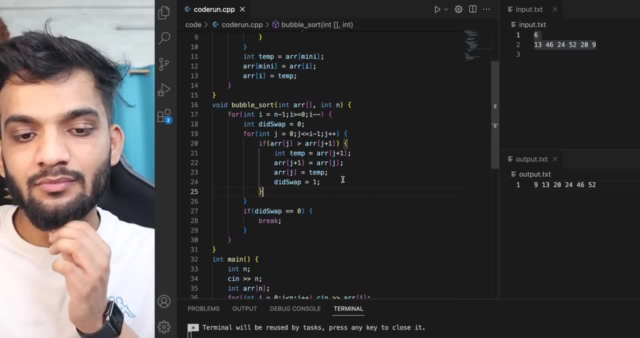 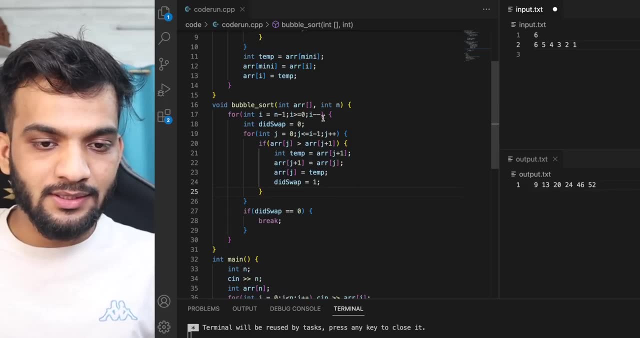 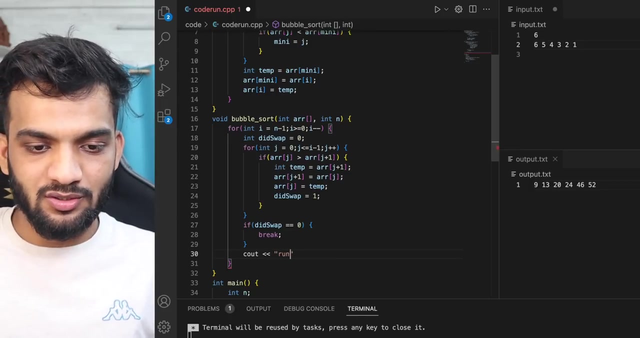 i'll prove you, uh, this one. i'll prove you this one. so i'll give you an example: see six, five, four, three, two, one. now what i'll do is i will just go ahead and and print this how many times the array runs- okay, and runs, and i'll just give it and you can see how many times it runs now. 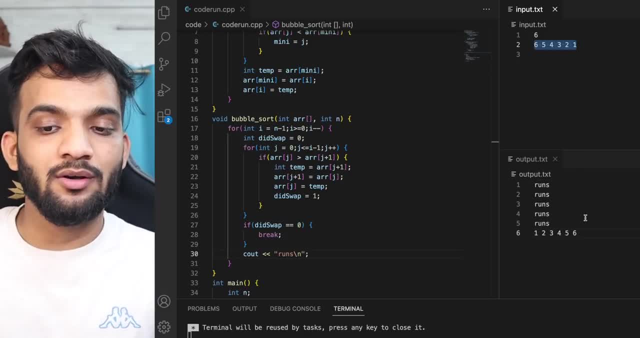 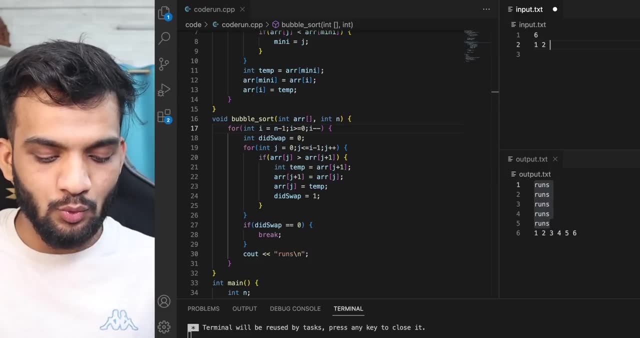 terminal and i'll go to run task. this is a descending order and it runs for five times. because the size is six, it runs for five. but if i just change it to something like one, two, three, four, five, six and i'll see how many times the first for loop just see. 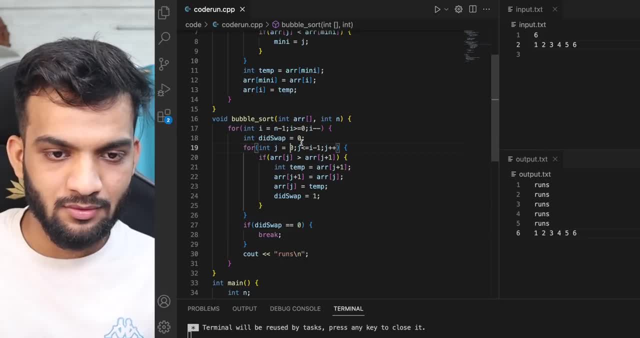 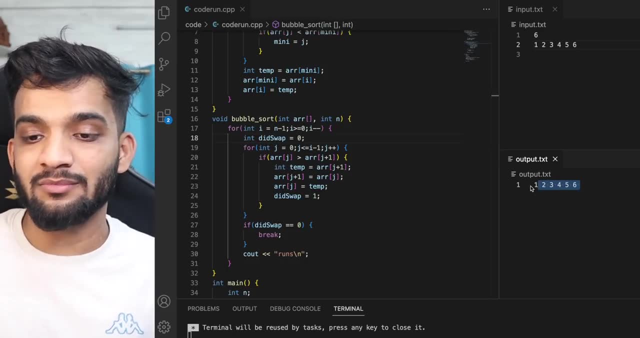 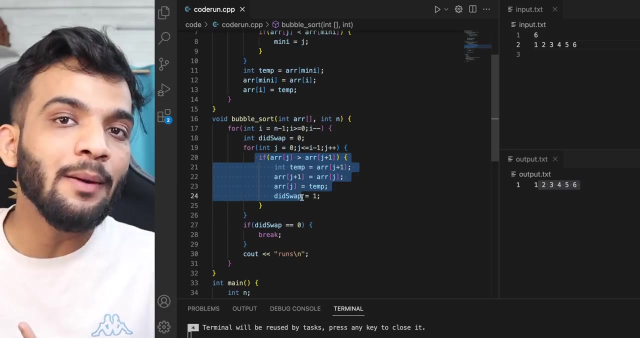 uh, did it run just a minute? that's one, two. okay, let's run it. run it. did you see something? it never came to this because it it did break over here, so it just ran for the first, did not swap and broke. so can i say, can i say the best time, complexity. 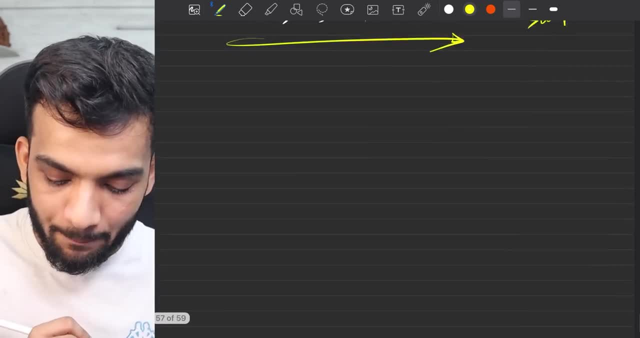 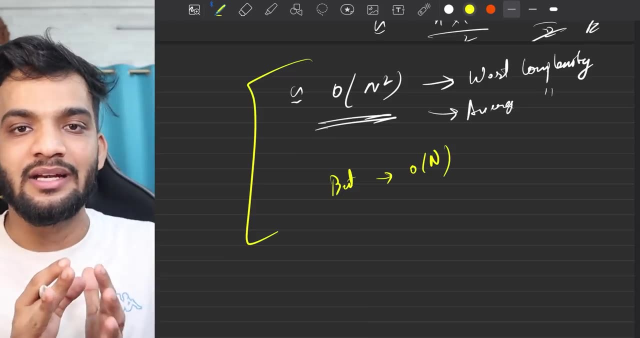 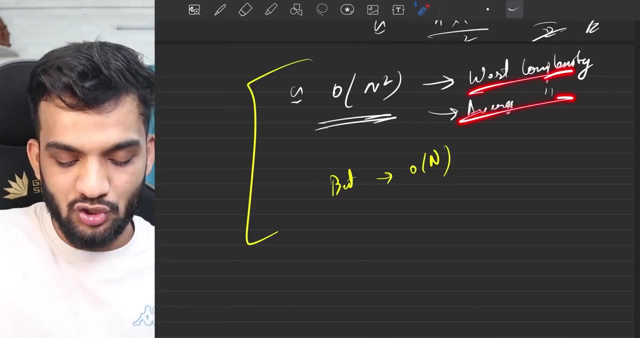 will be nothing but big go of n for the time, complexity for the best of the time. complexity of bubble shot is we go often this might be asked in an interview. you have to critically tell them the use case. you have to explain them in the dry run and tell them the worst and the average might. 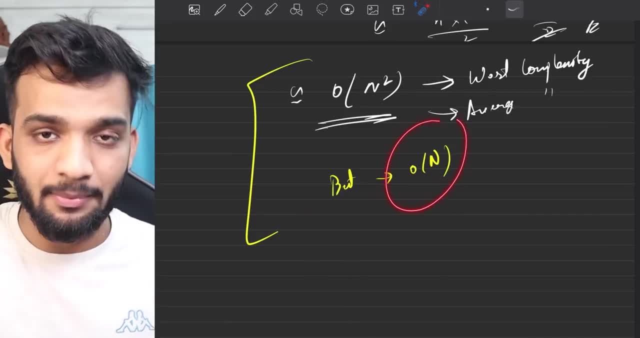 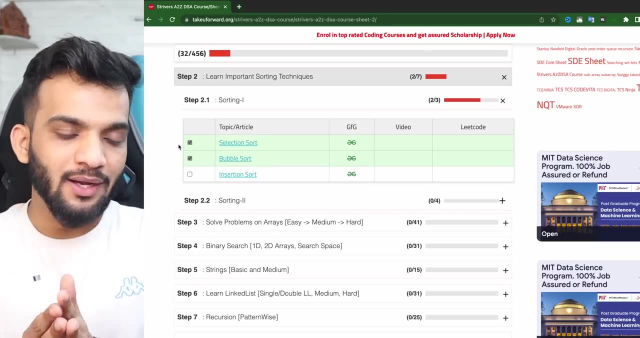 be n square, but if the array is sorted, i will break out and i'll end up getting a linear time complexity because the array is already so. so the bubble shot is done. now let's move on to the next one, that is, the insertion sort algorithm. so, talking about insertion sort, you need to remember 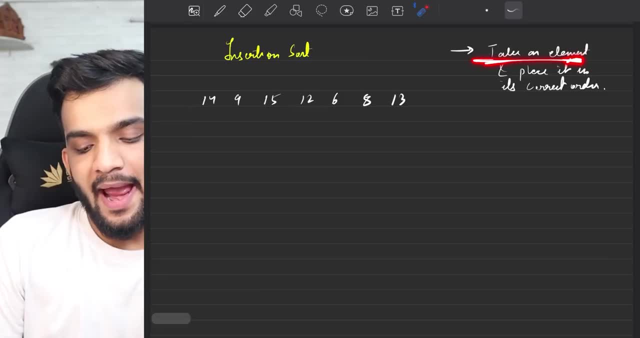 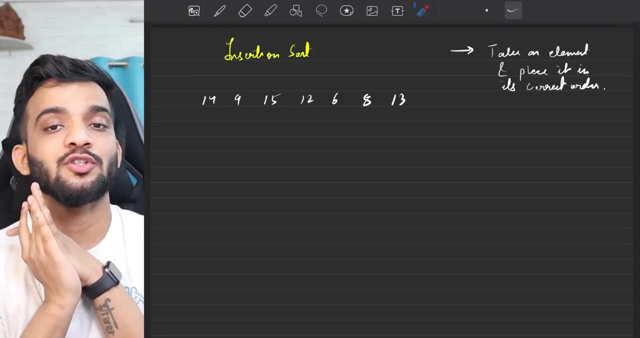 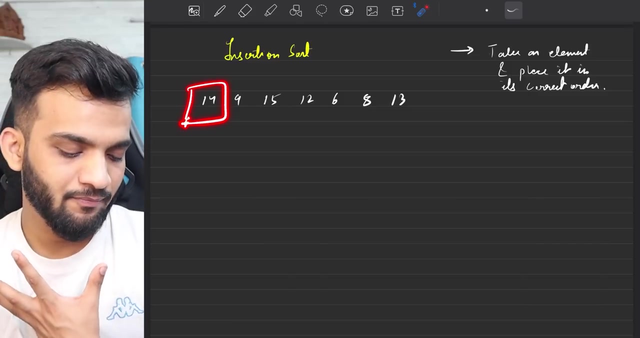 one thing: it always takes an element and places it in its correct position. takes an element and places it in its correct position. let's start. yeah, the algorithm starts with looking at the first element as an array and you will say that if this much is the array, the element 14. 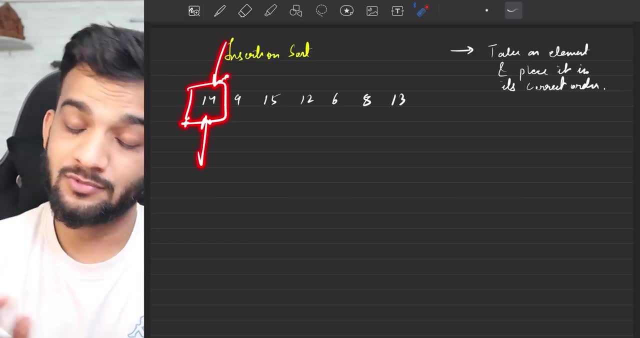 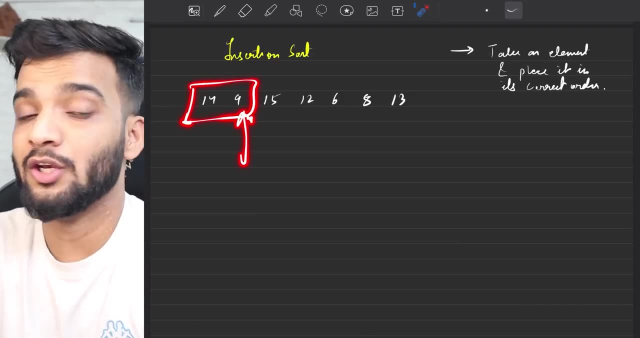 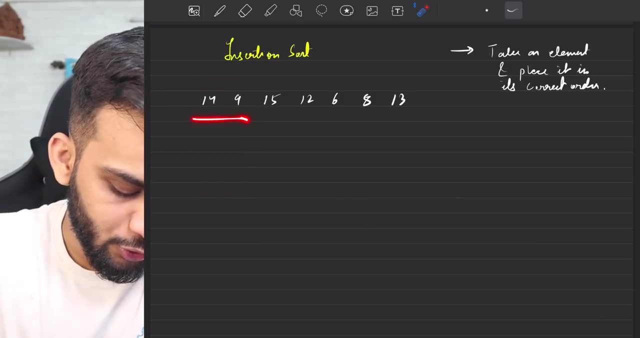 in a size, one array is at the correct. if i look at this much and and i ask you, is 9 at the correct position? you'll be like: no, 9 apparently should have been here and 14 should have been here. so this is what you do. you go to the next element and you ask on the 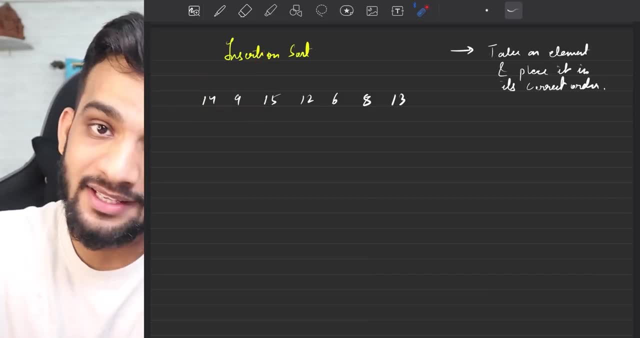 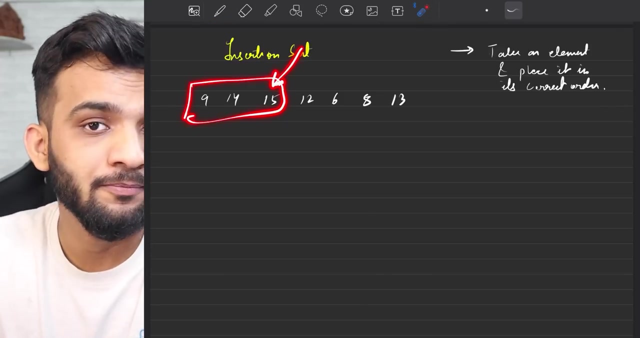 left side where 9 should have been and that is where you take. so you basically do it like this: 9, 14, perfect. so then you go ahead to this one and you ask: is 15 at the correct position for a size three? and you say: then you go ahead and say is 12 at the correct position? 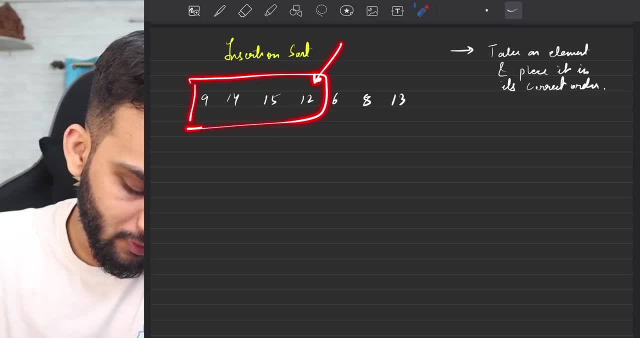 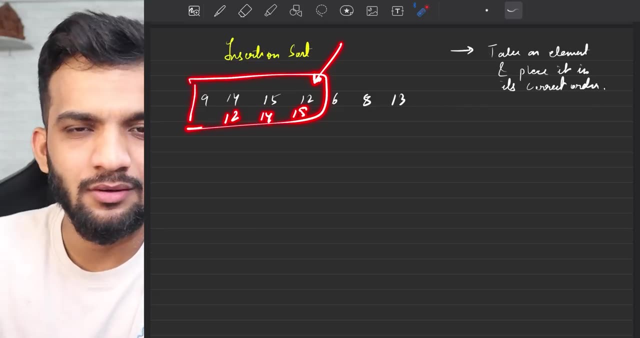 for a size four and you say: no, apparently 12 should have been here, 14 should have been here, 15 should have been. so do you see a pattern? it's like 14 will come here and 15 will come. everyone right shifts by one and 12 kind of goes in its correct model. so what you can do is 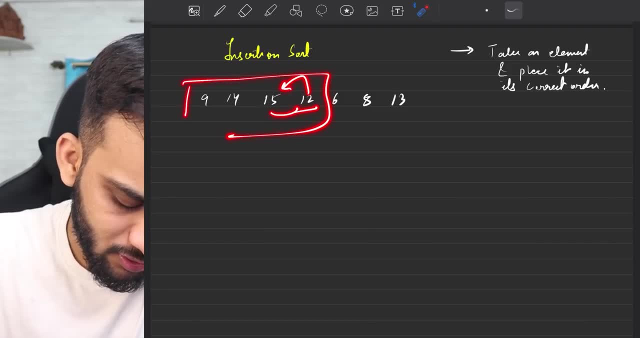 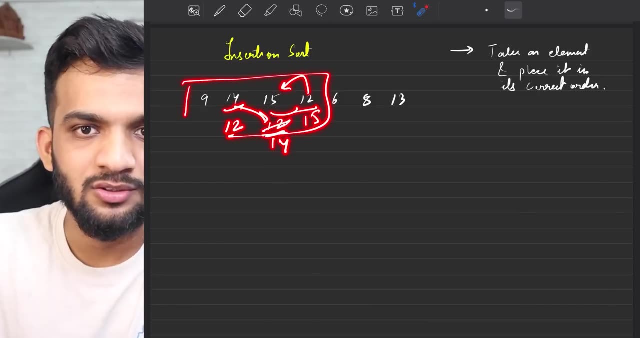 you can take 12 and you can say, okay, 12, 15, 15 will come here, 12 will go here. then you can say 12, 14. so you can 12 here and you can pass 14 here. you can go to the left and swap, swap, swap till it can. 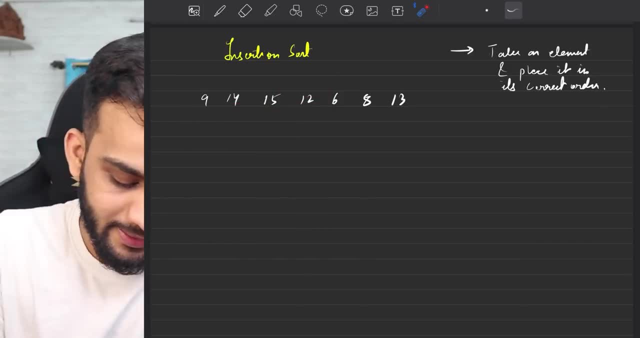 be swapped till it can be swapped. so if you do like this, 12 goes here, it's like 12 and 15, then 12, 14. so 12 goes here and 14 come. so go to the left till it can be. can 12 be swapped with 9? no, because 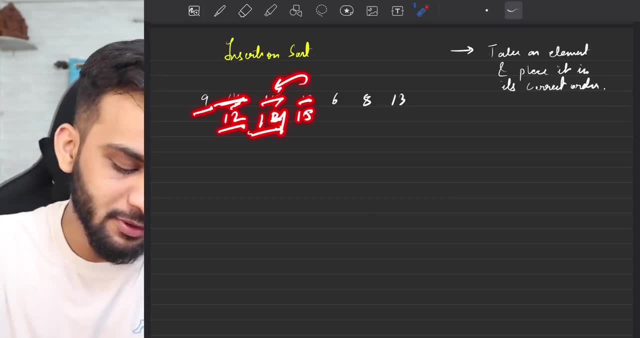 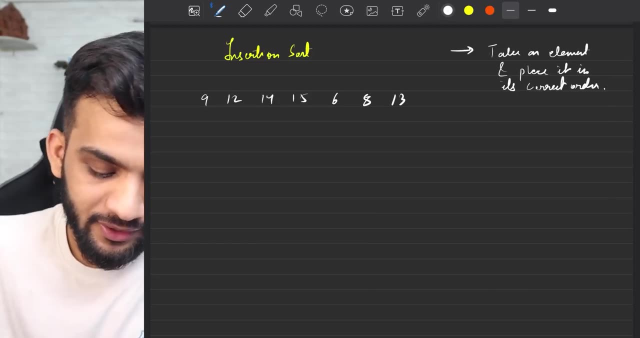 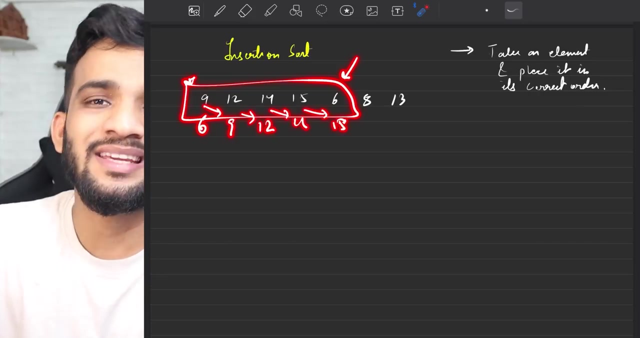 that will distort the order. it just goes till here, simple. so what will happen? it'll be like 12, 14, 15, perfect. next is 6. if we look at 6, where ideally should be 6 in this array, it should be here, 9 should be here, 12 should be here, 14 should be here, 15 should be here. so can i do this, can i? 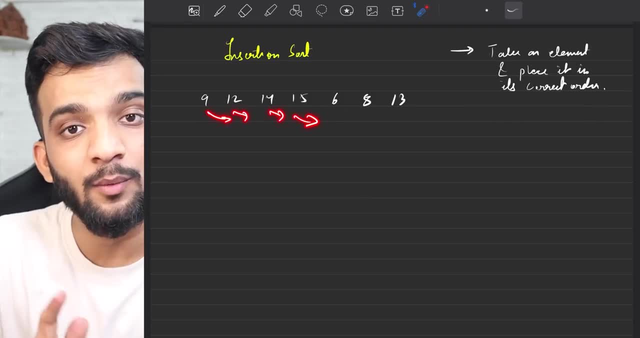 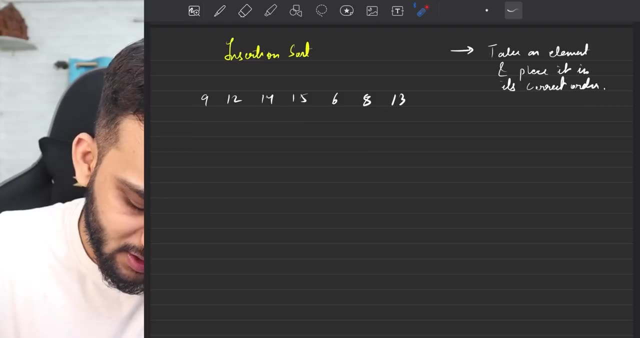 take the 6 here. but i have to. i have to right shift every one by one. how do you do it? you take 6, you take 15 and you say, okay, swap yourself. what happens is: 6 goes here, 15 goes here, swept. next you take 6, 14, 14 comes here and 6 goes here. next you take 6, 12, 12 comes here, 6 goes. 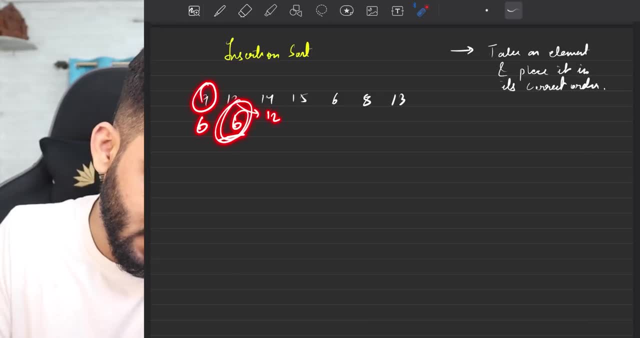 here. next you take 6 and 9. 6 goes here, 9 comes here. so if i have to do it, it's like 6, 12, 15, not in the correct order. let's swap it: 15 comes here and 6 goes here. 14: 6: no, 6 comes here. 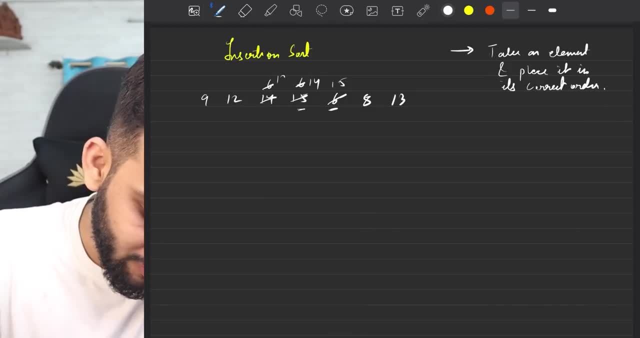 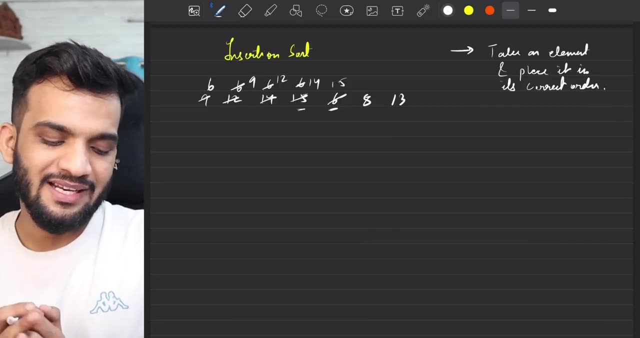 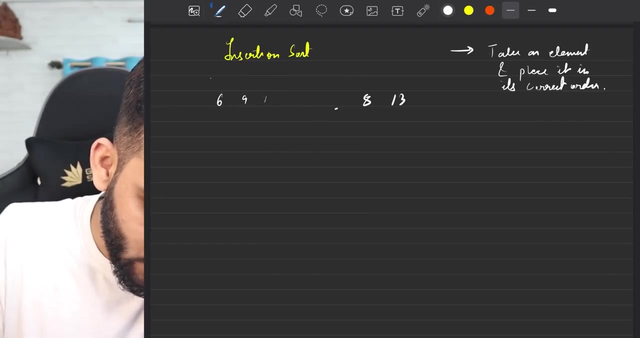 14 goes 6, 12, no, 12 comes here. 6 goes 6, 9, no. 9 comes here, 6 goes, perfect. it's like 6, 9, 12, 14, 15. so if i have to write it by raising, it's like 6, 9, 12, 14, 15, perfect. i just went on to the left. 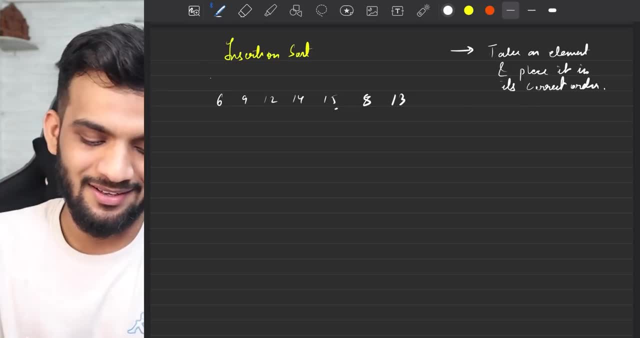 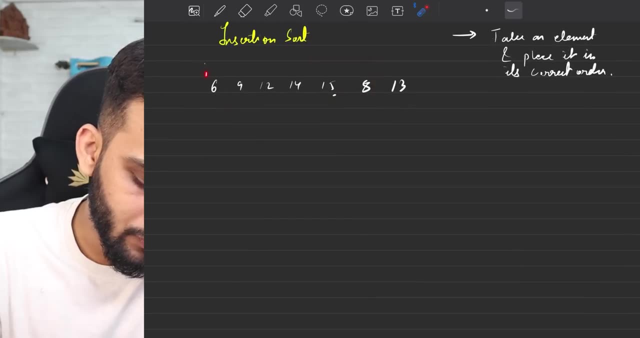 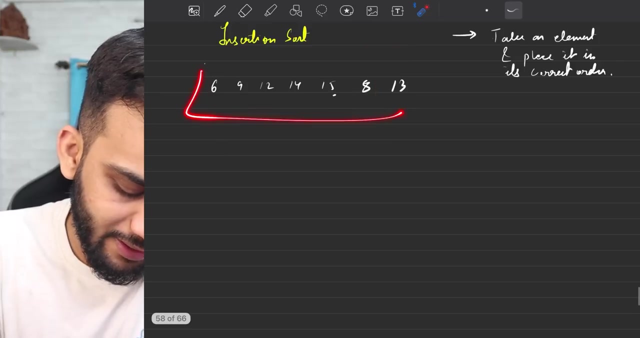 till it could have been swap, swap, swap. right next, 8 in this particular array. where does 8 will go? where will 8 go in this particular array? where will 8 go, ask yourself. the answer to that is: 8 will go here. so if 8 has to go here, 9 has to go here. 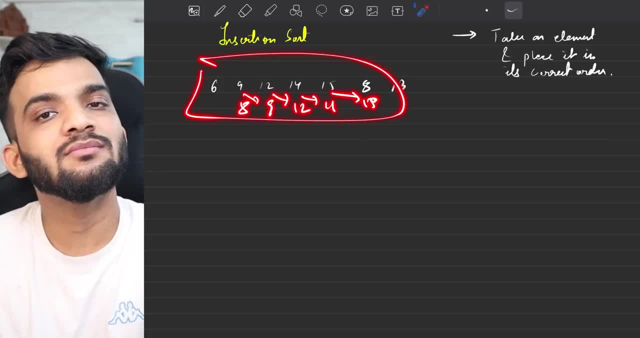 12 has to go here. so if 8 has to go here, 9 has to go here, 12 has to go here. so if 8 has to go here, 12 has to go here, 14 has to go here, 15 has to go here. so again, what do you do? 8, 15, so you say: 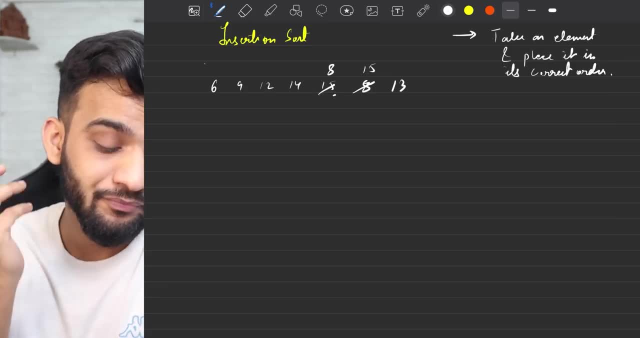 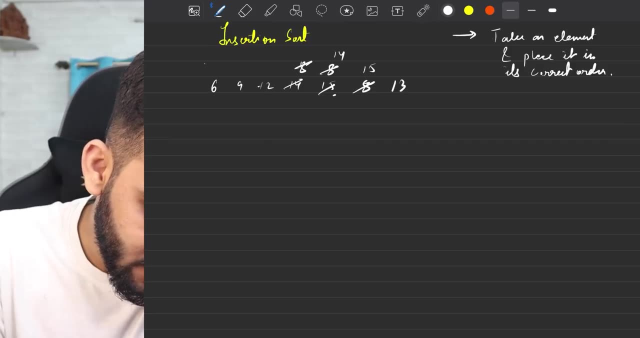 okay, 8 goes here, 15, so left can 8 14. can 8 go till 14? yes, 14 comes here. 8 goes here. can it go more left? yes, it can. 8 goes here. 12 goes here. can it go more left? yes, 9 goes here. 8 goes here. is it in? 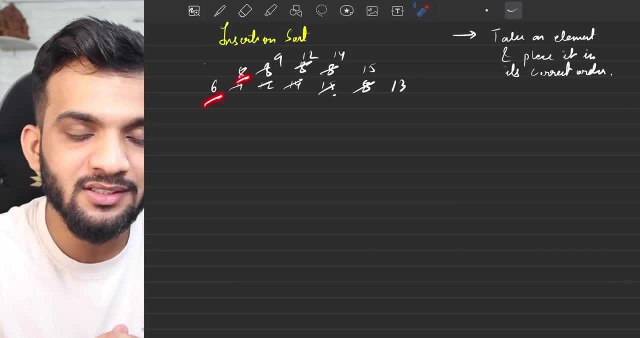 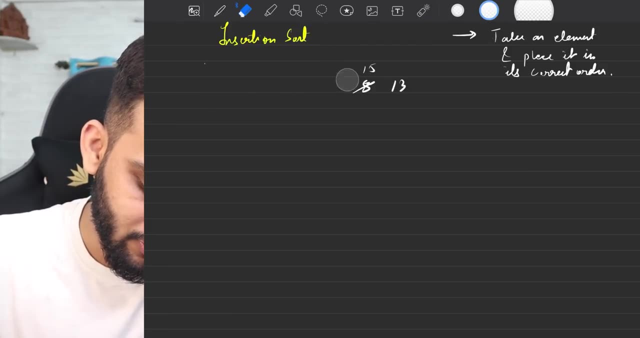 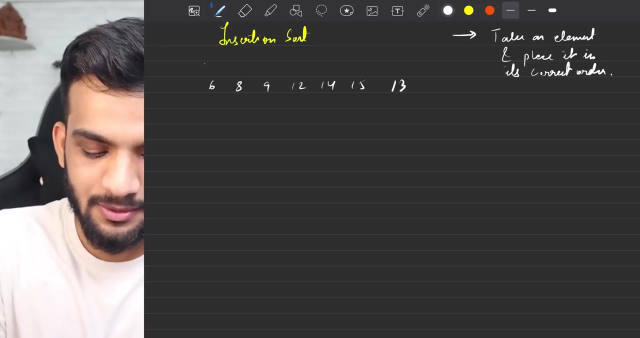 the correct order. yes, how do you know it? because when you compared 8 with 6, it was not compared done and dusted: 6, 8, 9, 12, 14, 15. 6, 8, 9, 12, 14, 15. remember this: 6, 8, 9, 12, 14, 15. next 13 is the. 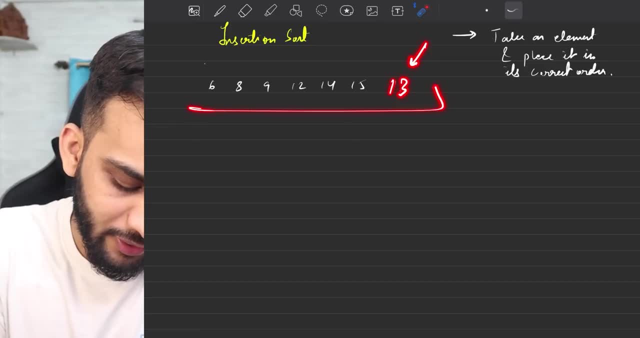 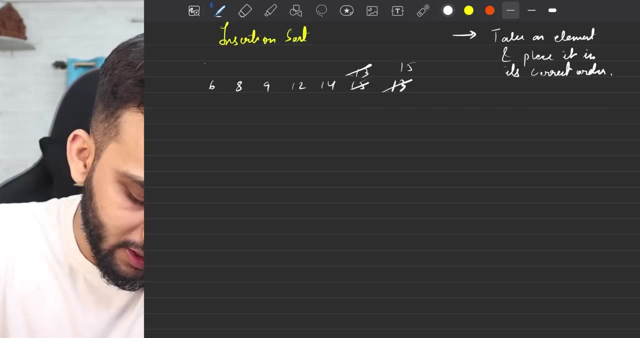 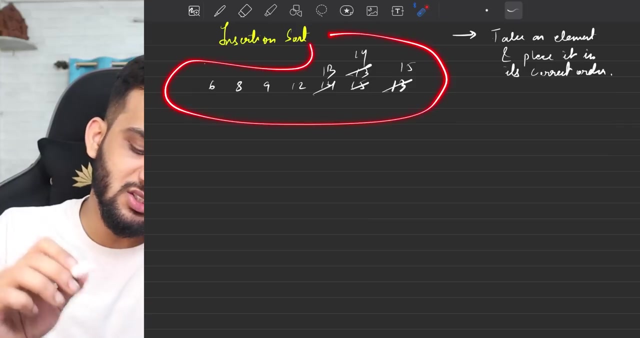 next guy that you are comparing. can i say 13? ideally over here should have been here, so do it again. 13 goes here. 15 comes here. 13 goes here. 14 comes here. can i do a 13, 12, no stop. can i say: post the last? the array is sorted. why? because you picked up every element and you did. 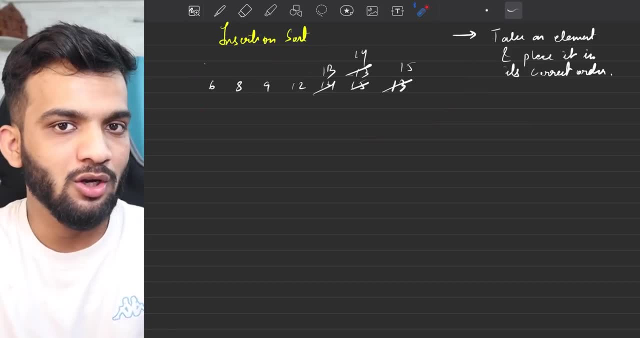 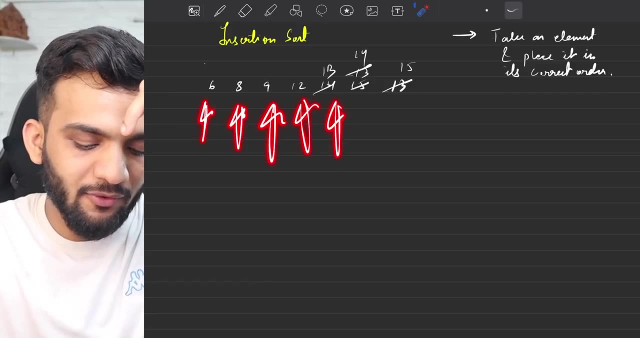 put it into its correct order. so how did it work? i picked up one first time. i picked up the first guy next time, i picked up the second next time, the third, next time, the fourth, next time, the fifth, next time, the sixth, next time, the seventh, picked up every guy. i'm running from index 0 to n minus. 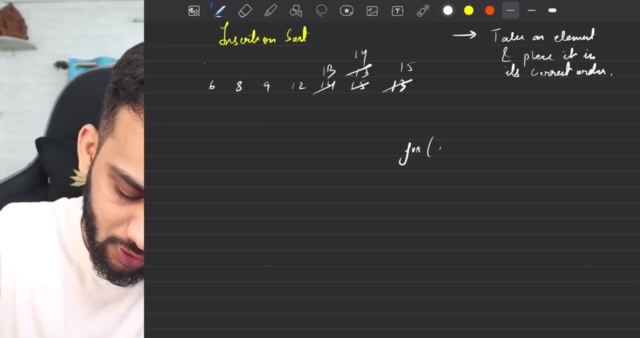 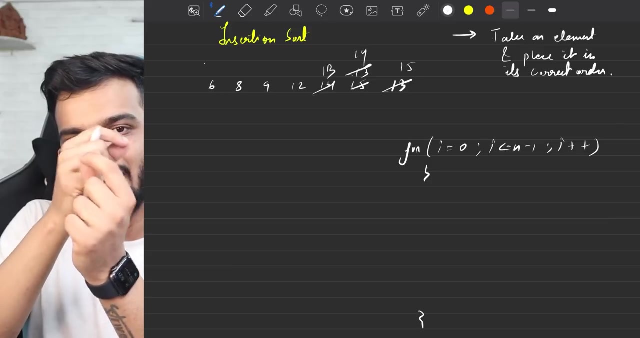 1, that's for sure. that's something for sure. i'm running from 0 to n minus 1, and what am i doing? what am i doing? every guy? i'm looking at the left. are you greater? are you greater? swap and till. i can do it like for 13. i could do till here, till it is possible. 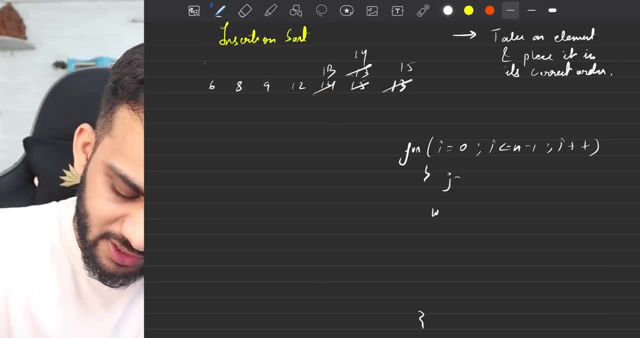 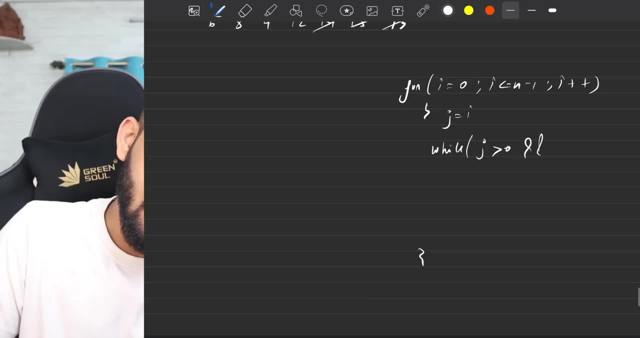 on the left. so i'll be like, okay, maybe j is i and i can keep while j greater than zero, and i can say and: and okay, hey, left j minus 1, and i can say and: and okay, hey, left j minus 1. and i can say: 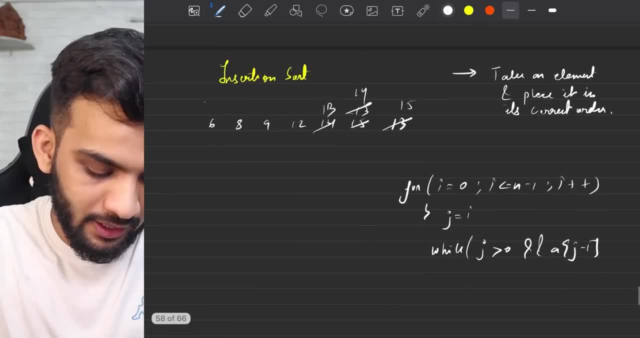 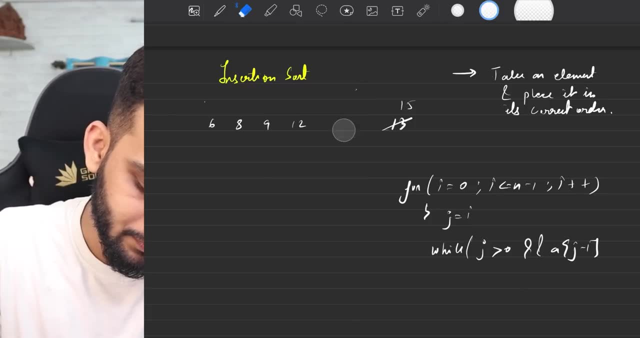 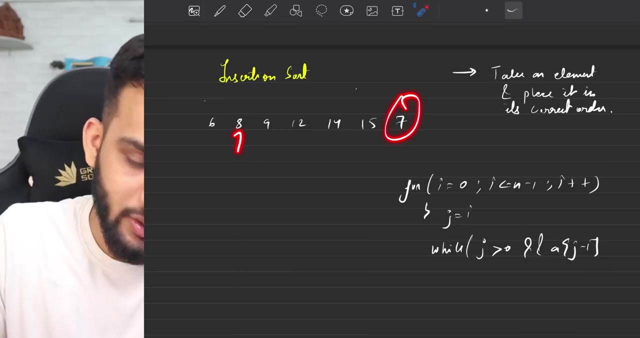 j minus 1, because the last that you can compare is still here, is still here. that's the last you can compare. so imagine this was not 13. i'll give you an example: if this was like 14, 15 and this was 7, so the 7 would have last gone here. or imagine this was 5, for an example: it was 5. 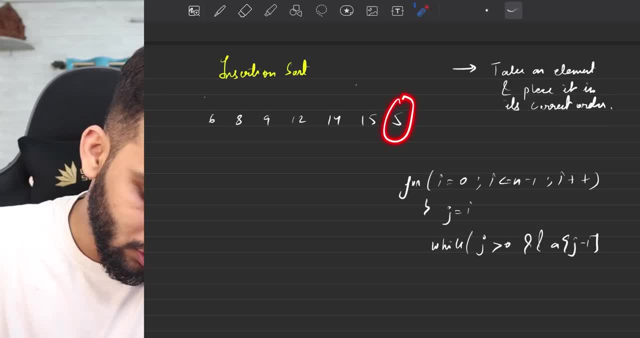 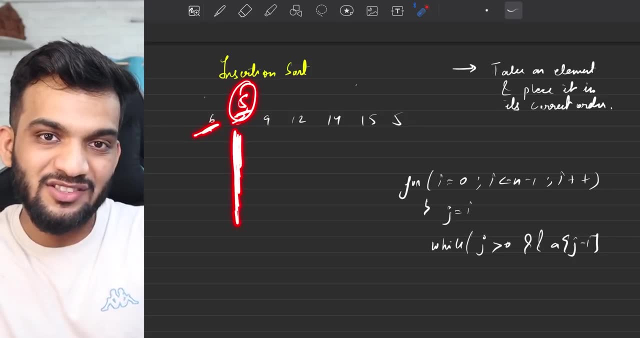 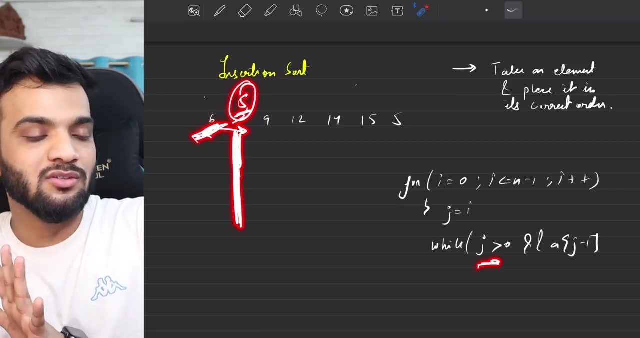 what would have happened? 5 would have gone like till here and then 5 would have got compared with 6. 5 standing here, 5 standing here would have compared it on the left. that's why you don't go till 0, because right before 0 you do the last comparison. that's why 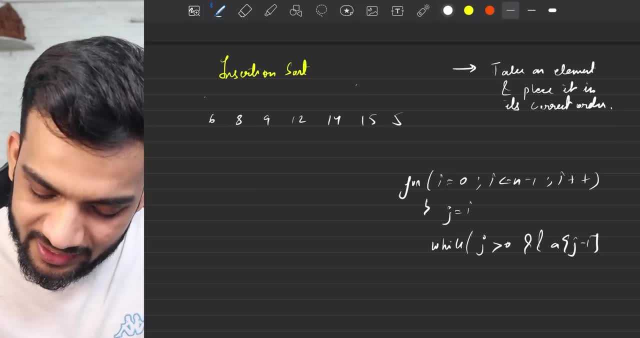 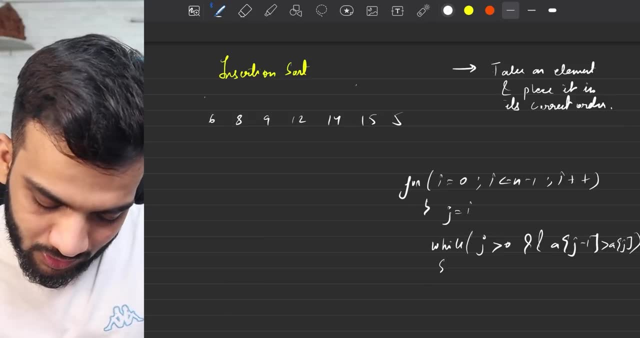 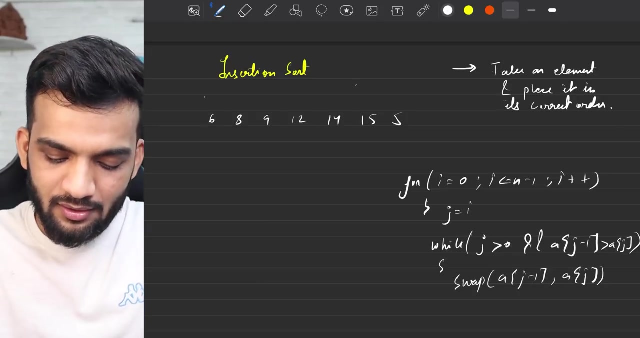 and that's why j minus 1. the last comparison: if it is greater than a of j. if it is greater, that means, can you please swap, so i'm not writing the swap. you know how to write. you say a of j minus 1 and a of j. that's what you say, right? 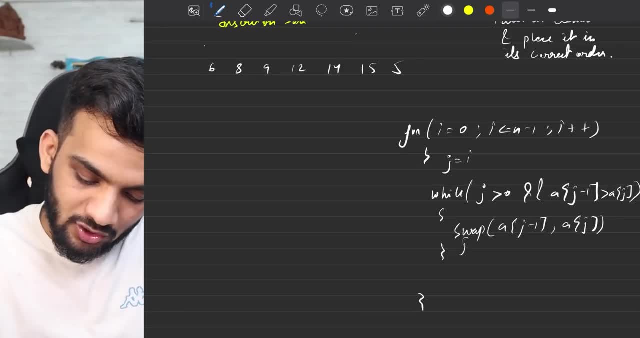 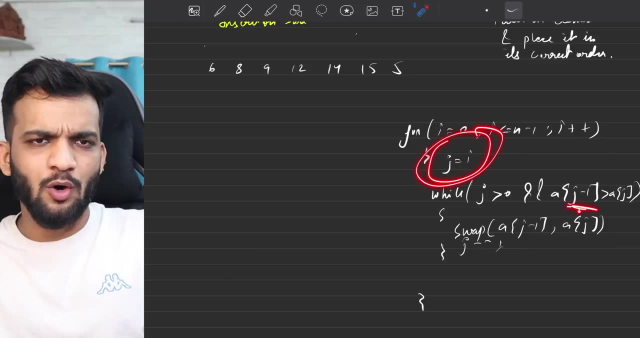 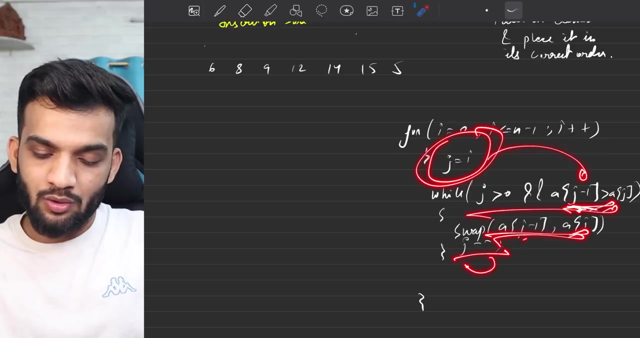 and that's when it ends and you can just do a j minus, minus over here. because what am i doing is i'm taking the element and i'm saying left short, left, small, left, small, okay, and go left again. come back, left, small again. go left, left, small, go. the moment it's not small, stop and go to the next guy. 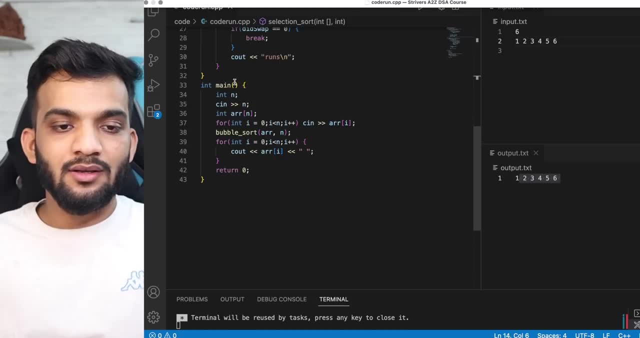 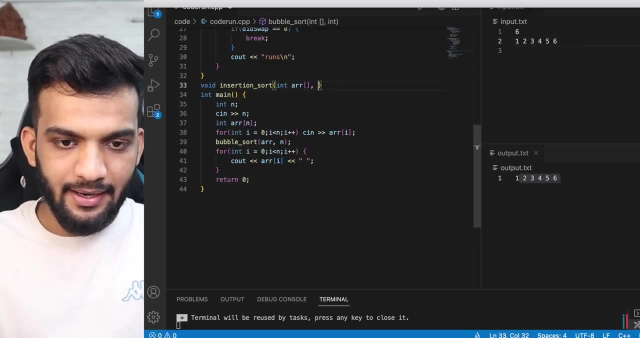 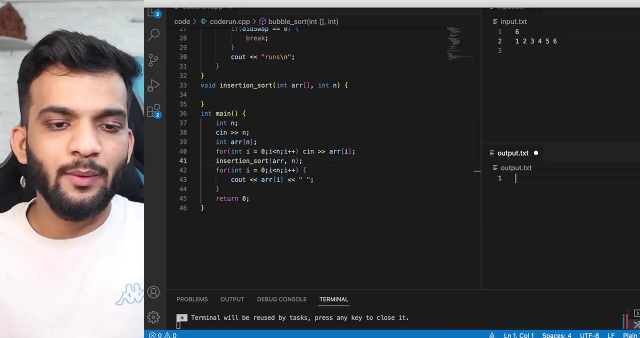 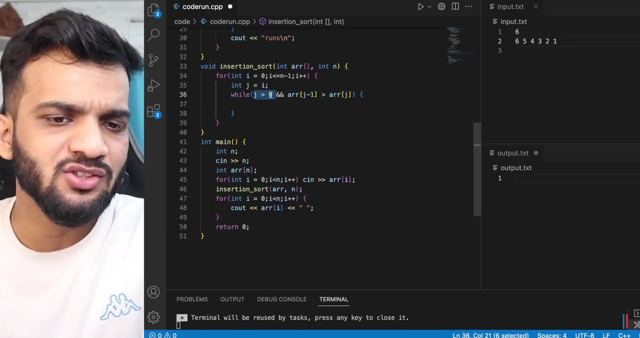 why it's now time to write insertion sort. right, so void, insertion sort. i'm going to write insertion sort, int array and int n, as usual. we can just do this as insertion, okay, and i'll quickly write the pseudocode. until here, you know the pseudocode. why j greater than zero? why not greater than equal? to imagine, 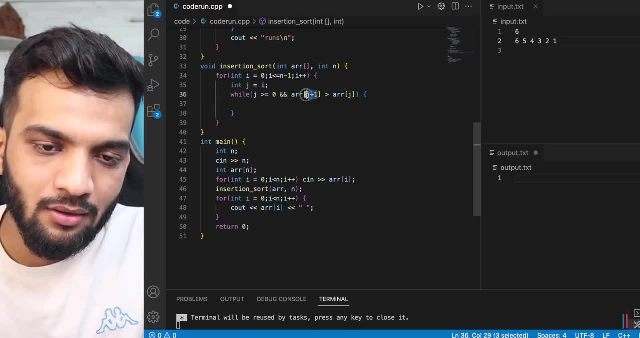 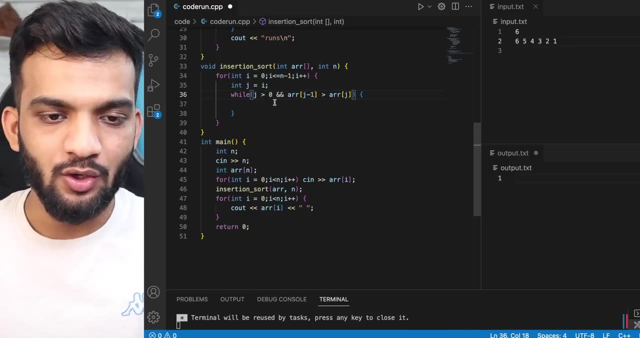 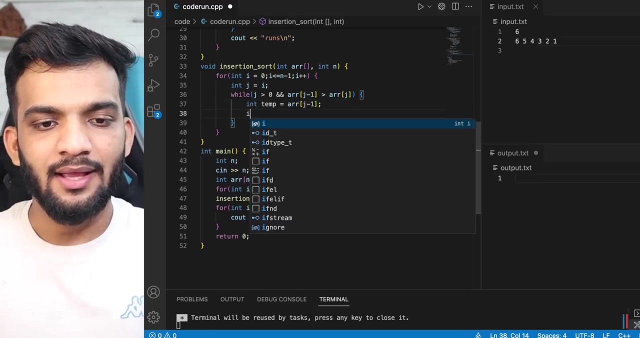 if j goes equal to zero, this j minus one- like when j is zero j minus one- will be minus one runtime. that's all right. so over here you can go ahead and swap it int temporary equal to array of j minus one, and that array of j minus one is array. 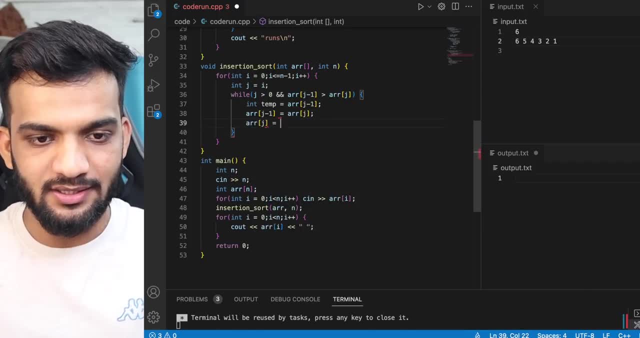 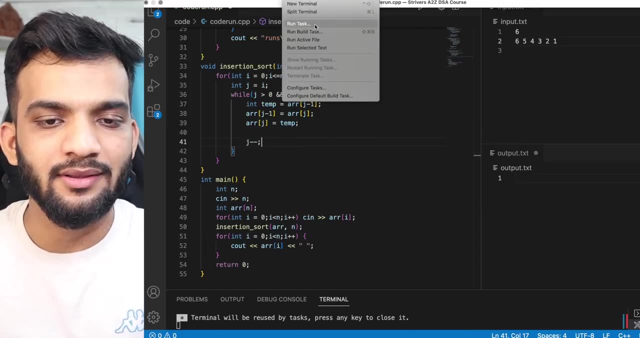 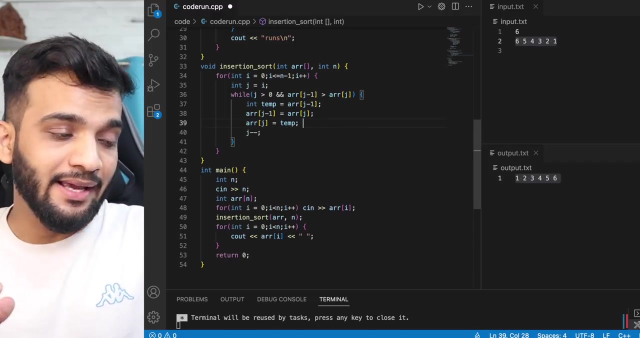 of j and then you can go ahead and say: array of j is equal to temporary and once you have swapped, let's go more left. so j minus minus. now let's go ahead and quickly run this and see if this is sorting this particular thing. yeah, it is sorting done, simple if we analyze the time complexity. 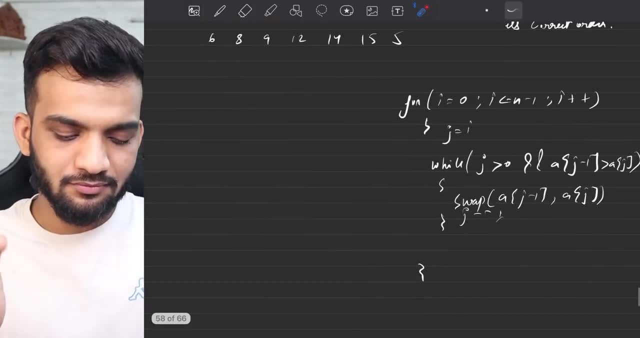 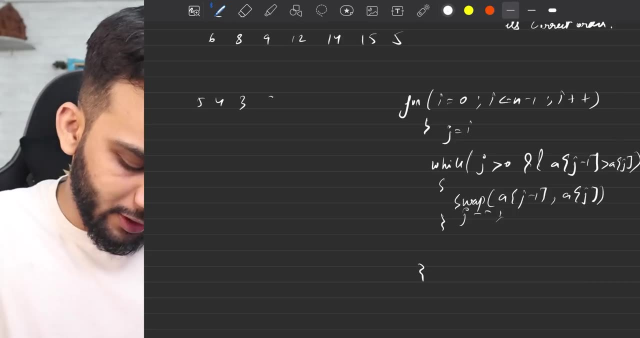 what will be the time complexity. imagine for a reversed array like something like five, four, three, two, one. what's happening for the first time, five, no swaps. next time it comes to four and does a swap, it's like four, five. next time it comes to three, does a complete like three goes here, then three goes here, next time it. so it's like: 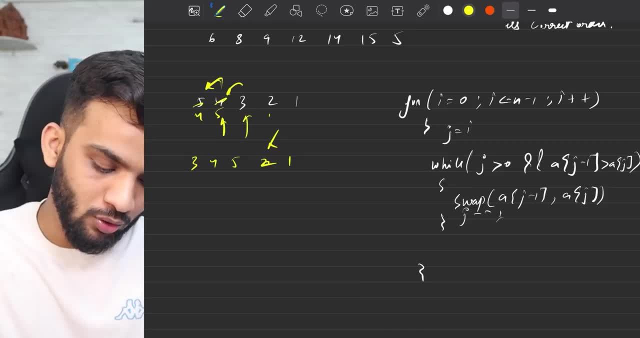 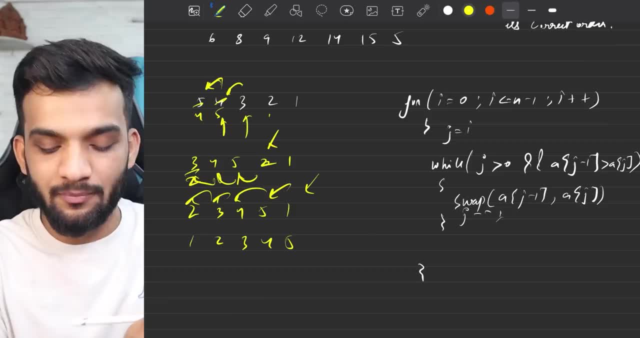 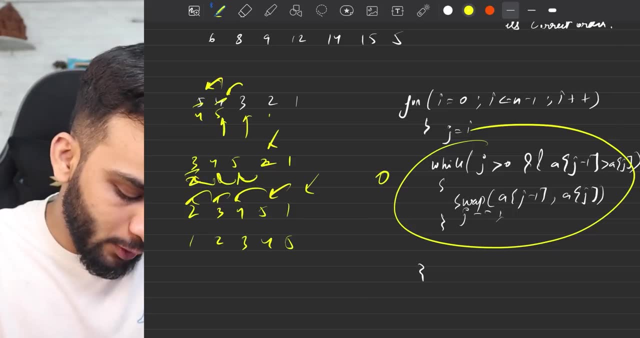 kind of going extreme left to the to the extreme left. this loop for the first time ran for zero times when it was at five, when it was at five 5.. When it went to 4, it swapped 1 place. Next. when it was at 3, it swapped 2 places, Next when. 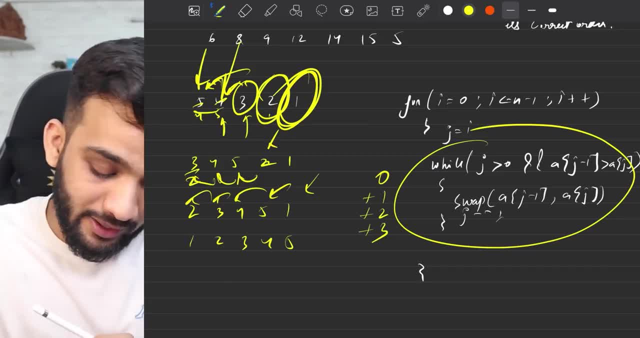 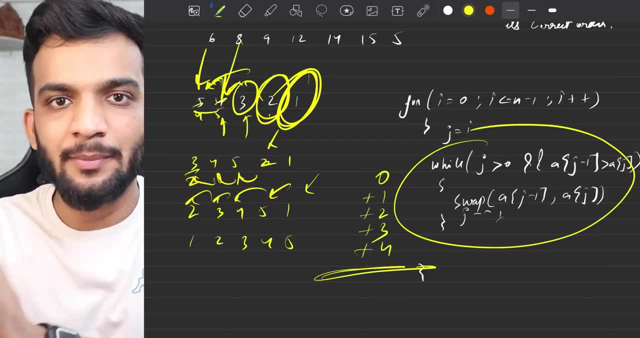 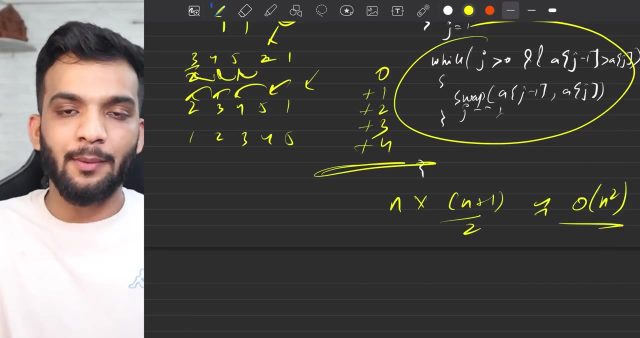 it was at 2, it swapped 3 places. Next, when it was at 1, it went left 4 places. It's kind of again going into the similar direction of summation of natural numbers, which is n cross n plus 1 by 2 makes it near about the time. complexity of n square. if you remember the 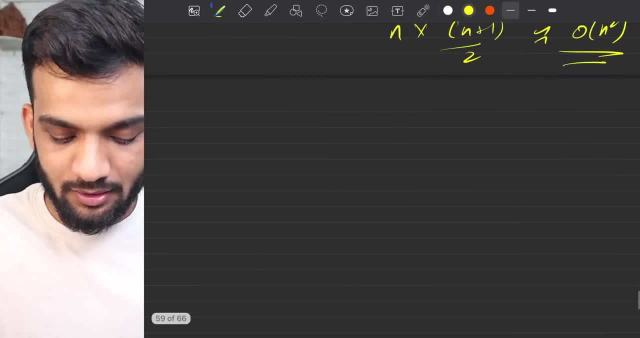 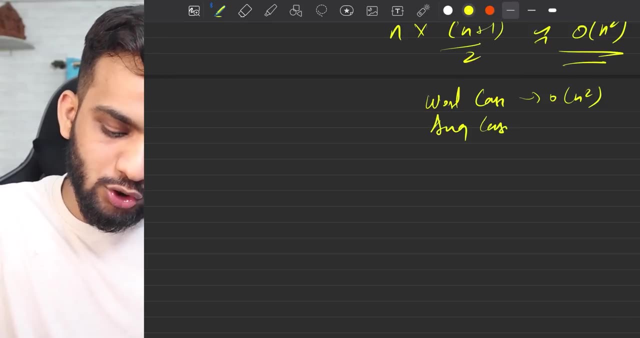 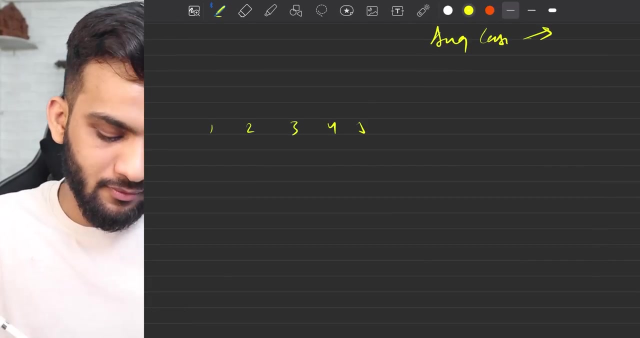 time complexity class. So I can say the kind of worst case is n square. The average case is also n square. But what about the best case? Imagine I give you something like 1, 2,, 3,, 4, 5.. 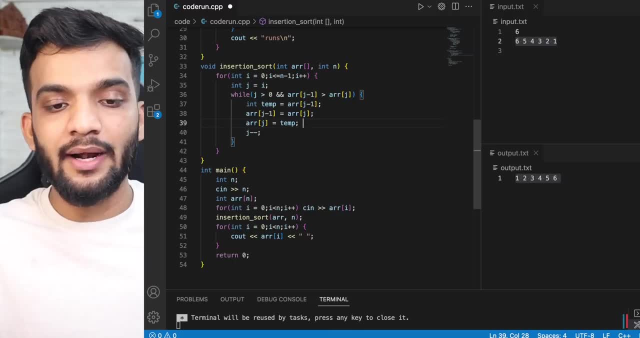 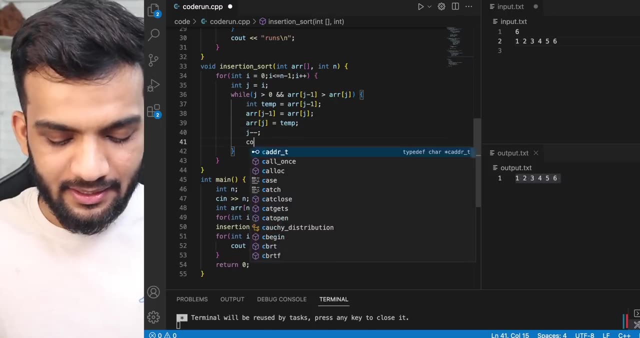 1,, 2,, 3,, 4,, 5.. And I go back to the code, And I go back to the code. So imagine I give you a completely sorted array And I go back to the code And let's see how many times. 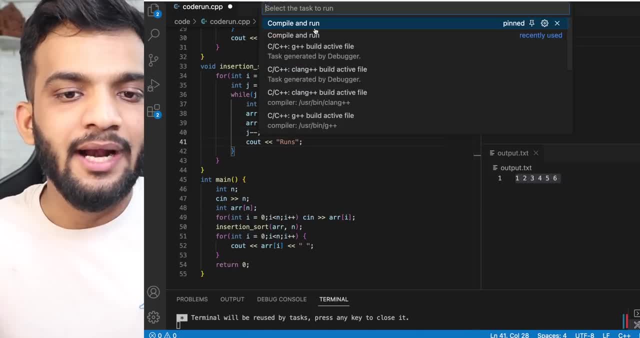 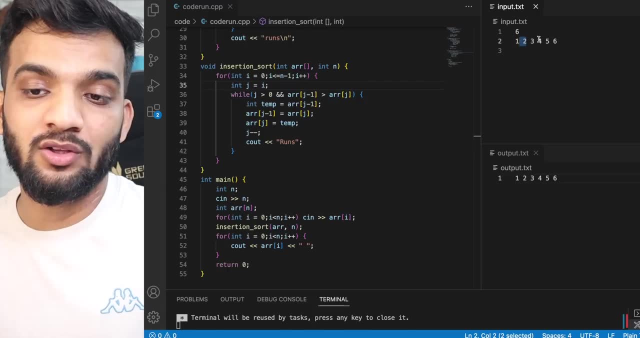 this loop runs. Go to the terminal and try to print it. This loop will not run a single time, Because for 1, there's no 1 on the left. For 2, there's no 1 on the left. 3 is already. 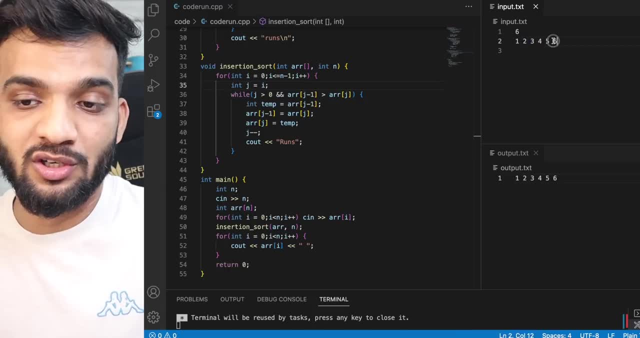 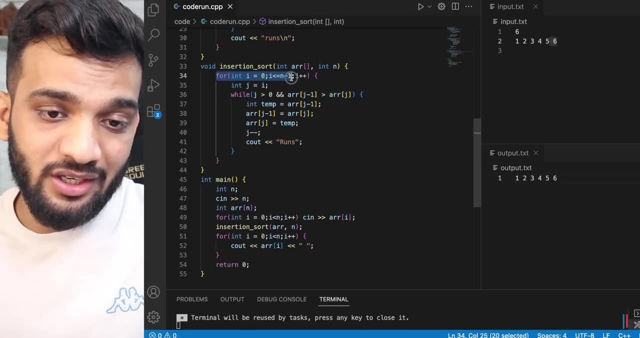 in its correct position. 4 is already in its correct position, 5 is already in its correct position, 6 is already in. So this putting them into the correct position never happens. So apparently only this loop runs for check. It's a B co-off. It's a B co-off n The best. 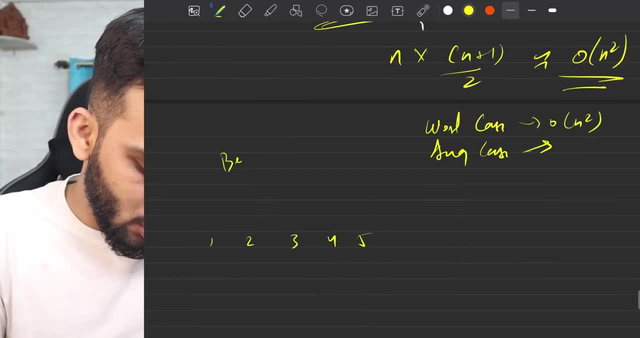 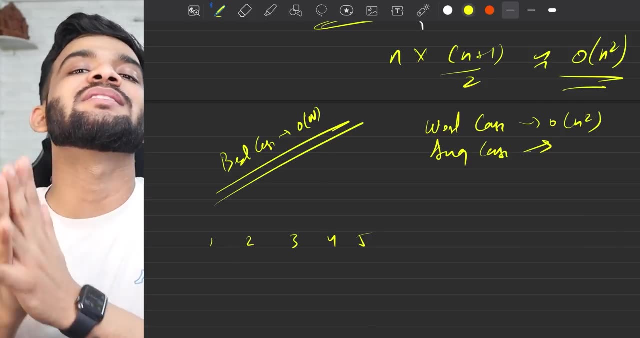 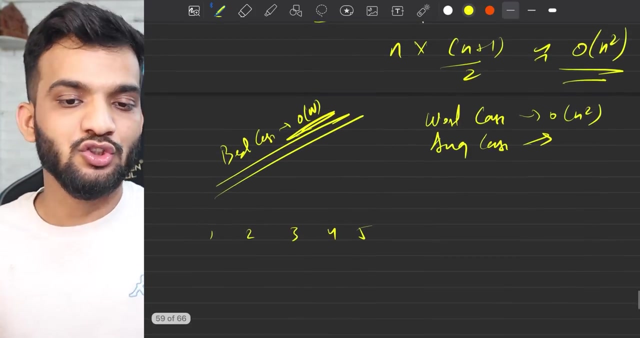 case for this is now n Nothing but B co-off n complexity, because there is no swaps that happen. Everyone is at its correct order, Just go to everyone. That is what the time is taken for in case of insertion sort. So with this I can tick mark insertion sort and it is completed. The 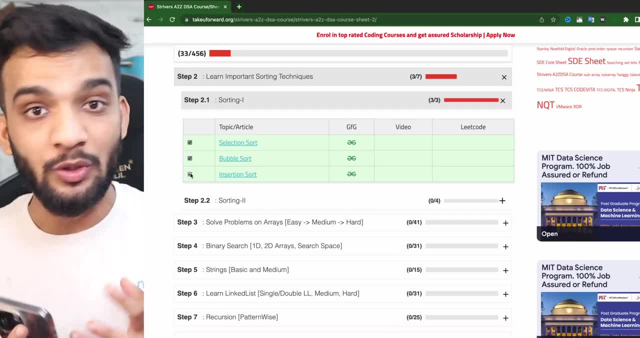 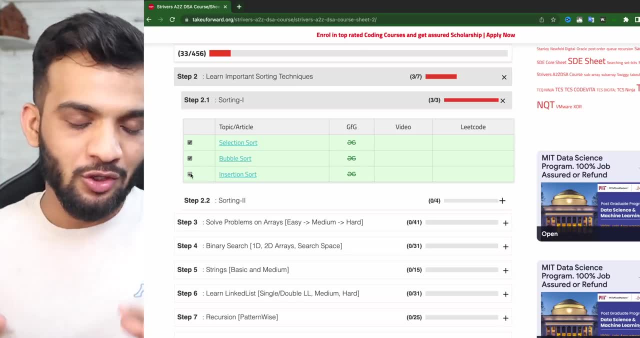 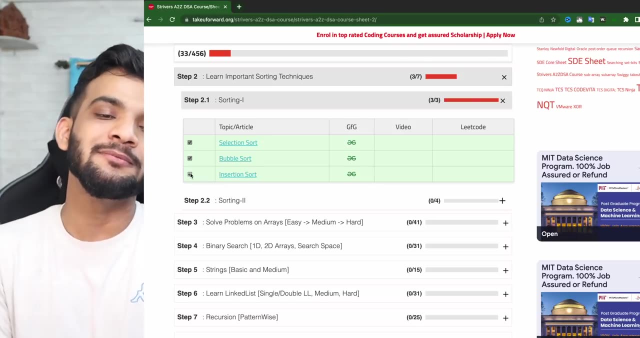 time is 529.. Yes, because I do take a lot of retakes while recording because I want it to be perfect, Like a lot of times I teach two or three times. So please, please, for this effort, if you understood everything, do consider hitting that like button and to follow our ritual. 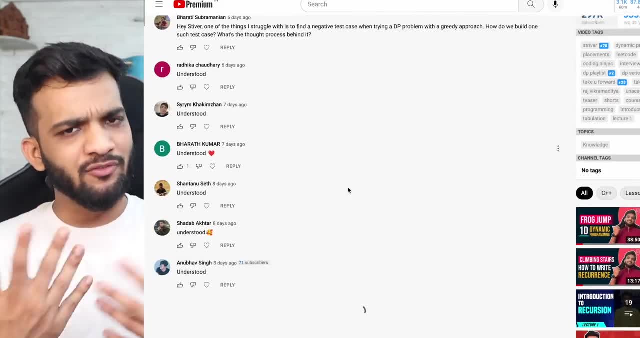 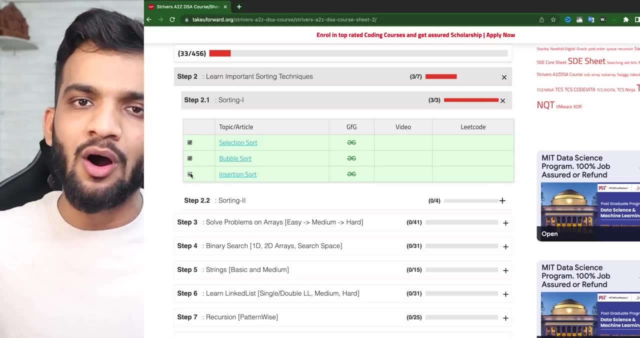 Please do comment. understood, if you understood everything. And if you have doubts, you can definitely put that into the comment section. I'll be replying to them. And if you're new to our channel, what are you waiting for? Hit that subscribe button and follow Stryver's A2Z DSA.